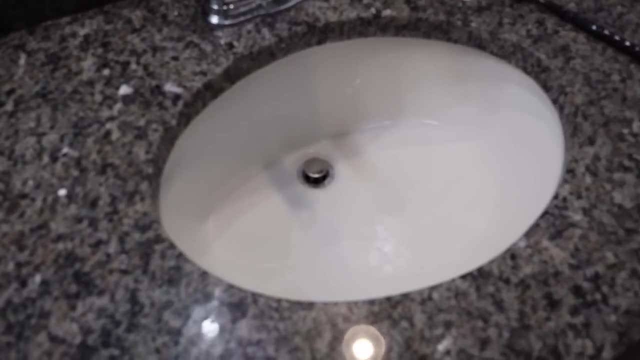 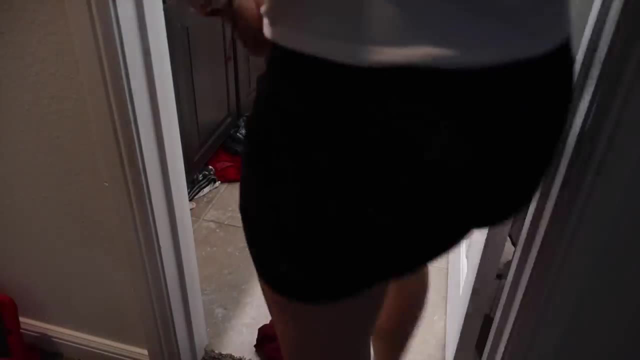 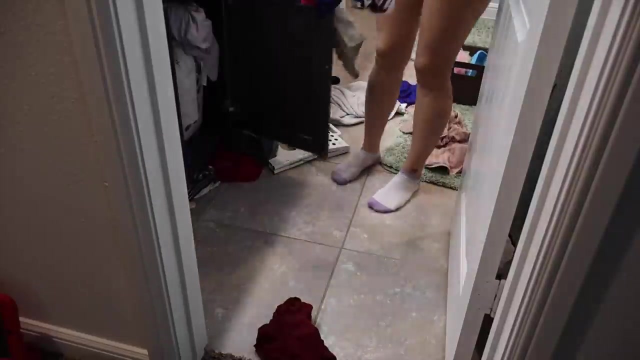 That are amazing, And I just want you to know that I truly appreciate you guys. being here and watching YouTube is my true passion, And I just love this community that we're building together. It really is a uplifting one. You guys leave me the best comments. overall, It really is a positive. 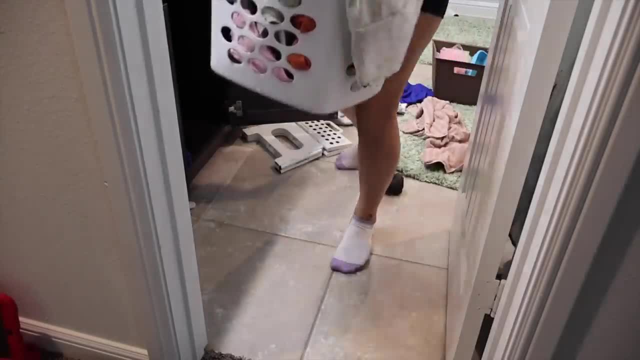 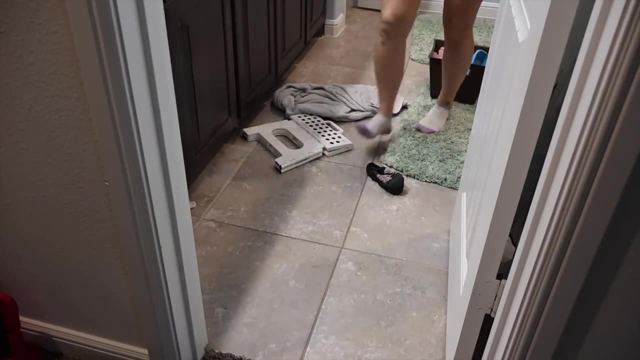 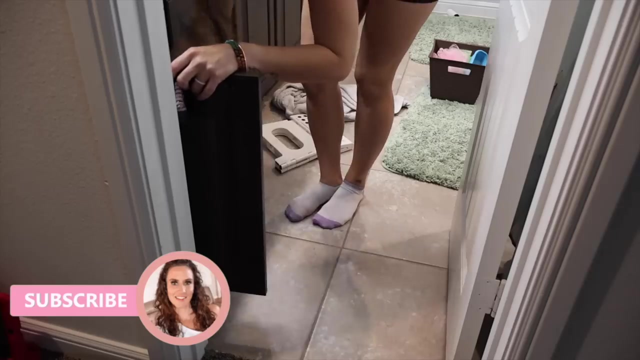 and uplifting environment And I enjoy getting on here and reading your comments. So if you are a fan of YouTube, I encourage you to leave me a comment down below just telling me a little bit about yourself. I love chatting. It is my favorite thing about YouTube And I hope y'all know that. 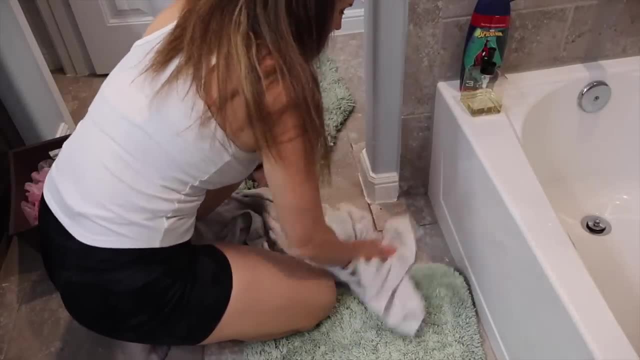 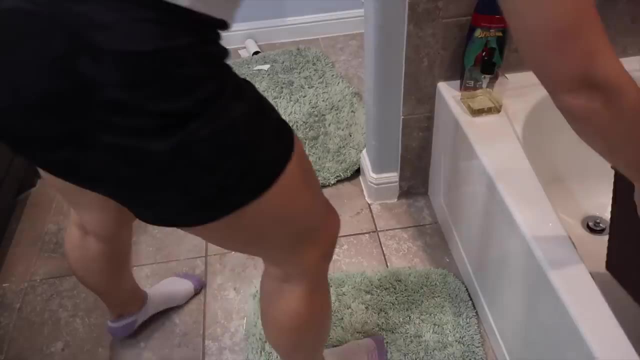 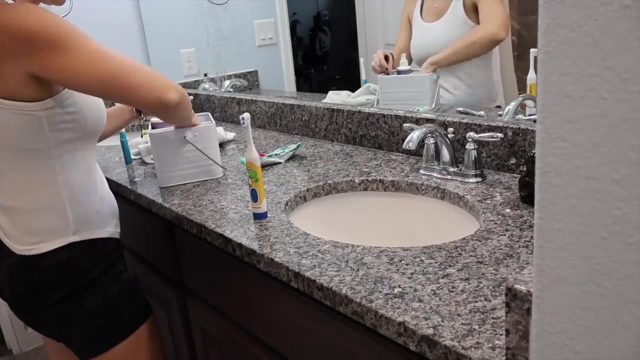 your comments do not go unread, And I will be forever grateful for this platform and for all of my amazing subscribers. I never thought in a million years that this is what I would be doing If you would have asked me five, 10 years ago. 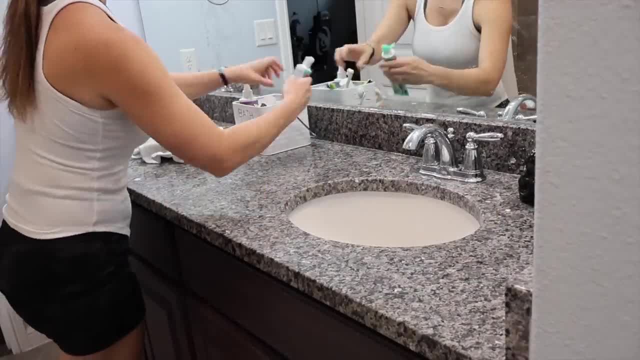 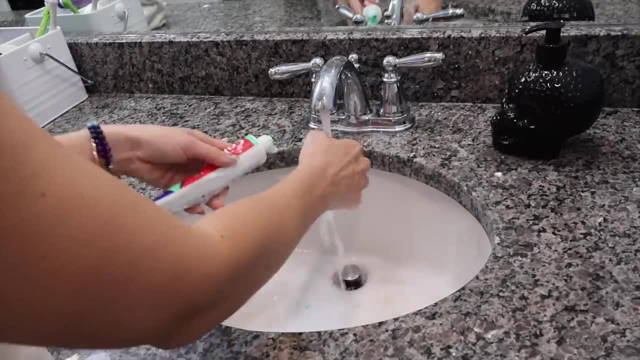 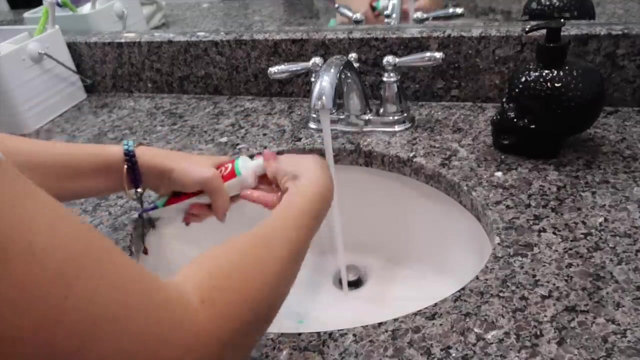 I mean, first of all, I didn't even really know about YouTube, Let's be honest, but it's just crazy. It's crazy. Now there is this platform where we can come together from all around the world and encourage each other. So this is just so special And I hope you know I do not take 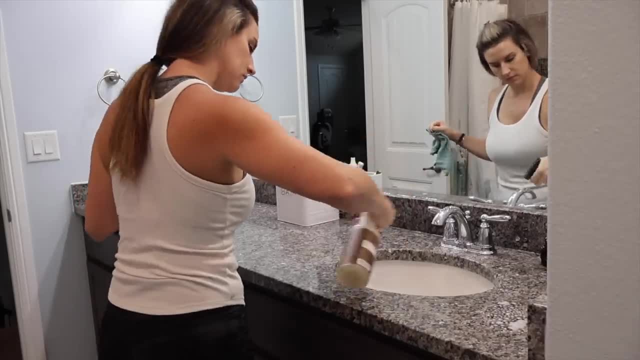 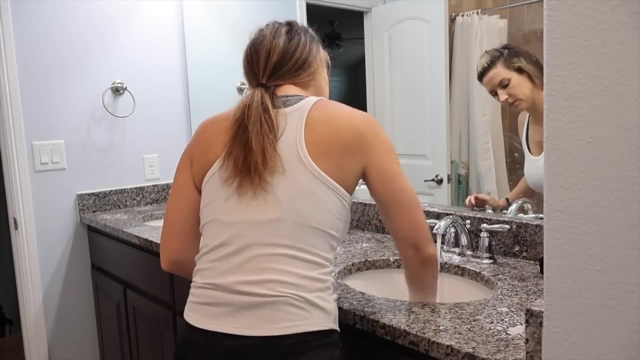 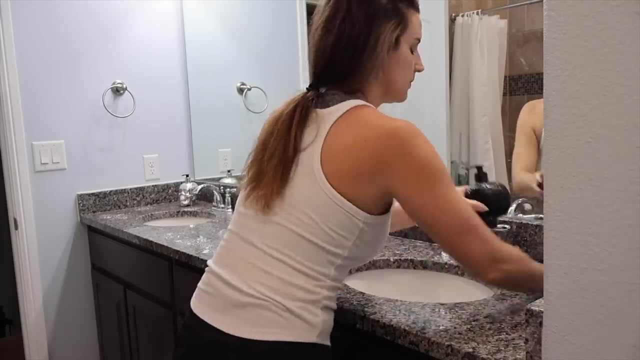 it for granted for one minute. but now let's get into all of this cleaning. As you can tell, we're starting off upstairs, in the kid's bathroom, And it was definitely destroyed. So Ethan, my youngest. he is now four years old. He typically 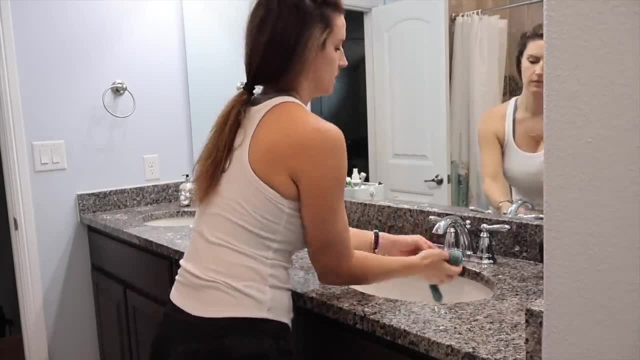 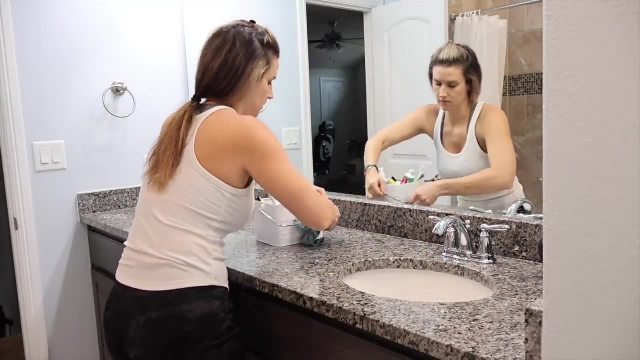 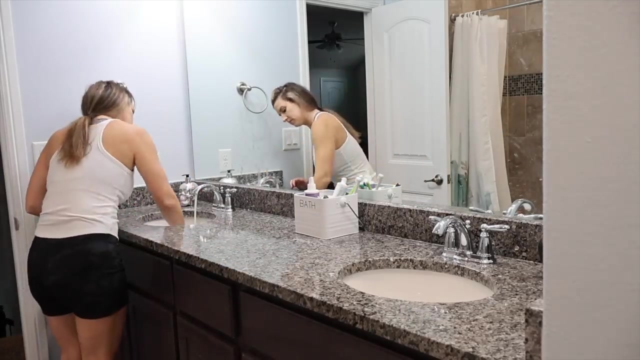 brushes his teeth using a step stool. Well, the night before he couldn't find the step stool, So he decided to try to jump up and spit the toothpaste into the sink And clearly he missed. it was all over the mirror, It was everywhere, So I knew I needed to get in here and get that. 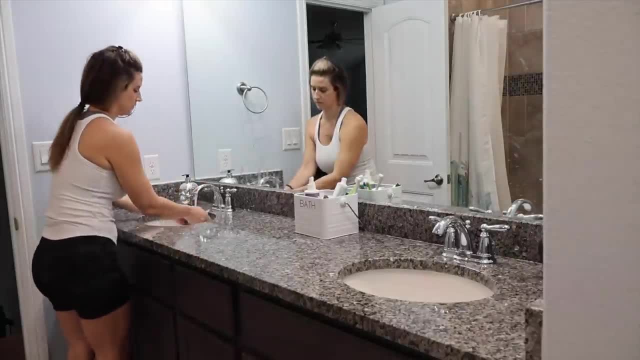 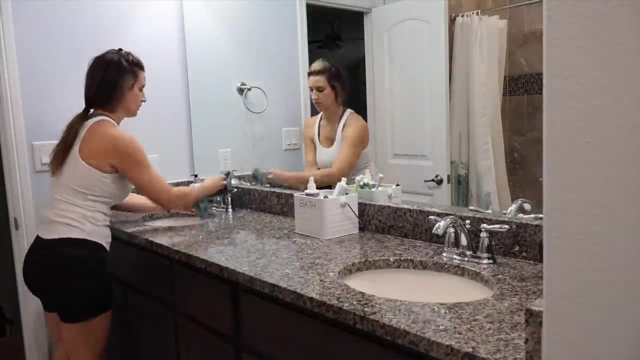 cleaned up, And you'll see here in a little bit. there was more of a mess than I even knew was in here, So we're going to do some deep cleaning. I'm also going to be sharing a hack with you guys that I'm really excited about. I just figured it. 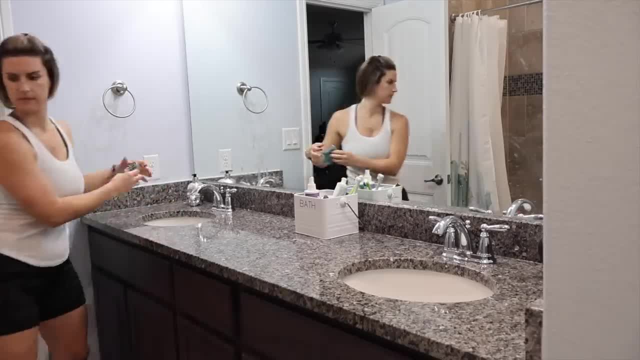 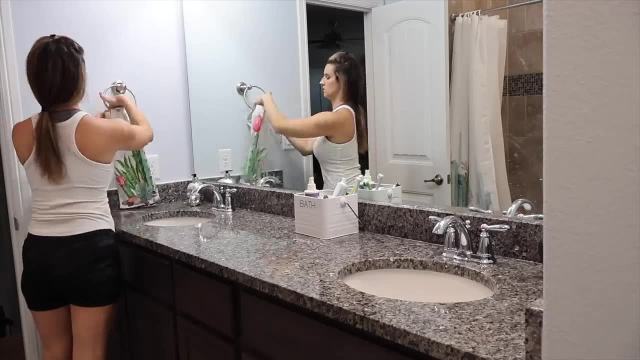 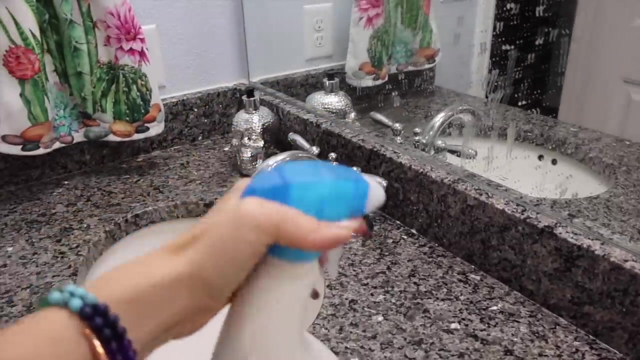 out and I am excited to use it now And I think y'all are going to love it. It's going to save you some money, especially if this is a product that you use often, So make sure you stay tuned. I will be sharing that with you guys in just a moment, But as I was cleaning this mirror, 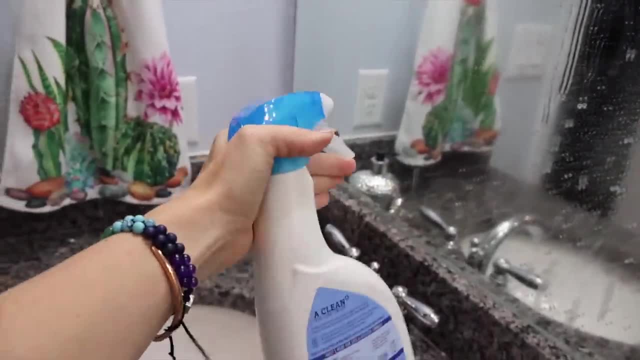 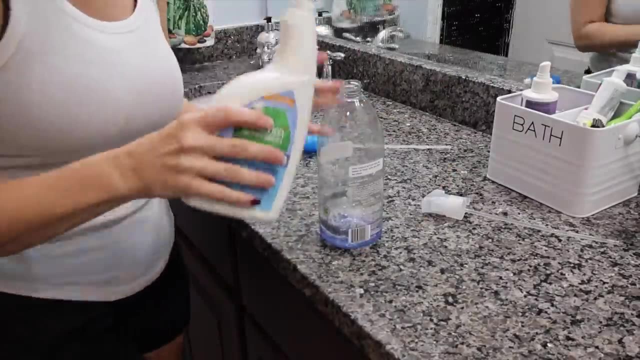 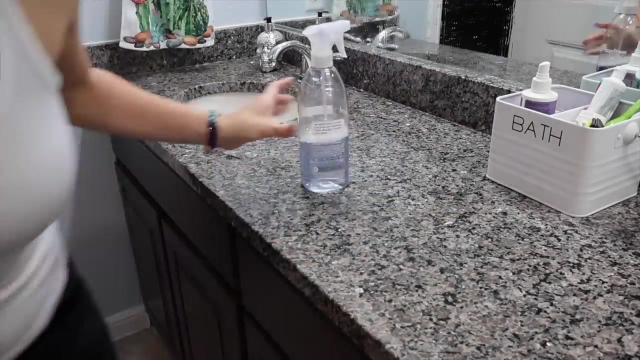 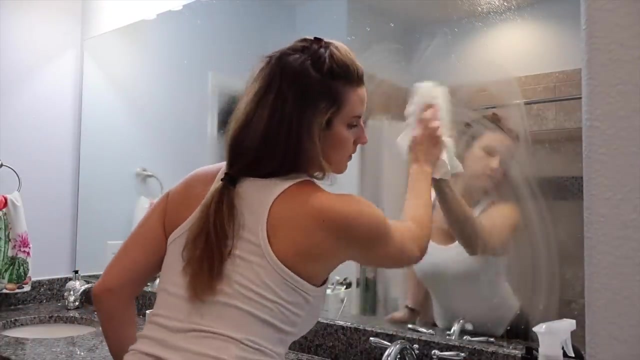 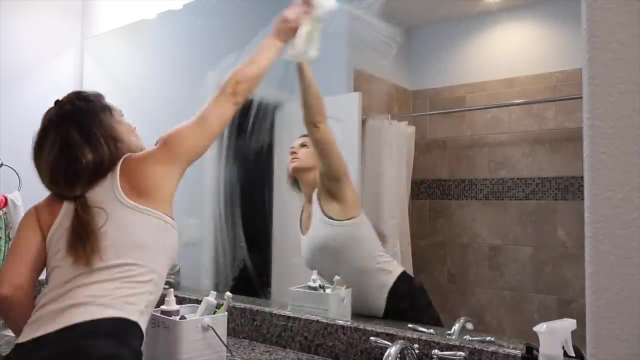 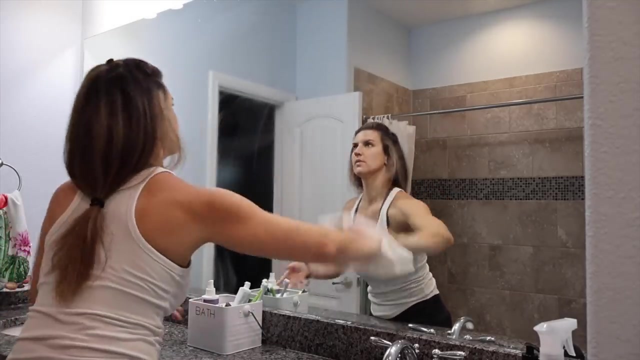 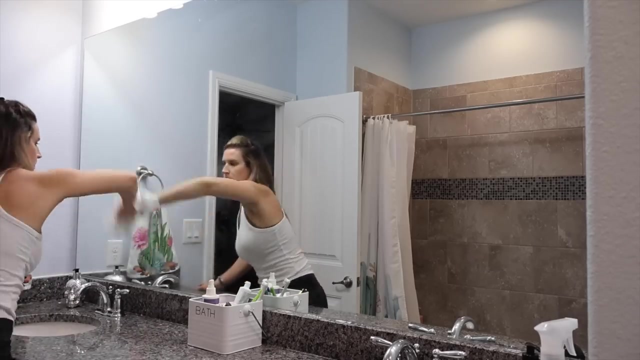 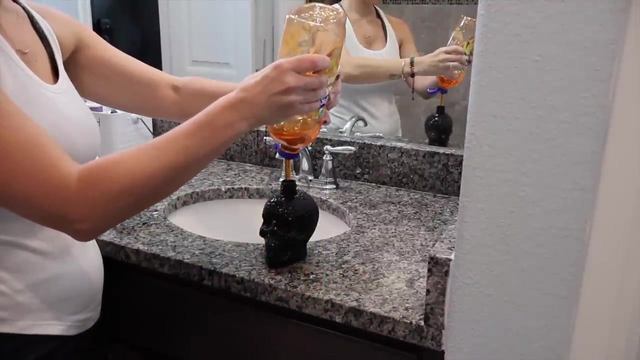 my sprayer broke on me, but thankfully I had an almost empty bottle of method. So I went ahead and just dumped my seventh generation into my method bottle. That way nothing went to waste. I also needed to refill the kids little soap dispensers. They go through so much soap. 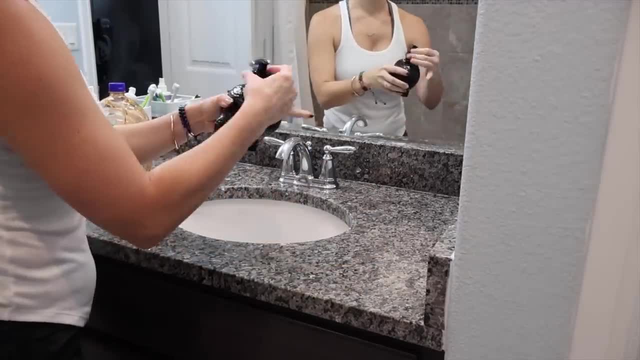 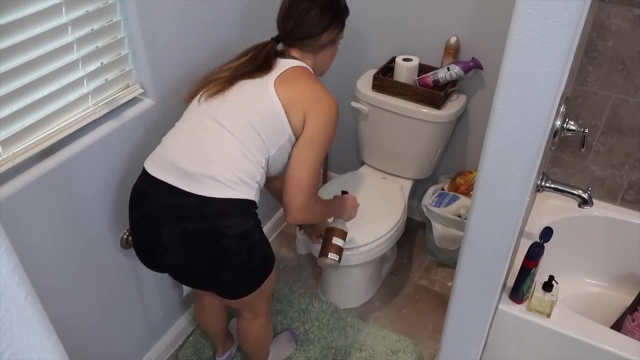 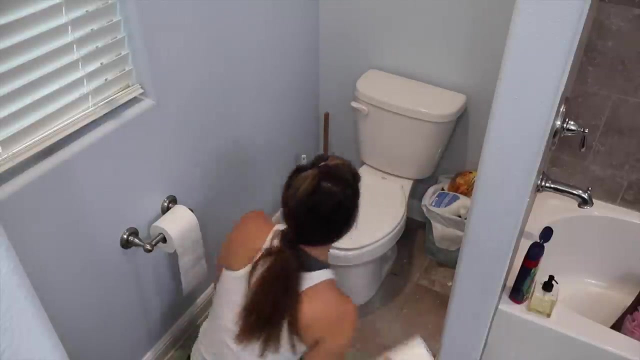 especially my oldest Aubrey. She wears contacts So she's constantly washing her hands, You know, before she puts her contacts in and after and all of that. So I like to try to stay stocked up on the hand soap And we've currently been using the pumpkin spice scented one. It 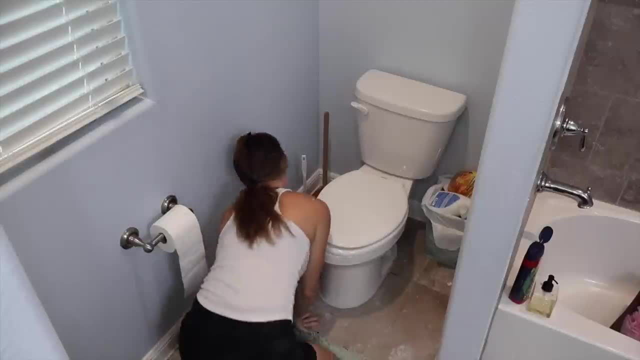 smells so good. But, like I said, today we're doing deeper cleaning upstairs And I like to really focus around the bottom of the toilet, especially when I'm doing deep cleaning, because, I mean, if you have boys in the house, I'm sure you know how it is. 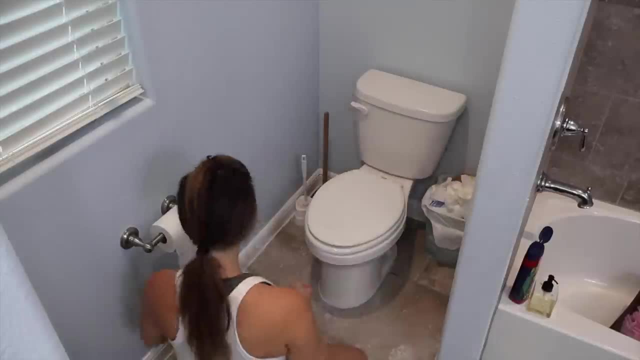 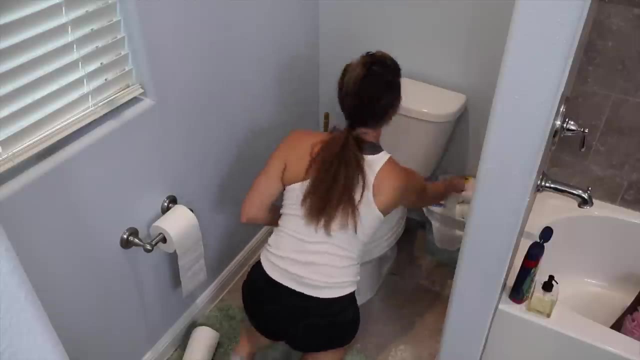 It gets so smelly And sometimes you just got to get in there and give it a really good deep cleaning. So I sprayed all around the bottom really well. I wiped up all of the dirt and everything else And then at the very end I am going to be steam mopping in here. 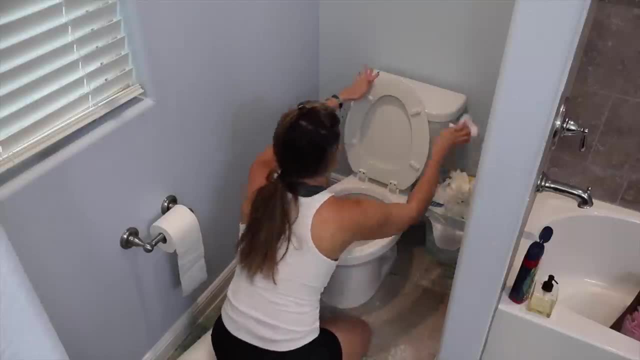 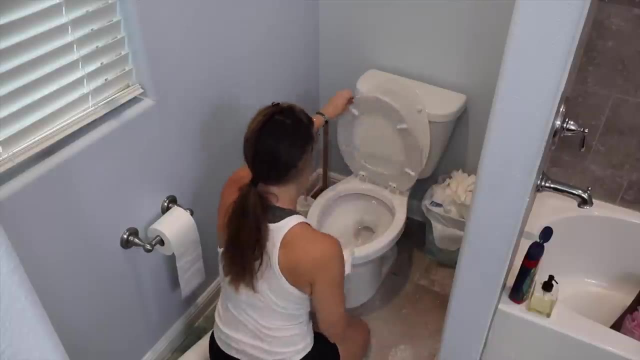 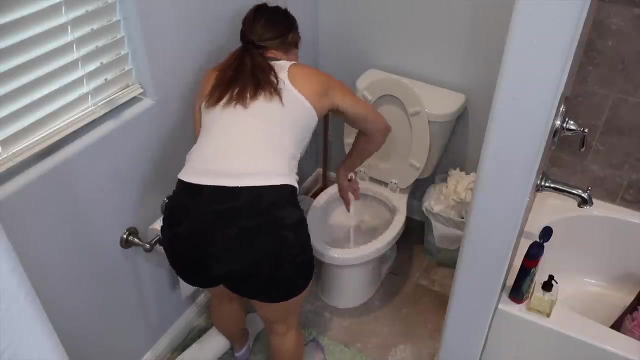 just to sanitize and make sure everything is germ free. I don't like anything I put in here and I will be able to clean it all up, But I'm going to be using a little bit more soap. This one is also one of my favorite scented. 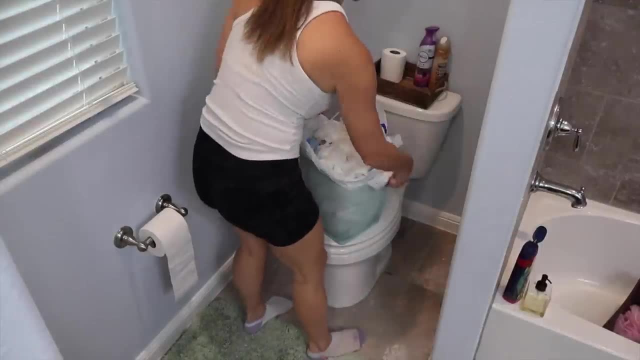 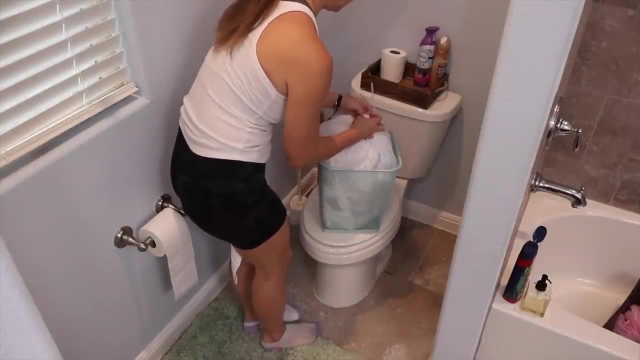 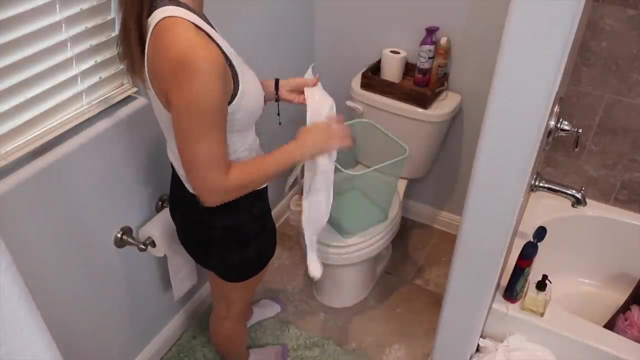 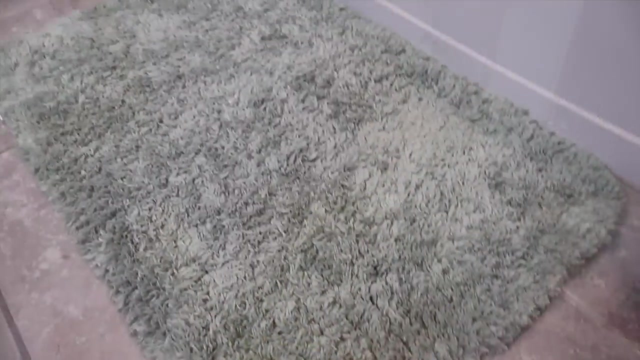 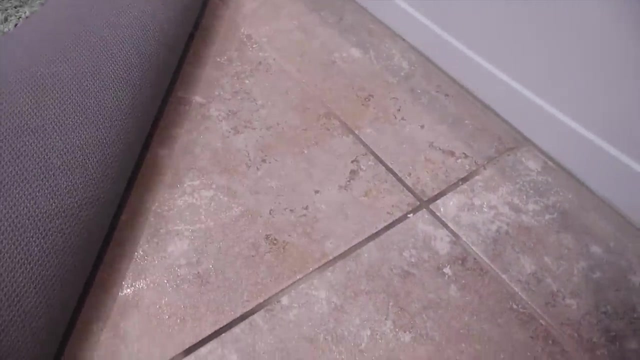 hand soaps. This one is called the Red durch Soap. Soap is organic. You can use it to make anything. And then what else? Soap Cleaning, Cleaning, Cleaning, Cleaning. If you guys watched my last video or two, I was talking about how the kids soak this rug. 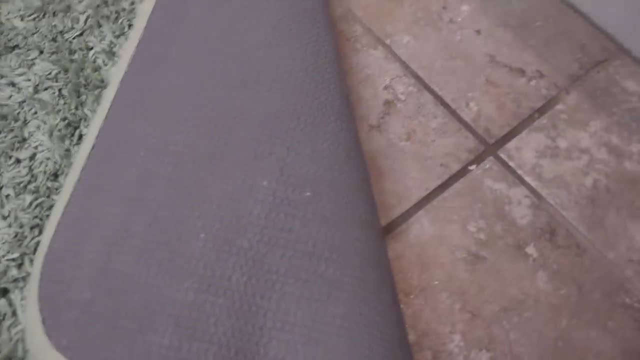 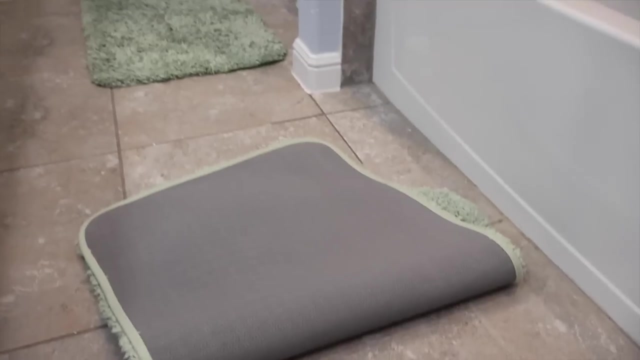 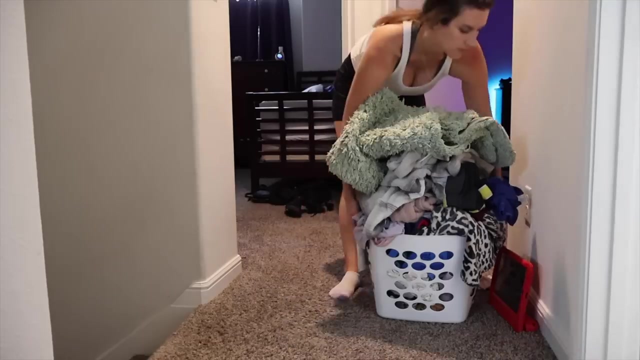 Did you hear that This is soaking wet? Oh, my goodness, I'm just going to go ahead and pull both rugs and wash them. It is so true when they say you never know what you're going to get when you have children. It is always something every day that surprises me. It surprises me, but also. 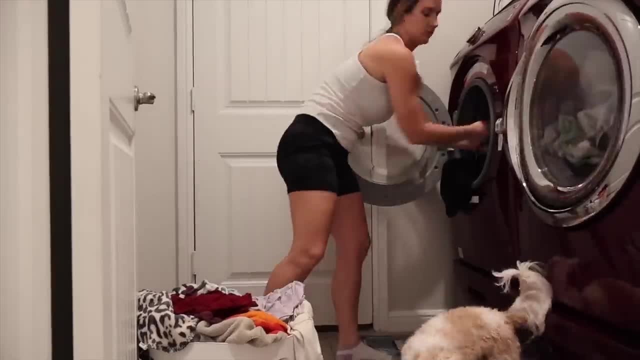 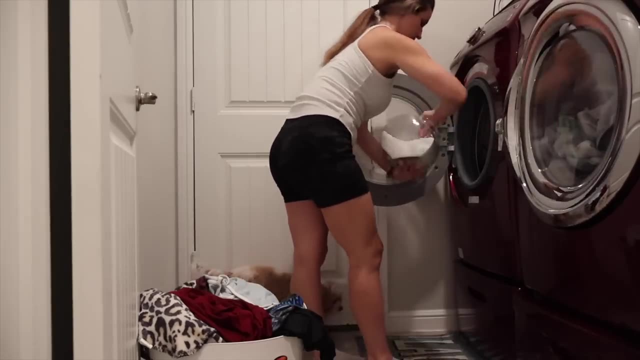 it doesn't surprise me- I'm sure you know what I mean if you're a parent- but I went ahead, brought all of the dirty clothes downstairs because it was overflowing. We're going to get some laundry going and then we're going to go upstairs and I'm going to share the hack with y'all. 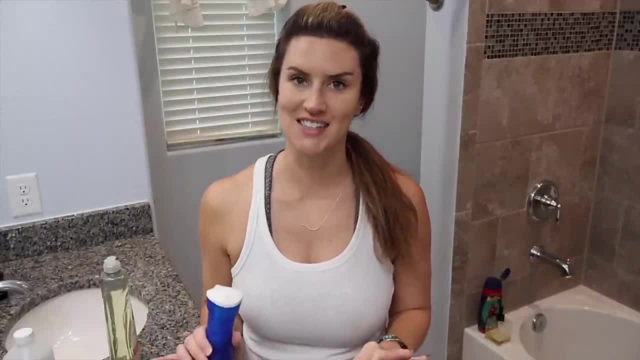 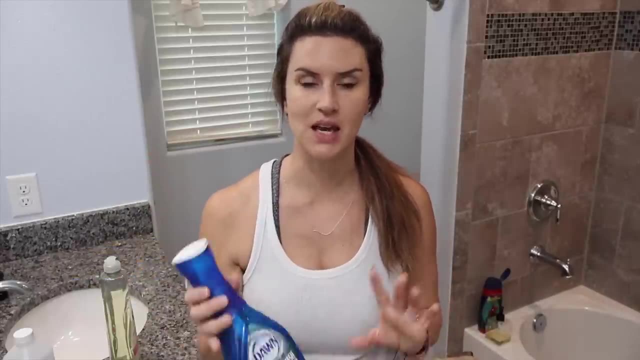 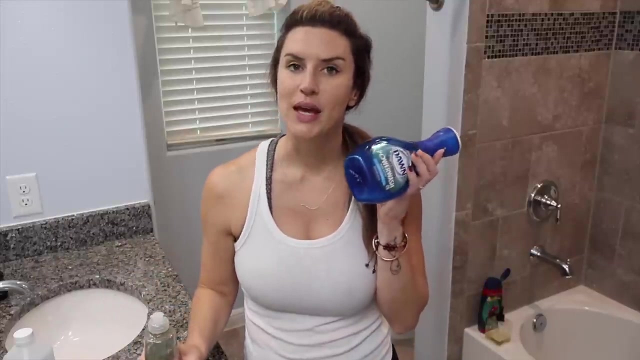 I thought we would try out this hack together. I have not tested this. We're going to find out today if it works. but you know how everyone is raving about the Dawn Power Wash. This stuff is amazing. I love it too. It works great. but I saw a YouTube short that said: you can make the 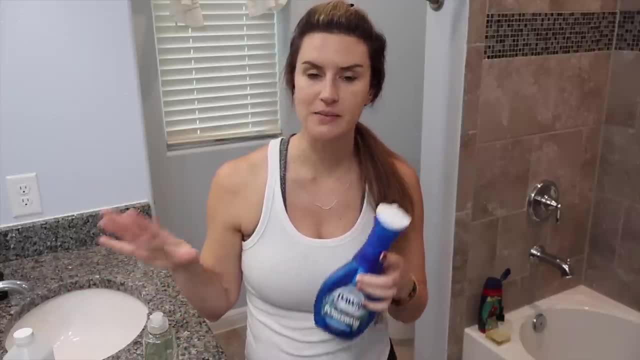 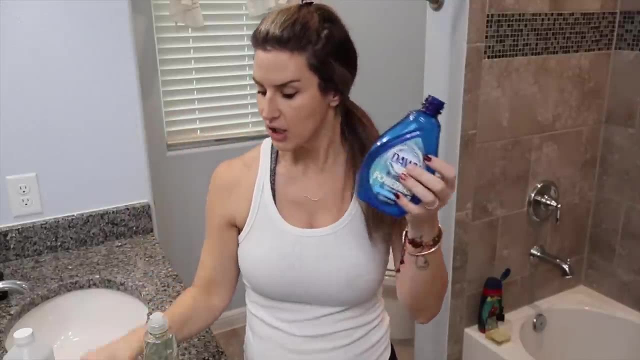 same thing using a few household items, and it works just the same. So I wanted to find out. So this is an empty one that I currently have. So all you need to do to recreate this, which, if you want to use Dawn dish soap, you can do that. I'm going to show you how to do that. 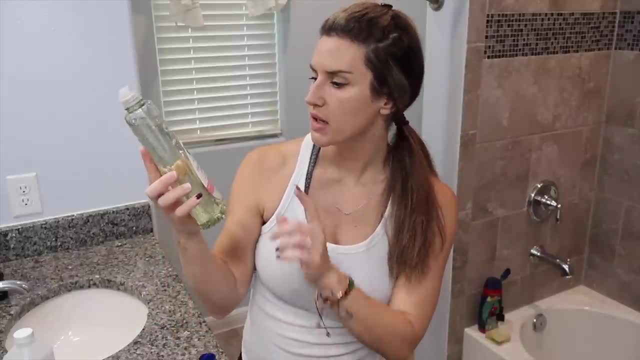 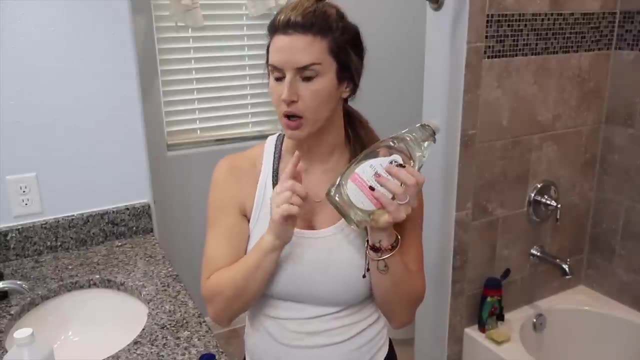 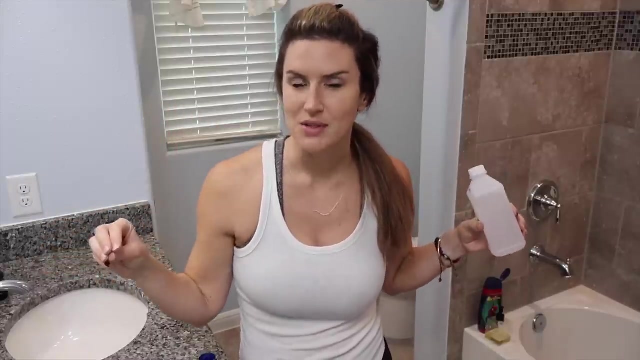 I don't have any on hand, so I'm going to be using just some Fielding Future. This is like all natural soap from HEB, So you're going to do like one third part soap, one third part rubbing alcohol and then the rest with water. I think that was around the measurements. I could not. 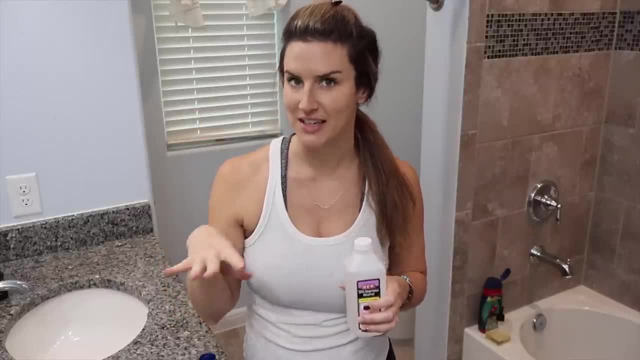 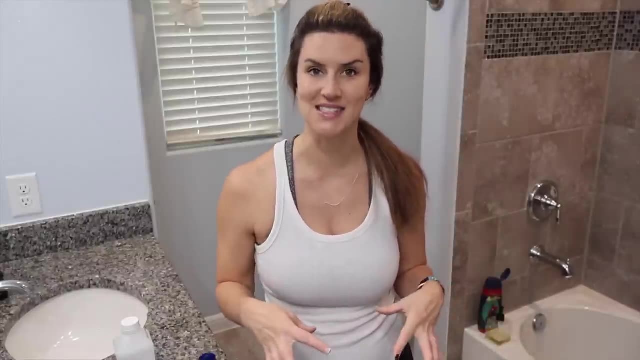 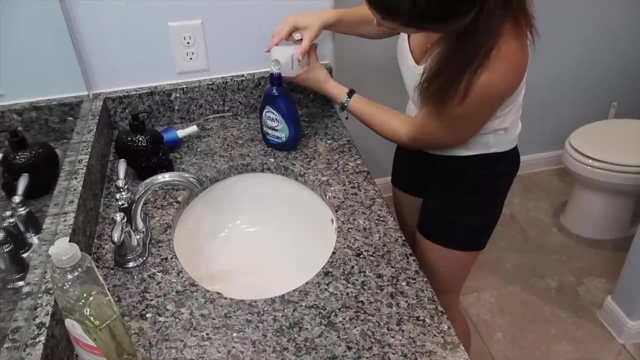 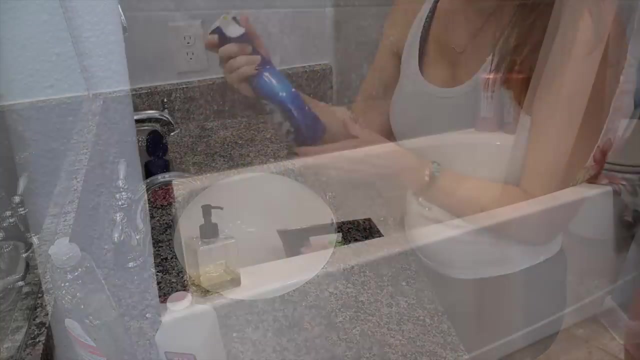 find the video again. I just remember it was these three ingredients. So let's make this and we're going to try it out in the shower and see if it comes out in that same consistency. Y'all have no idea how excited I was to try this out. I have been waiting until I could share it. 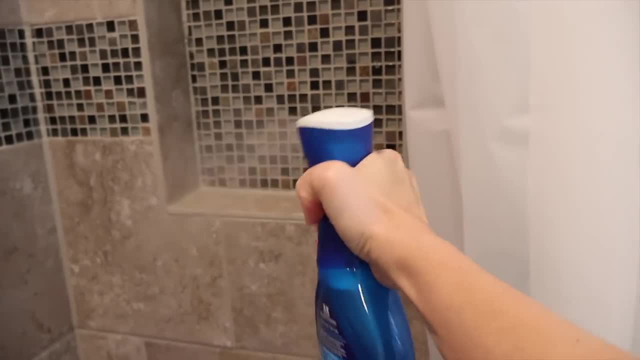 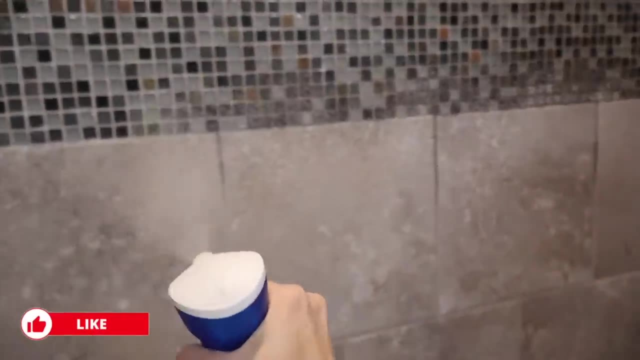 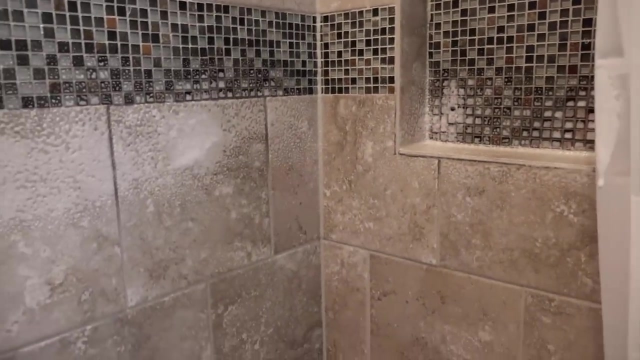 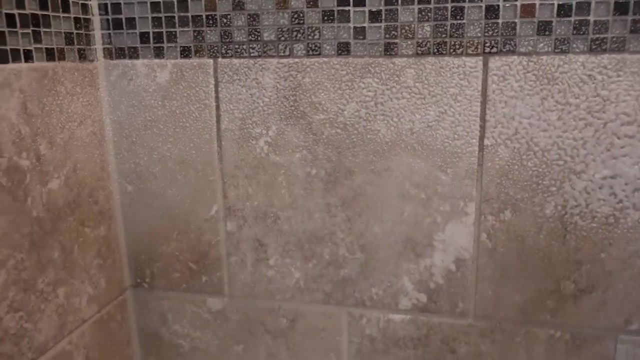 with you guys to do it. Oh my gosh, you guys, it's working. I did squirt it a lot just to make sure there wasn't, like, any old product left in there. But look at that, you guys. Oh my gosh, I am forever doing this now. 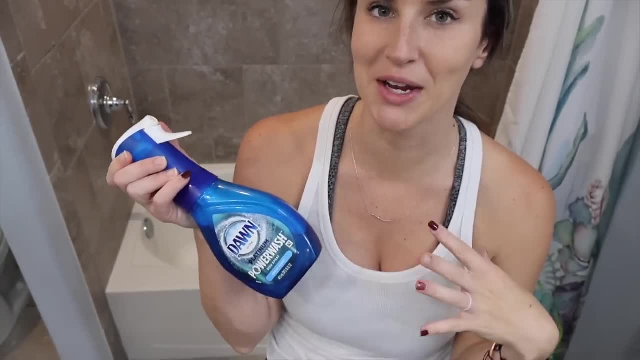 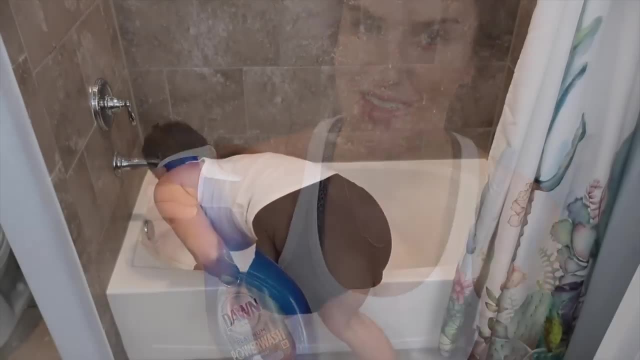 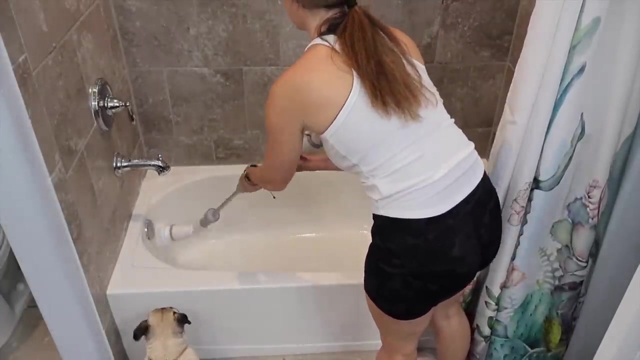 This stuff does smell really strong. It smells like hairspray. So maybe a little less alcohol next time or maybe some essential oils. But overall, you guys, this is a 10 out of 10.. Definitely try it out If you already have a Dawn Power Wash bottle lying around, and it's almost. 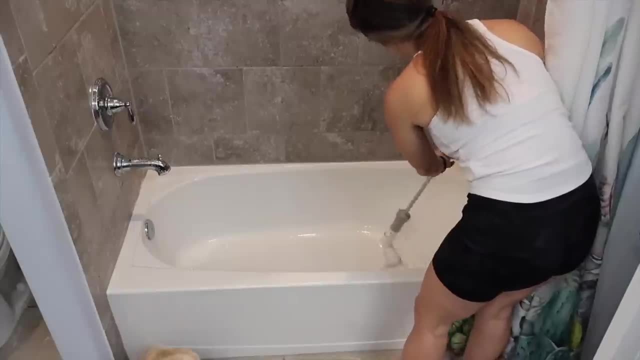 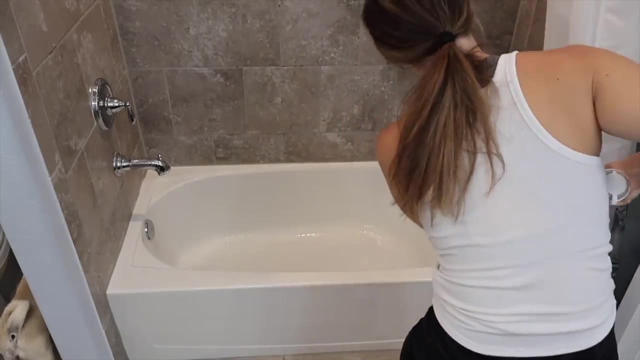 empty. give this a try. If you do, let me know down below what you think about it. My kids actually said they love this. I'm going to show you how to do it, So let's get started. This smell. it does remind me of hairspray, but also just kind of like an alcohol smell. 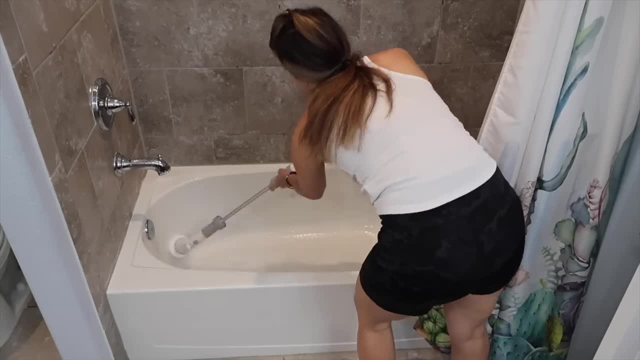 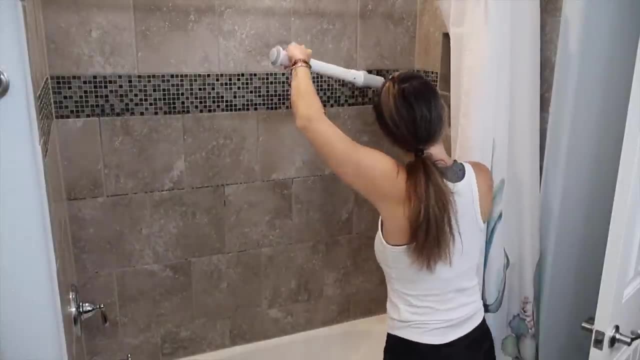 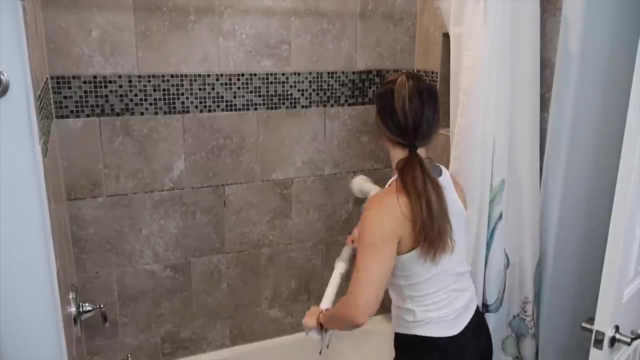 like a rubbing alcohol smell, So it doesn't smell bad at all. It's a really good scent. It still makes it smell clean And I just love that it's sprayed out in that same like foaming way. I've also been using it on my dishes And so far I feel like it works just as good at getting on. 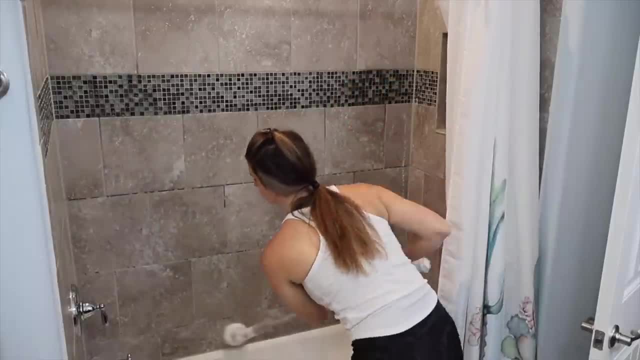 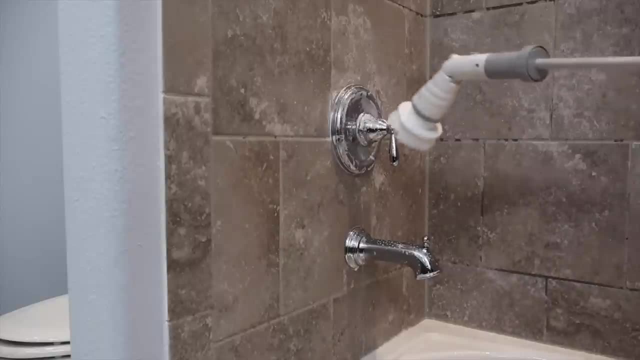 the stuck on grime and all of that. So let's get started. So I'm going to keep testing it out. I'll let you guys know if my opinion changes, But so far I feel like this is working just as good as the actual product. 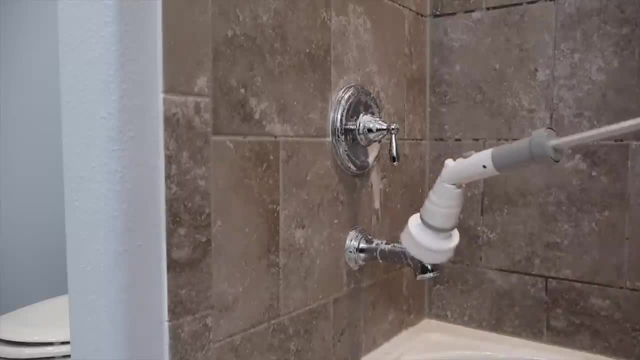 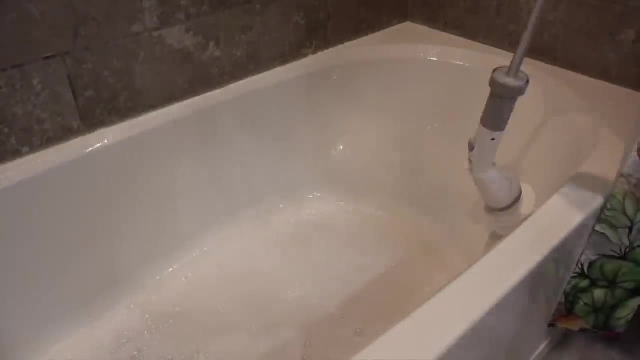 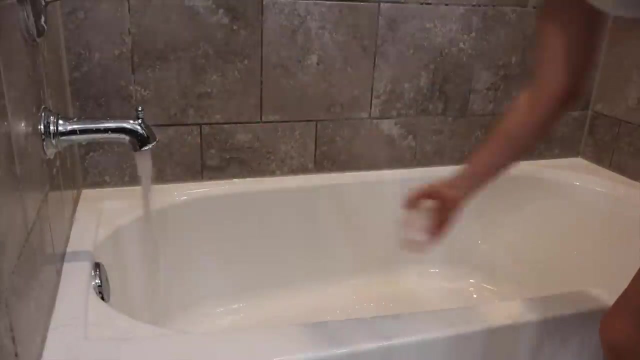 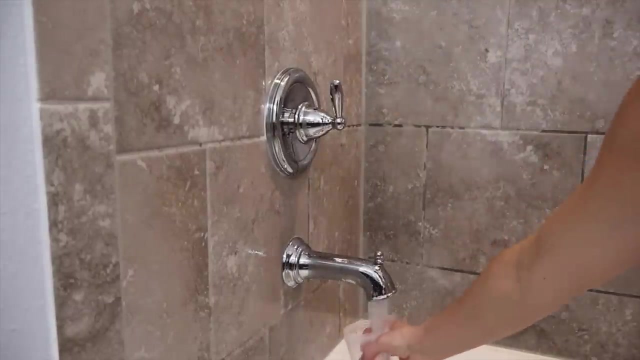 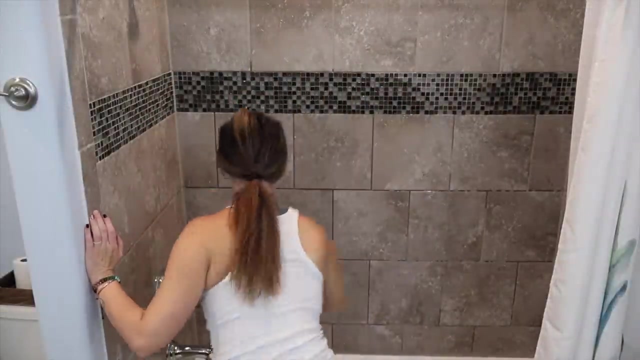 Y'all, this little shower scrubber has made all of the difference for me. I've mentioned this before that cleaning the bathtub, cleaning the shower, was something I always put off because I do not enjoy it. It is one of my least favorite things to do because it just seems so strenuous and tedious And I just never liked. 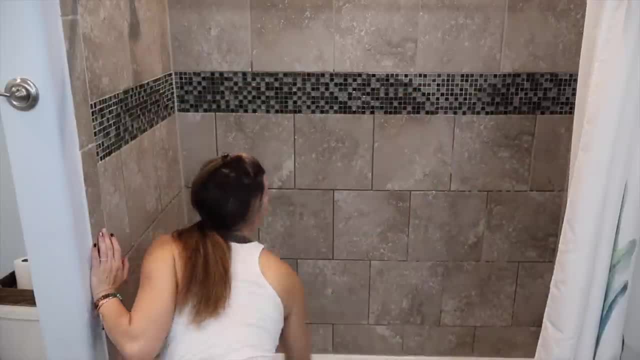 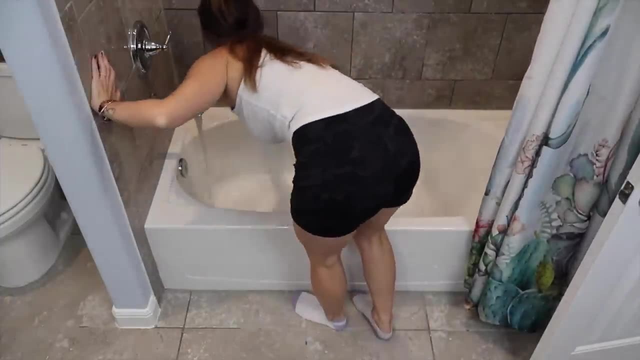 it. But now that I have my new extension electric scrubber, I actually look forward to cleaning the bathrooms now, Like I get so excited to use it. My back doesn't hurt, I don't have to lean over and struggle. So if 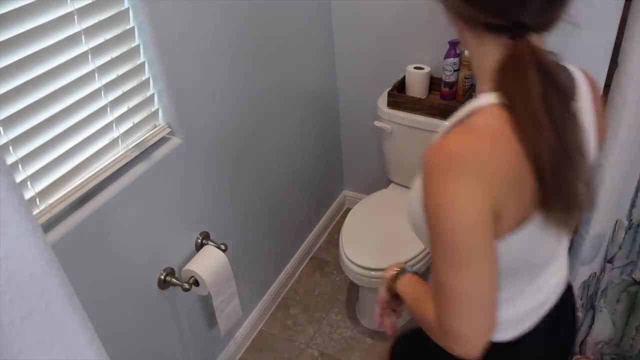 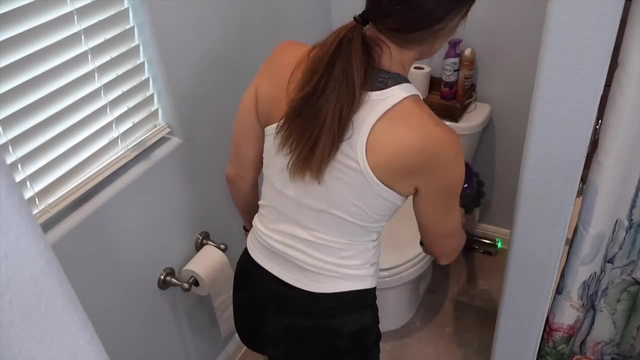 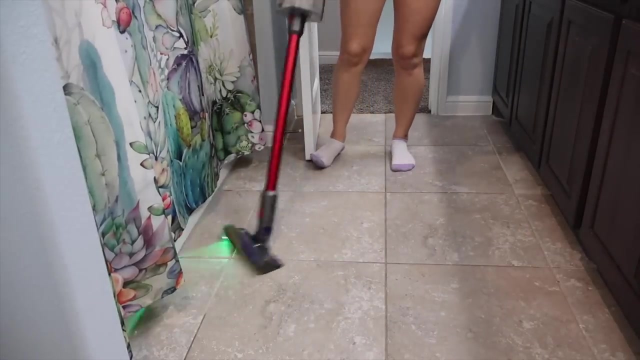 you guys have been thinking about getting one and you haven't. I definitely recommend it. Put it on your Christmas list or your birthday list or whatever. Just go out, treat yourself, Because I promise you it's game changing. I at first, when I saw it, I was like: Oh, I don't need that, That's. 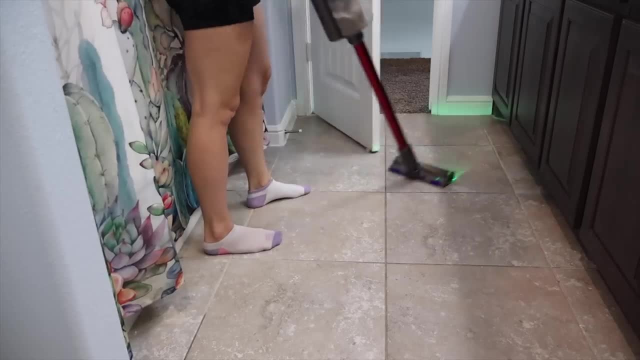 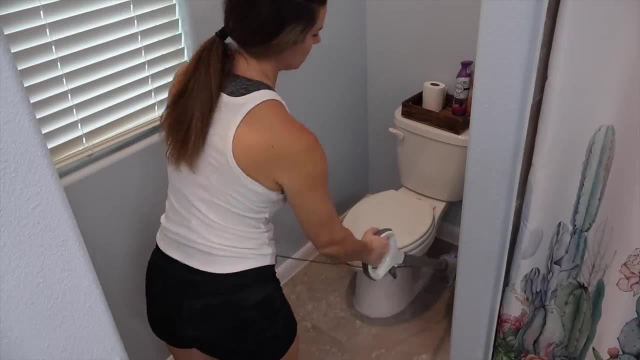 just a waste of money. No, no, no. you guys, I'm telling you. you know, I don't need that, I don't need it. It is so awesome to have It makes cleaning your shower and bath a million times. 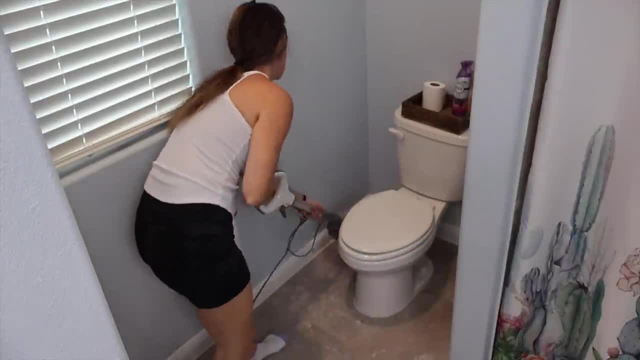 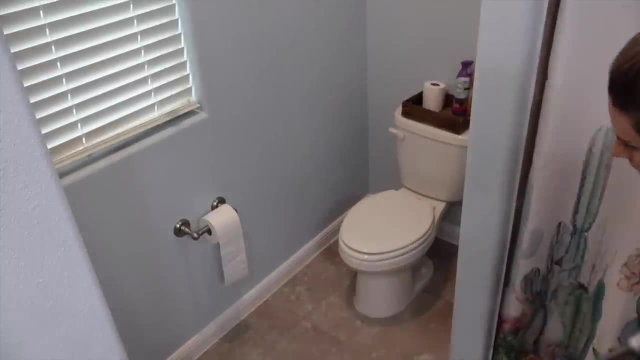 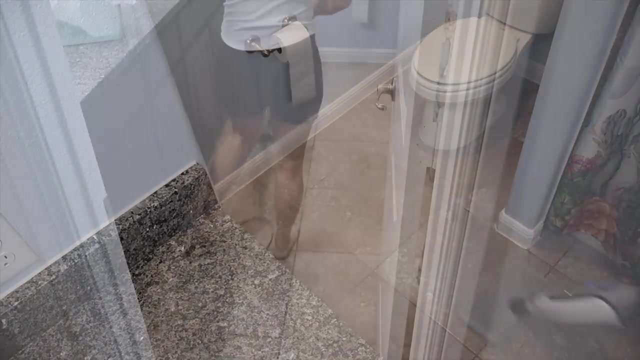 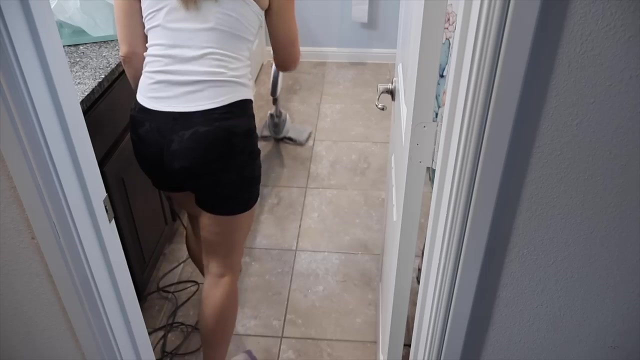 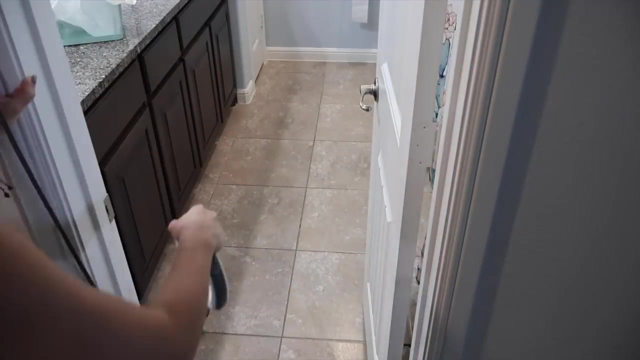 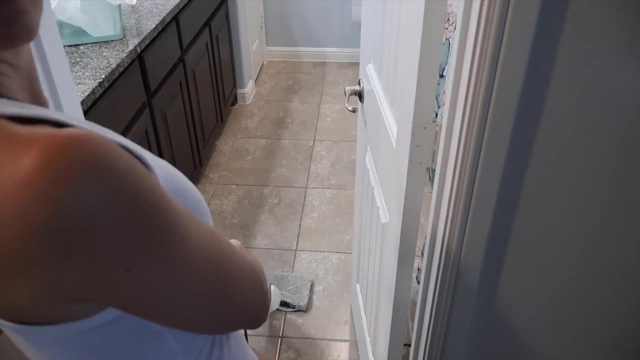 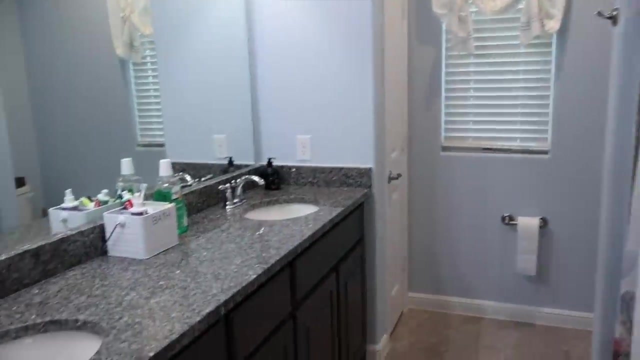 easier. Steam mopping is something I just love to do. I feel like it leaves the air feeling so clean And so fresh. I love it, And I just love knowing that the germs are killed and my floors are freshly cleaned and not sticky anymore. So once we finish up in here, we're going to head into Adrian's room, one of the 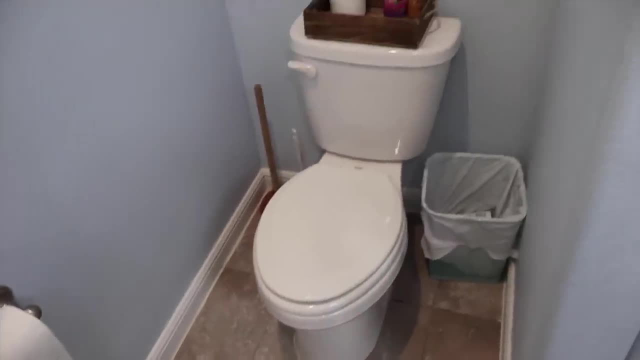 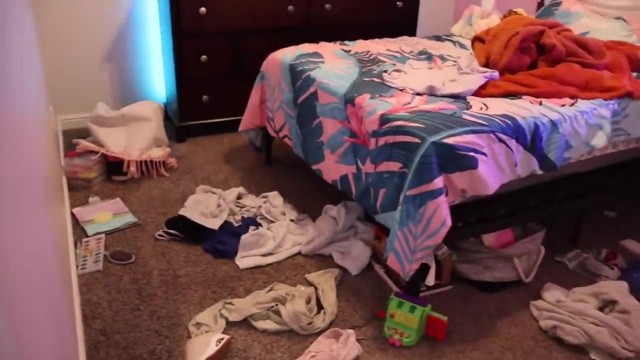 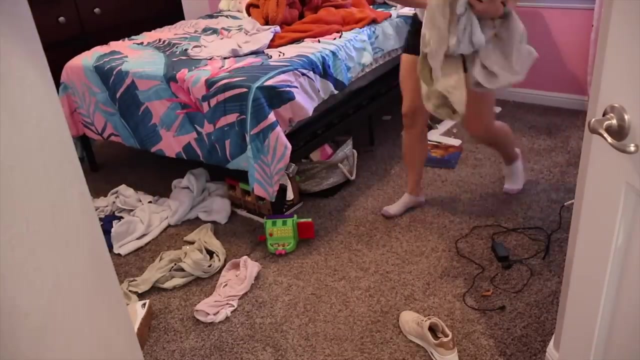 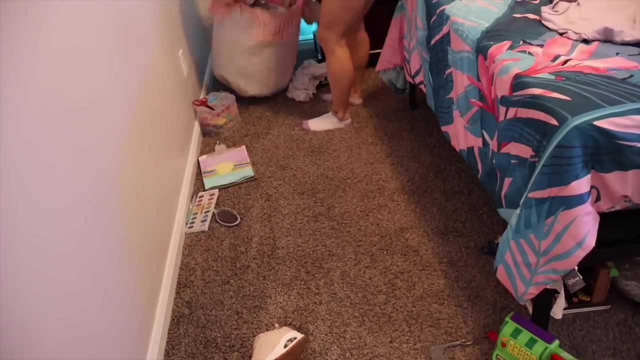 rooms. So we're going to head into Adrian's room, one of the most requested spaces for me to clean, And today is not going to disappoint, Because look how messy her room was, you guys. And this wasn't even the bad part When I got into the drawers is when it's like, Oh my goodness, she loves to save every little bit of paper. That is her thing. She loves doing arts and crafts and making things, and then she just stores them all into her drawers. So 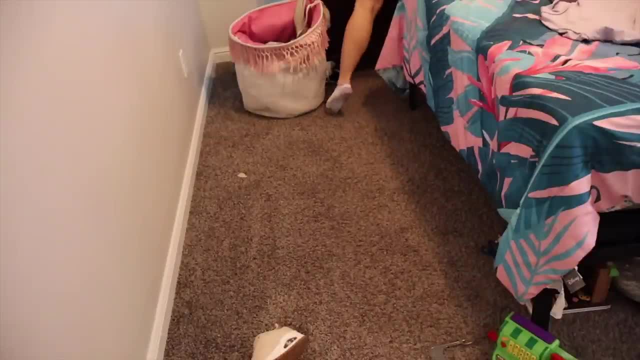 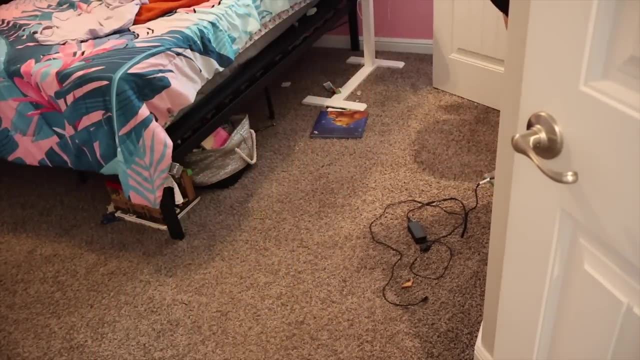 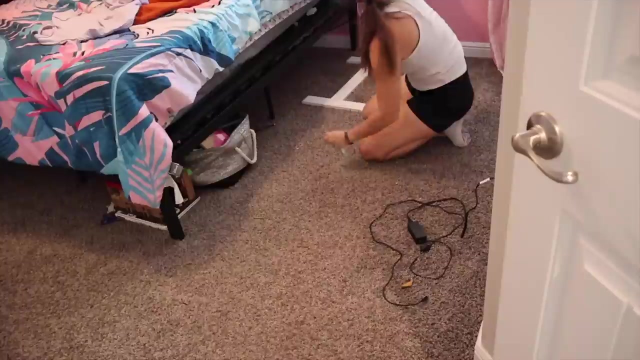 we're going to go through it, we're going to declutter, we're going to organize it, And it feels so good when I get done. I'm also doing a lot of deep cleaning because I noticed the other day which my kids usually always have their fans on. They're kind of like me: they can't sleep without the fan on. They just prefer having you know that light breeze going. So I typically don't notice their fans because they're always on. Well, the other day I went in and the fans that were in the kitchen- they were always on. So I'm going to go in and I'm going to clean it out. I'm going to clean up the movedions a little bit more. I got them all clean, So I 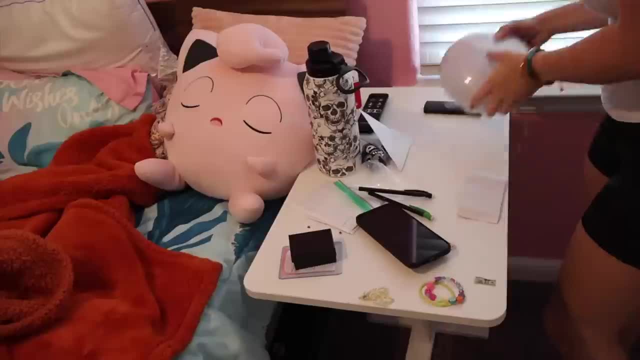 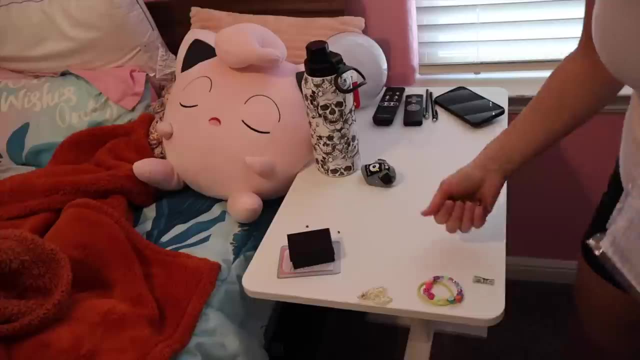 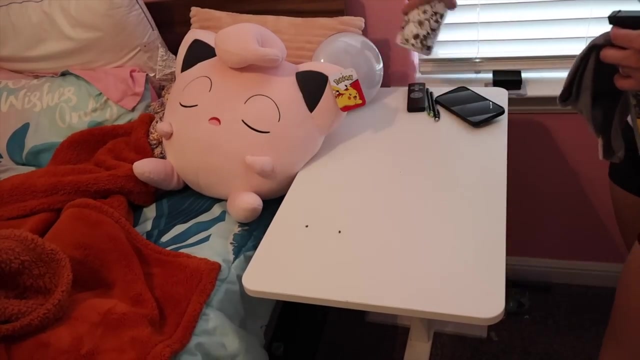 hands were off and, you guys, there was a probably half an inch thick of dust on the edges of my girl's fans. I could not believe it was so filthy, So I put it on my to-do list and I knew I was going to be tackling it today because it was so bad And since I was going to be doing the deep. 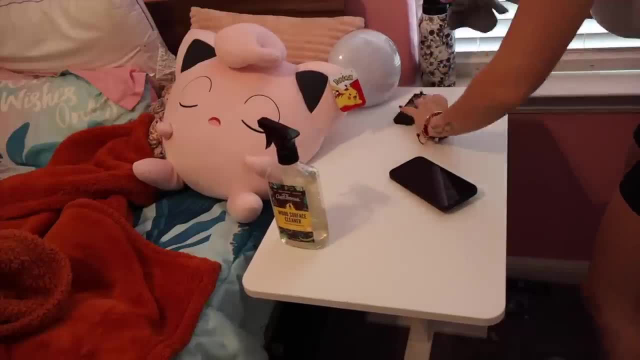 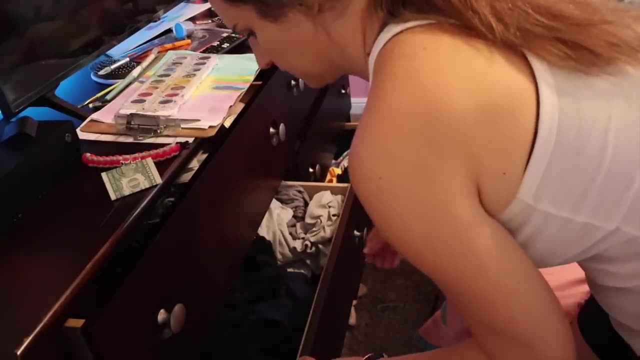 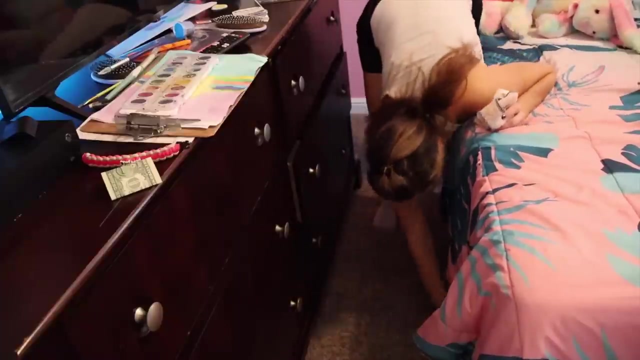 cleaning. I was like you know what? I haven't cleaned Adrian's curtains since we bought them because she has this like lace- um, it's like a regular curtain and then it has lace attached to it, which is really pretty. We love her curtains, but I'm terrified to wash them because I just 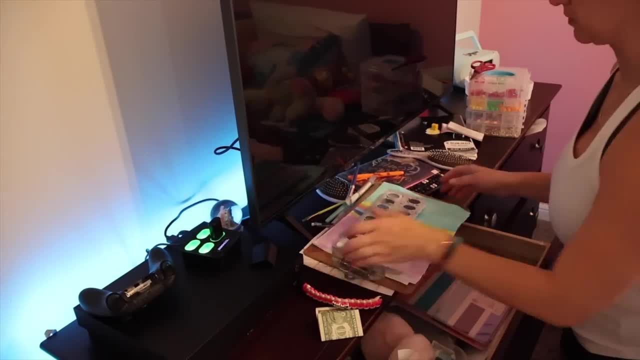 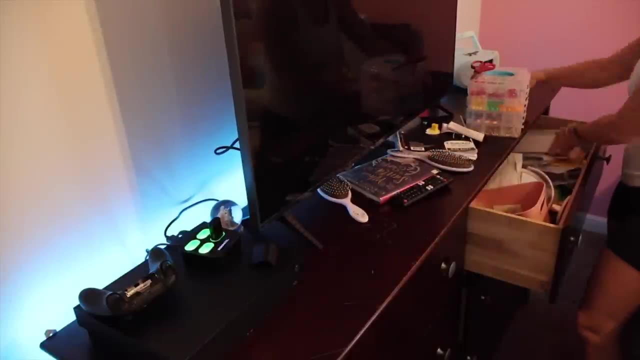 don't know if it's going to mess them up. So I thought you know what, while I'm in here doing some deep cleaning, I'm also going to shake the curtain out to get all the dust out of it And then also go in with my steamer to try to kill any germs, sanitize them, get any allergens. 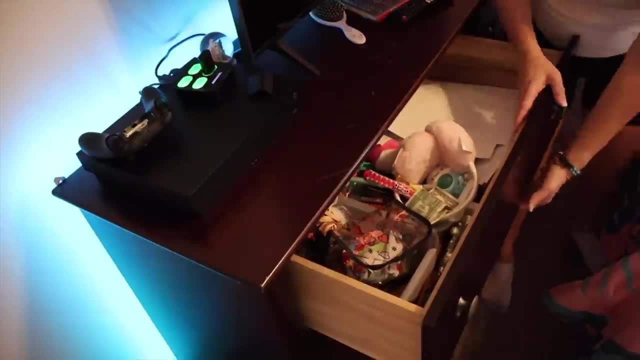 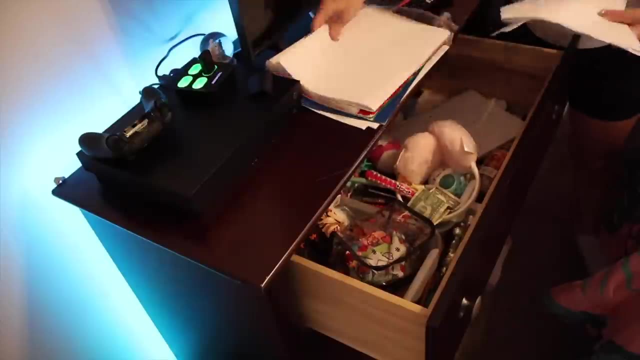 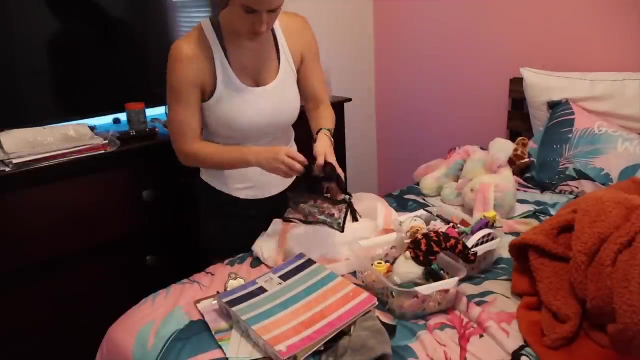 off Of them. So this room was like a complete one- 80 transformation- And I know for a lot of people looking at this mess can feel very overwhelming, which is totally understandable because, I will admit, even for me, whenever I'm decluttering a space I get the feeling of just like being 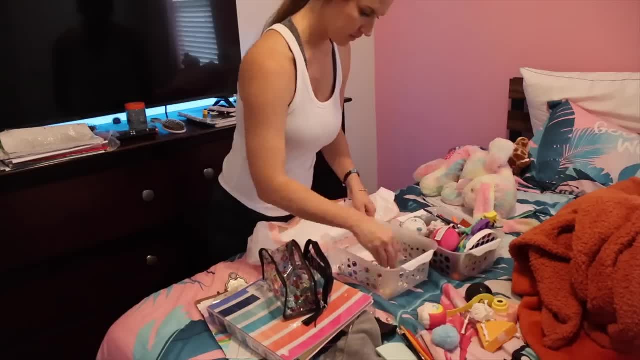 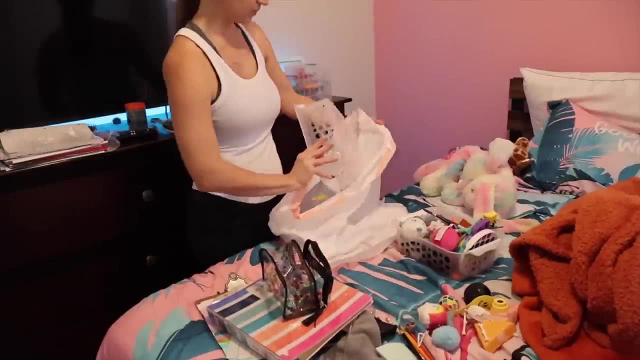 overwhelmed. Where do I start? What do I do first? So just know that if you get those feelings too- and it often it scares you away from decluttering, just know you're not alone. We get, we all get those. 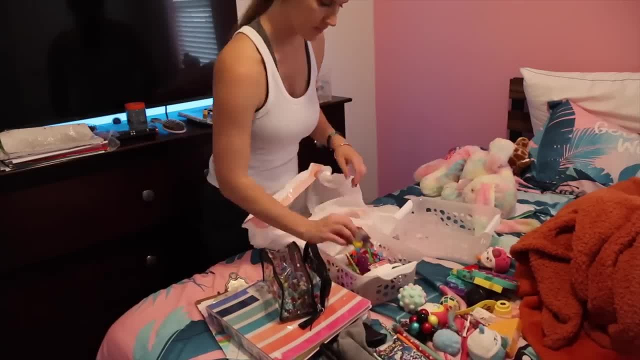 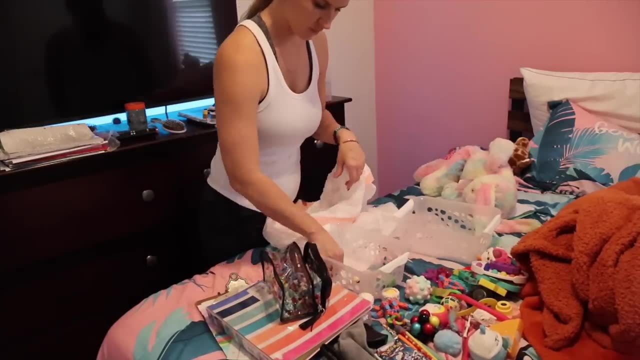 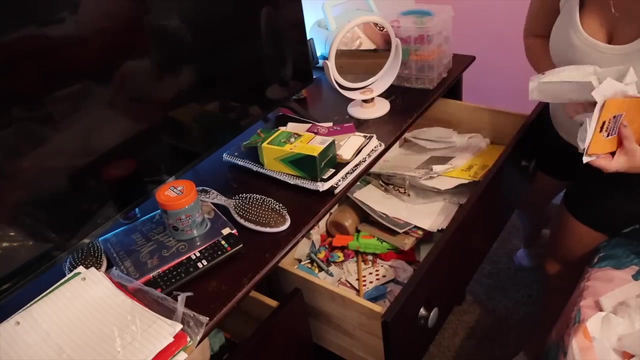 feelings and it's okay, You can work through it And whenever I get that feeling, I try to just slow down, take a breath and try to focus on one thing at a time. So I will open up just one drawer, focus on that one drawer And then, once you get that one space organized, it really does give you. 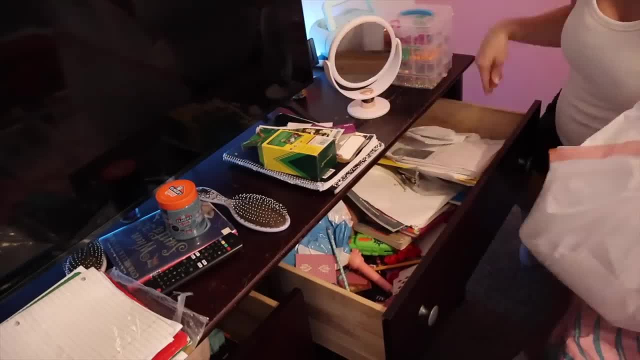 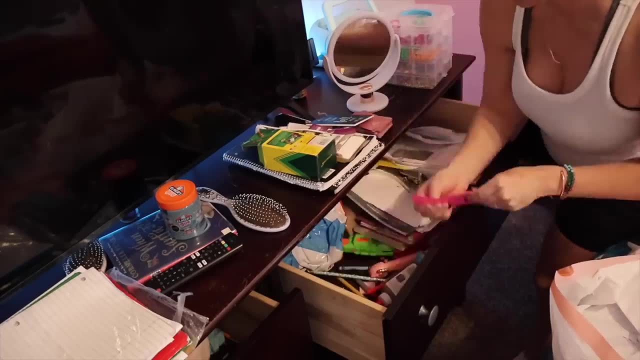 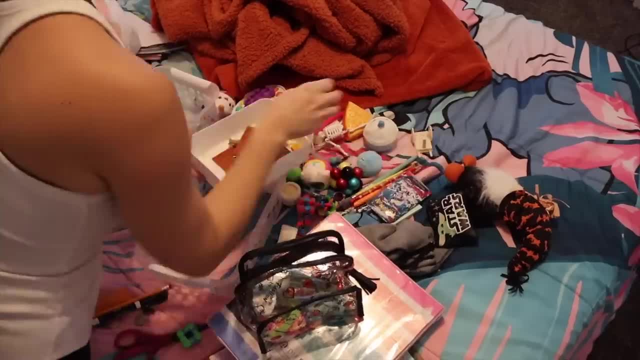 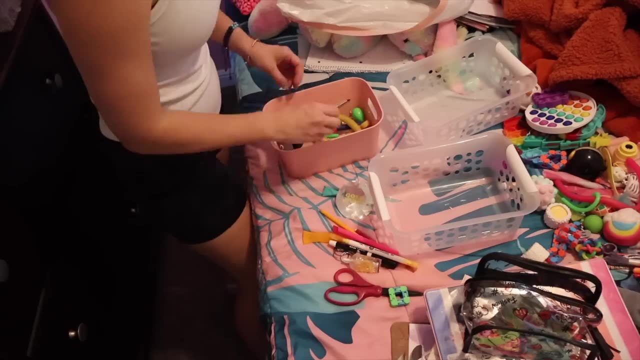 eventually that is going to add up And before you know it the space will be completely decluttered. So don't feel like if you can't do it all, then you should do none. That is the wrong way to look at it. So if you only have a little bit of time, 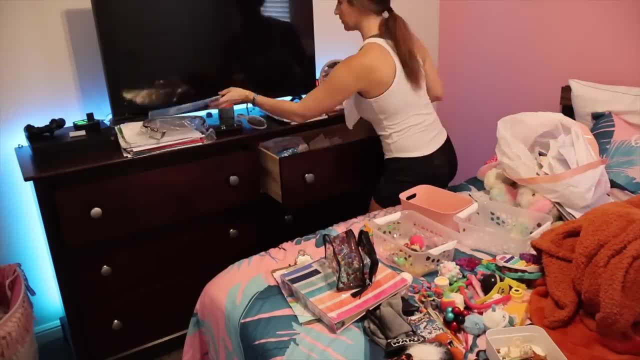 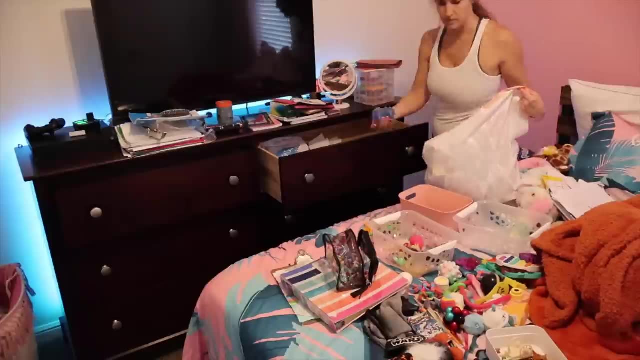 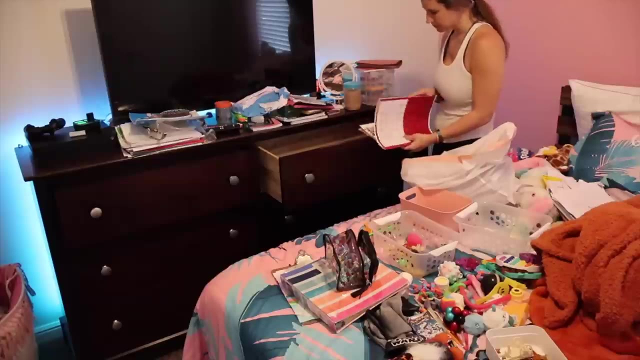 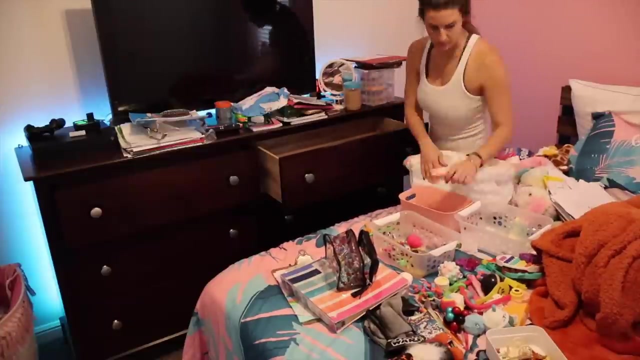 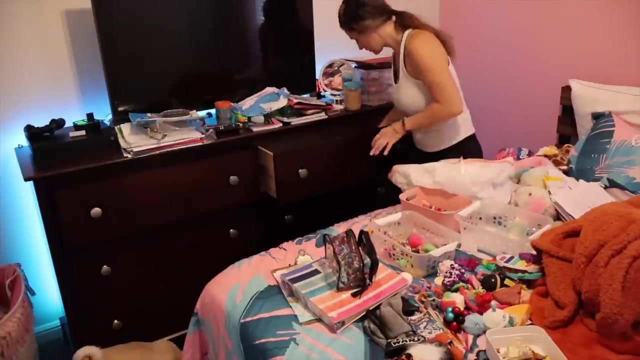 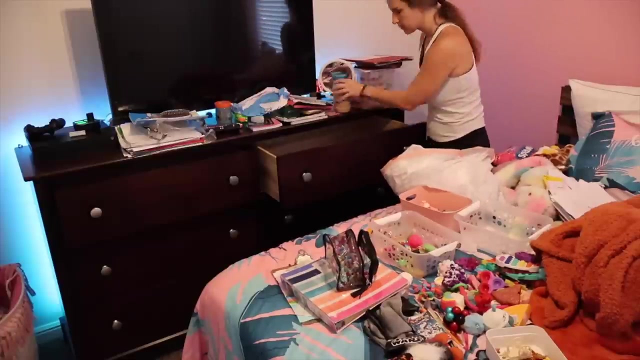 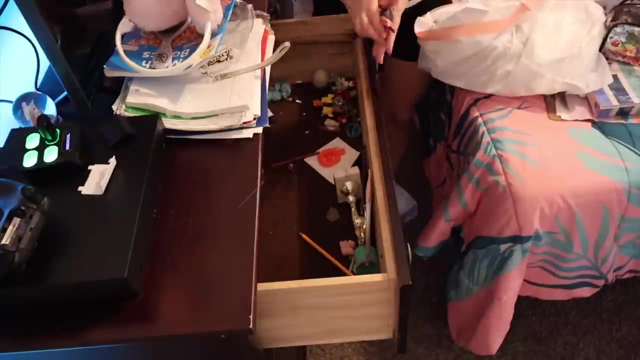 work with what you have. give yourself some grace, because decluttering is no easy task. So let's get started. Something that I kind of wanted to bring up in case maybe you think this way or maybe you know someone who thinks like this, but I was actually having a conversation with a friend who was 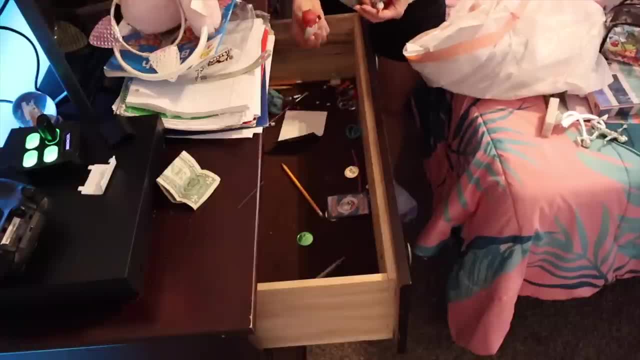 talking about like I don't know how you do it. Like, how do you get everything cleaned up? How do you keep it organized? They often feel very overwhelmed, And even when they do clean, they just feel like they're not doing it right, And so I was like I don't know how to do it. 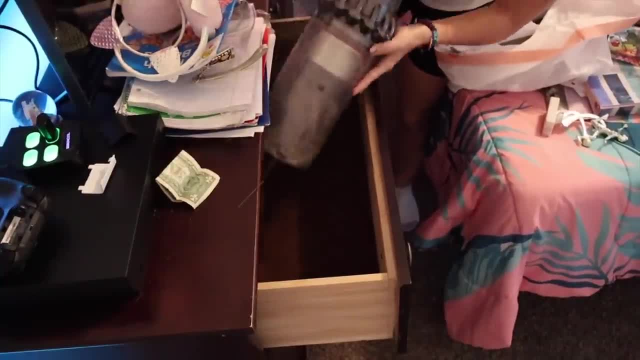 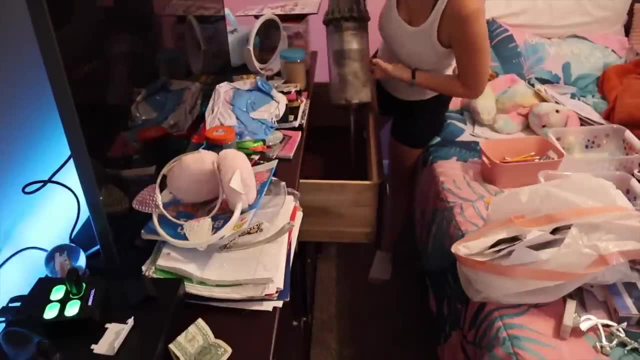 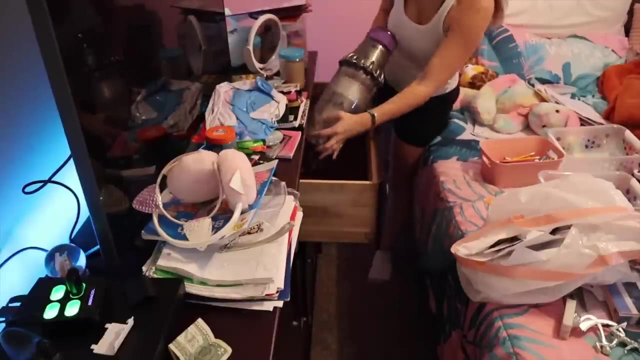 struggle with throwing anything away because in their mind they just see price tags and how much they spent on it, which is so understandable. You guys, I really struggled with that too When I first just started feeling that overwhelming feeling like I had too many things I couldn't. 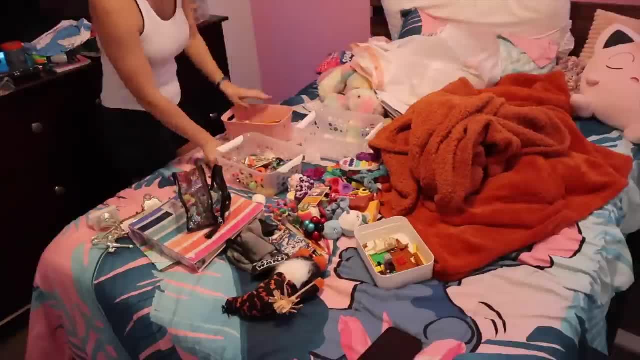 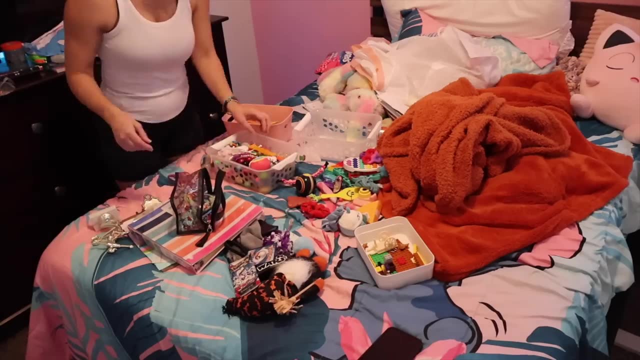 find a space for them. but then I didn't want to throw them away because I felt like I was just flushing my money down the toilet And it is understandable. but what I had to do to help shift my mind frame away from that and to look at it in a different perspective. 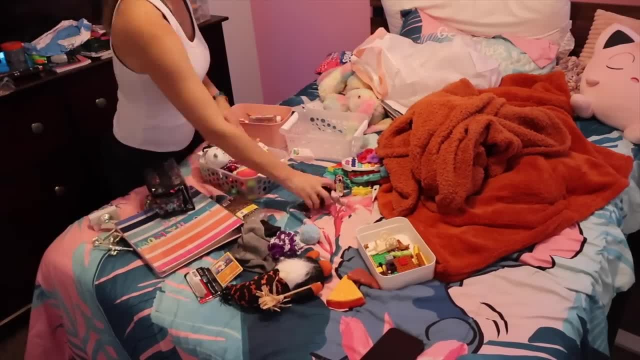 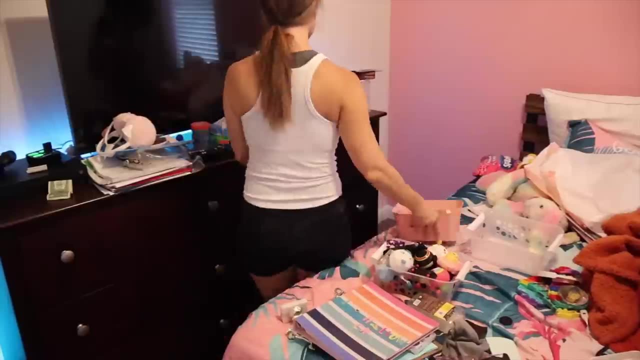 and it really helped me because otherwise I really wouldn't have thrown anything away or donated anything. But what I like to do now is ask myself four little questions. One: how much did it cost? Two: how long have I been living like this? And three: 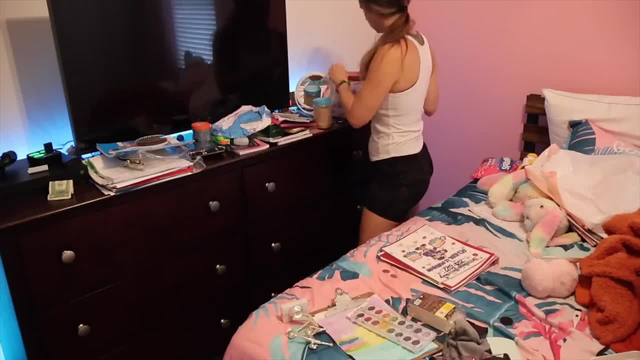 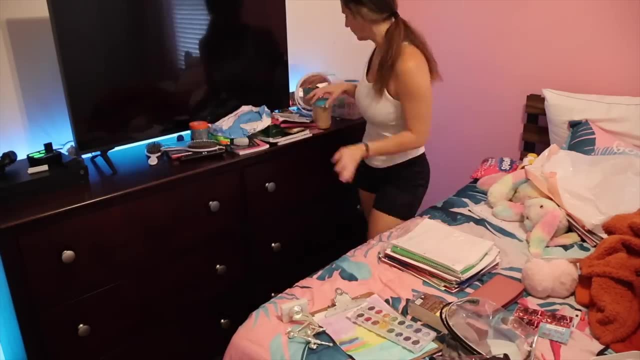 how long have I been living like this? And four: I had it. Three: do I use it Or when was the last time that I used it? And four: does it bring me happiness? And whenever I ask myself those questions? number one, I like to look at the 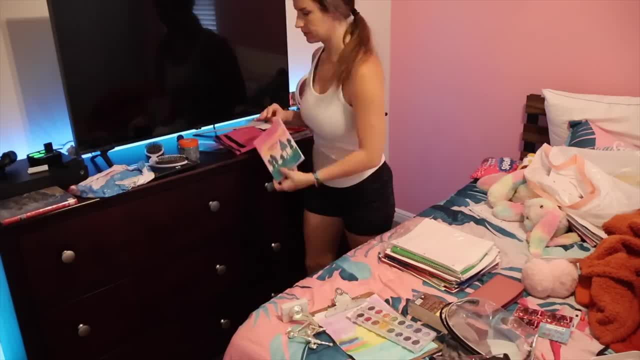 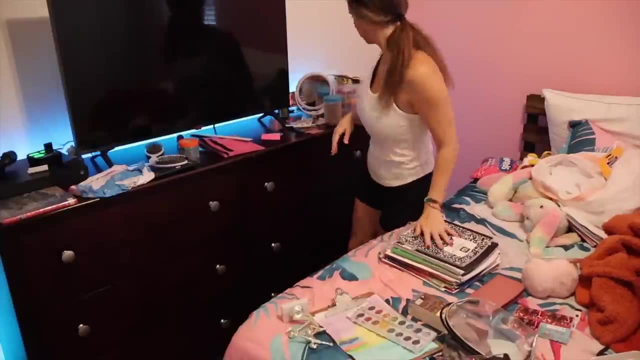 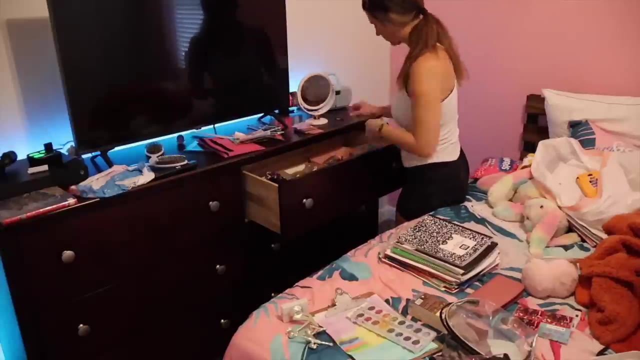 biggest one. The biggest one is: have I used it? If you have not used it in over six months, you likely won't use it in the future. Of course there's exceptions, like seasonal things, decor stuff, like that. You can make it a little bit longer, Like, okay, have I used it in the last? 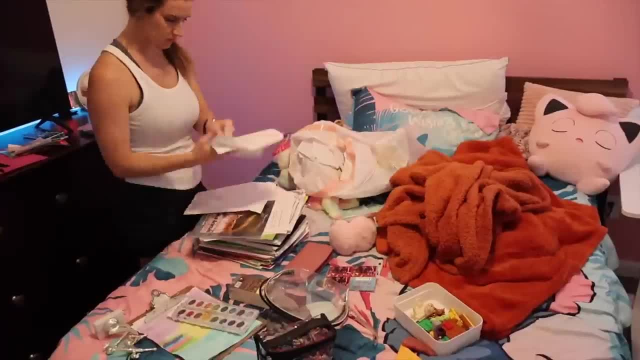 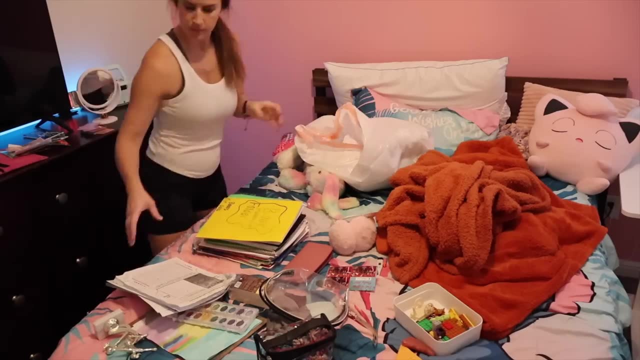 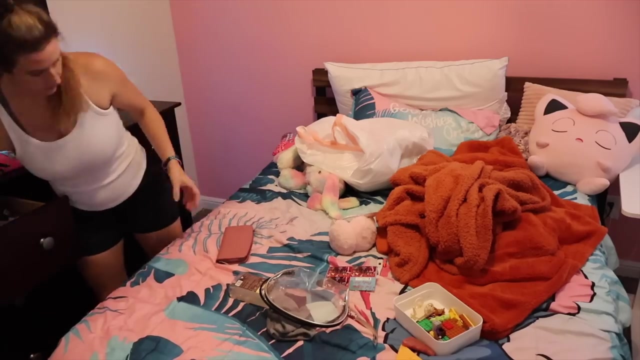 two years Does it bring me happiness? But when it comes to your everyday household items or even your clothing, you want to ask yourself: have I used it in the last six months? Does it still fit me? And if I didn't spend that much money on it, did I get my money's worth? Do I feel like okay? 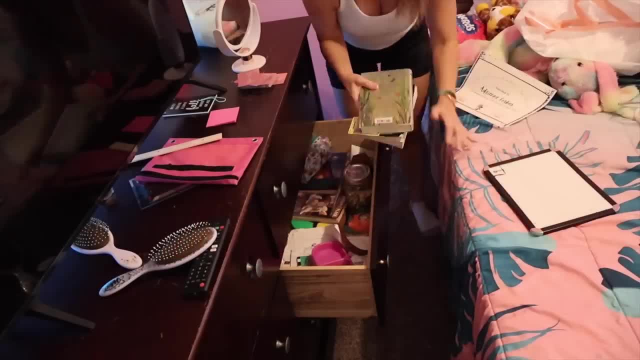 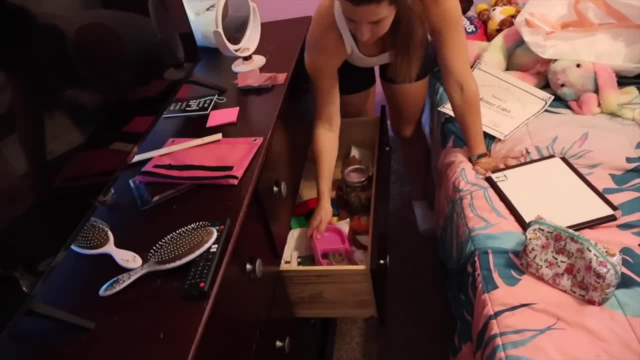 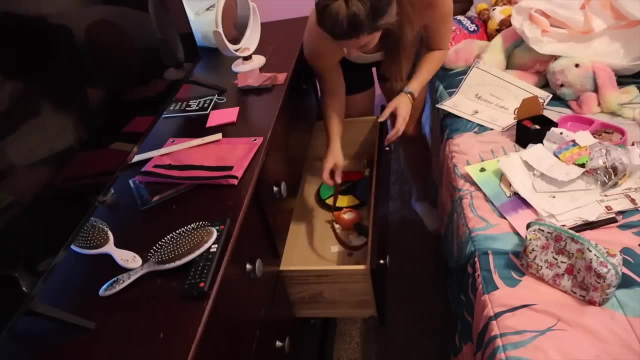 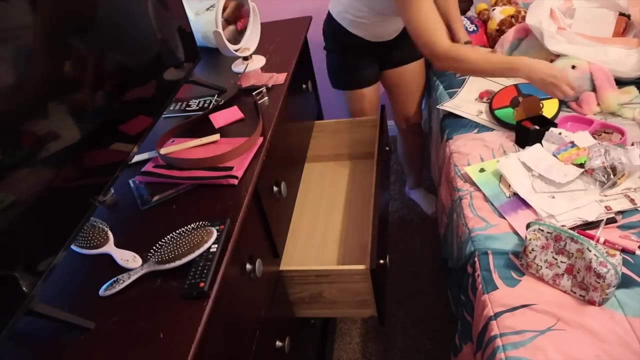 $20,000 on it, Do I feel like I got my money's worth, And that really helps me shift my perspective on things and make me realize like, okay, yeah, it really wasn't that expensive. I got my money's worth out of it And now I'm ready to donate it or sell it in a garage sale. 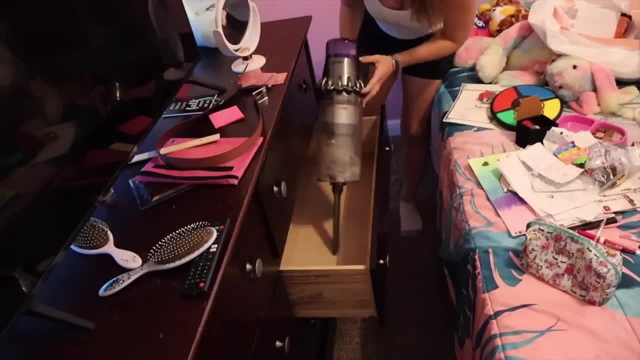 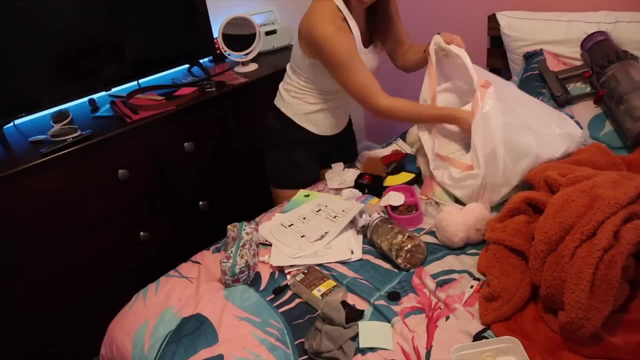 and help someone else out who might be looking for this item but can't pay, you know, full price for it. So those are just some of the things I ask myself And it really helps me out a lot because, honestly, you guys, I really did struggle with decluttering. I would shift things. 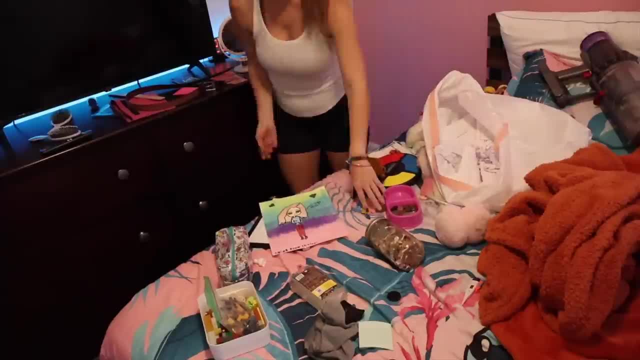 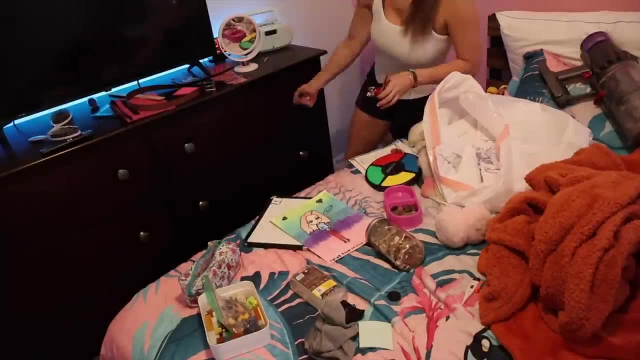 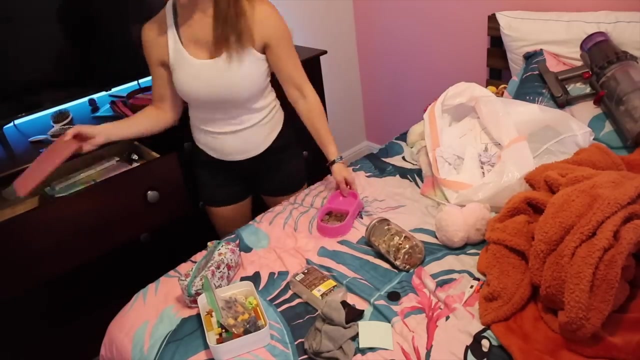 from one bin to another, from one closet to another one, And my husband used to tell me all the time that I was a pack rat. So I know the feeling and I know the struggles are real, but I promise you can get through it. Baby steps, start in one little space and work your way. 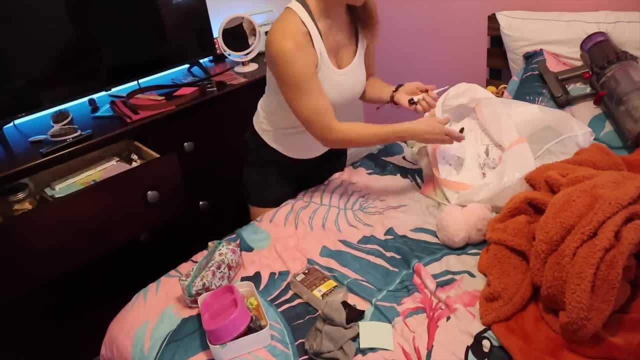 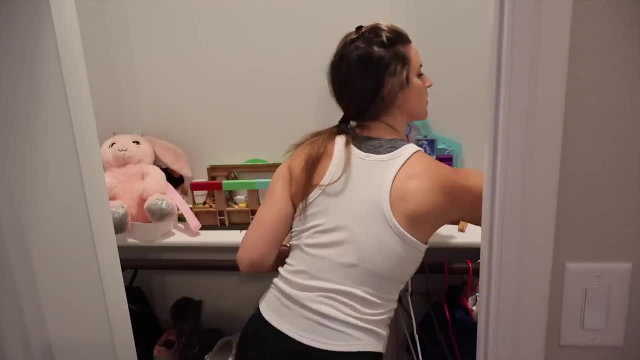 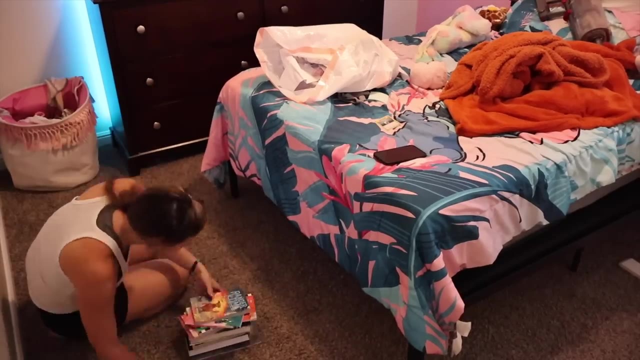 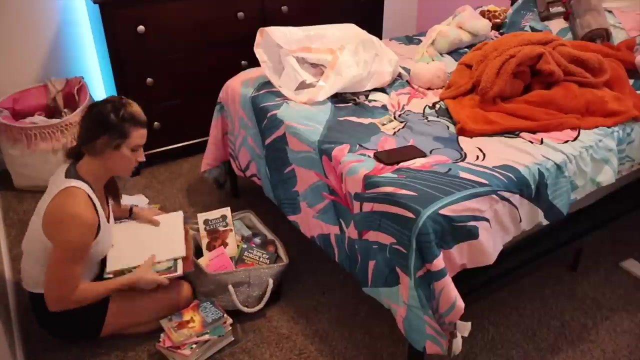 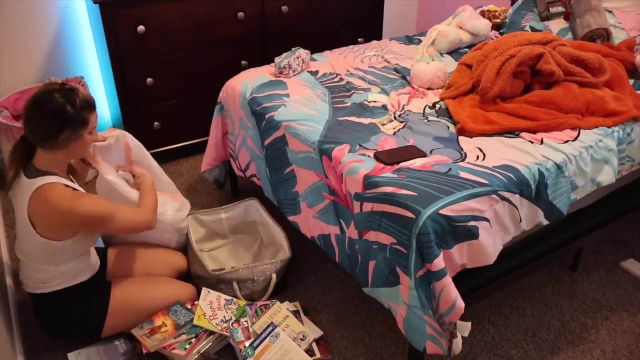 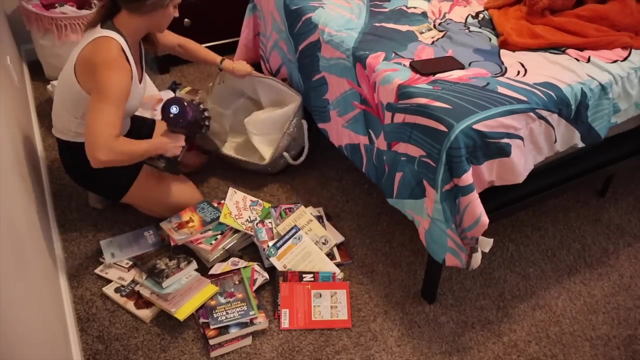 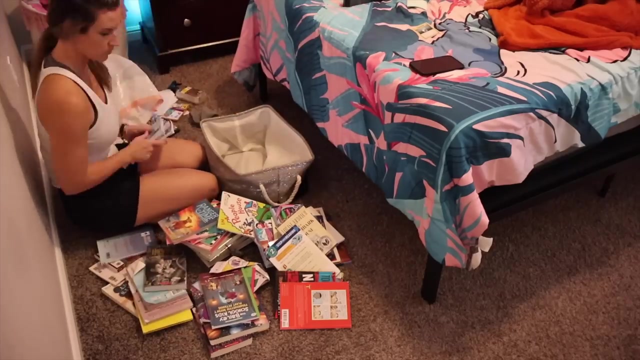 around And eventually your home will be completely decluttered and organized. So while I was organizing, organizing Adrienne's dresser drawers, I did find a lot of books in there, so I went ahead, pulled those out, because she has a little bin under her bed that she keeps all of her books in. 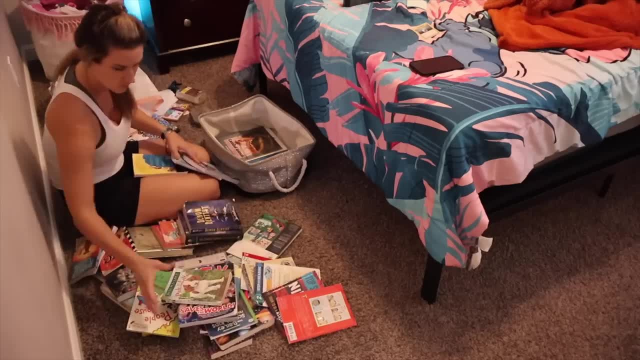 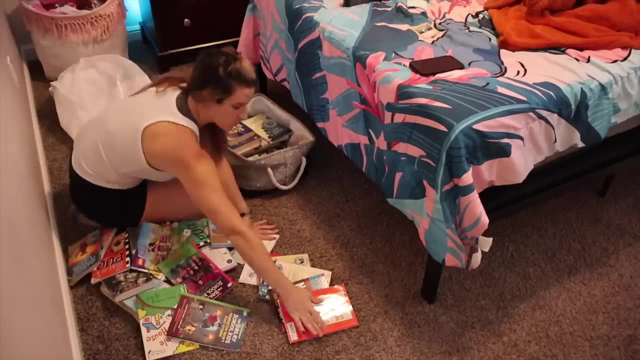 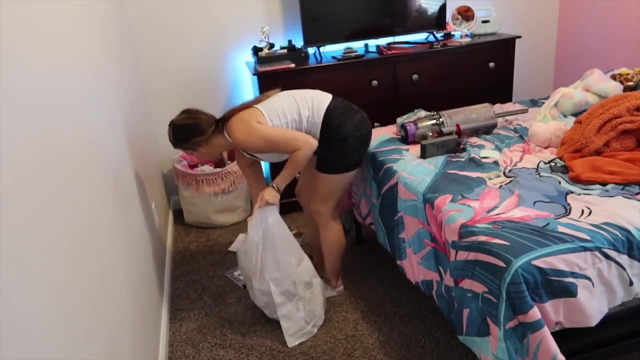 so I wanted to go ahead and reorganize those to try to fit them all in here, because her collection has grown a lot. If you guys watched, a couple videos ago, I mentioned that we went up to the library and they were having this awesome event where we could fill a bag for five dollars with 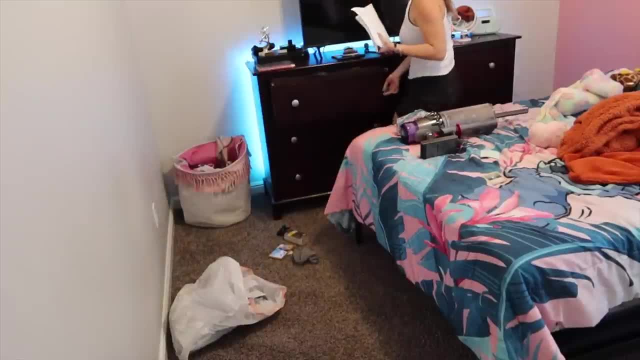 all of the books that we wanted. so now she has quite the collection. so I got it reorganized for her. It needed to be vacuumed out. There was a lot of like random crumbs in there, but now she can see all of her books nice and neatly. 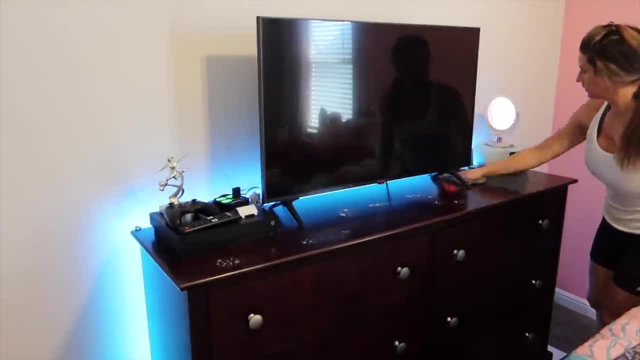 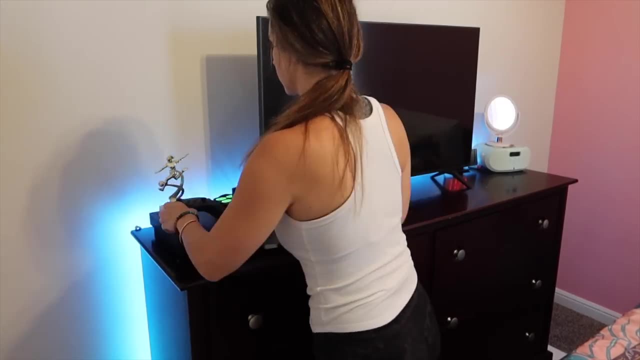 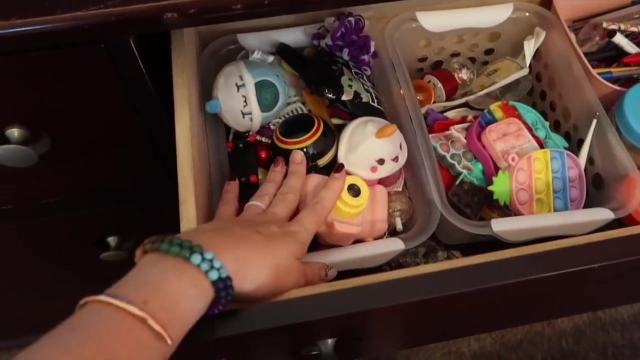 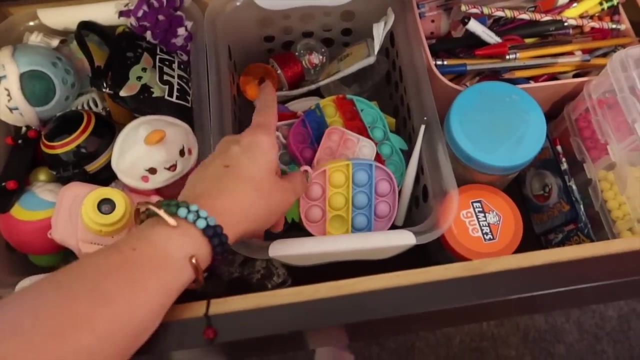 So for organization in here, what I did was put all of her fidgets and little knick-knack toys in this basket, and then I did mainly all of her little poppets, a few random ones, her slime pens, pencils, markers, crayons. 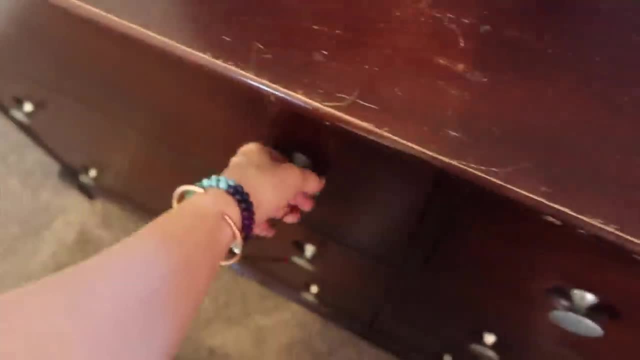 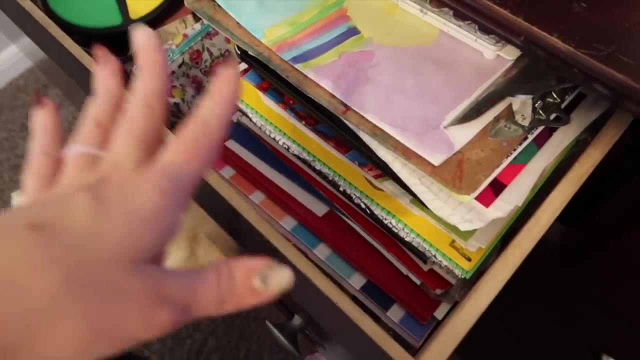 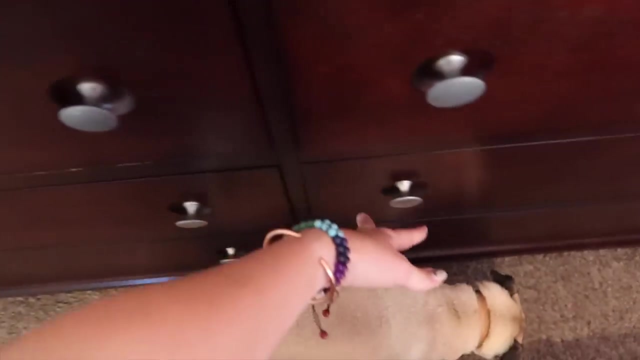 set, and then her bead set, and then in this drawer I have all of her notebooks, paper, painting stuff, all of that stacked up, and then these are just like a few random items I put in there. but what I'm really excited is I got rid of so much that we freed up this drawer. I do plan on 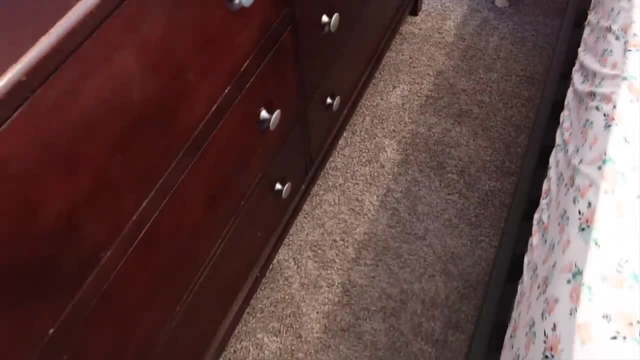 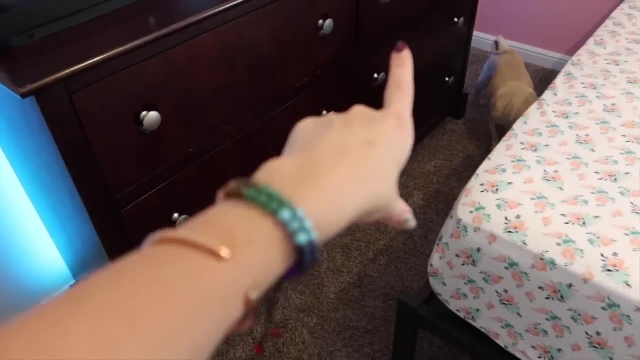 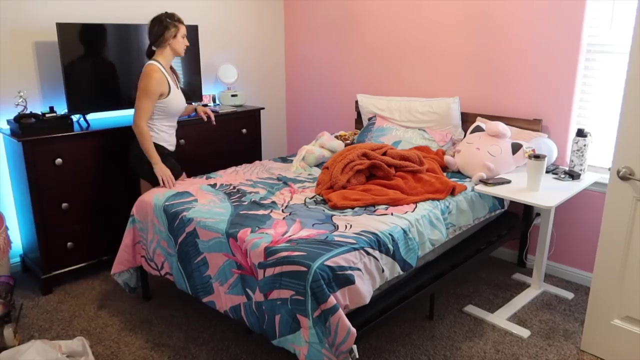 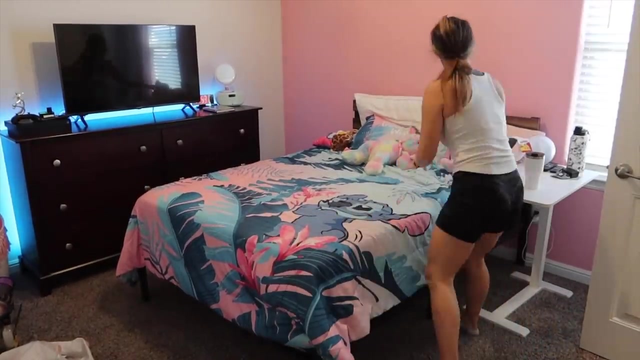 doing like a decluttering and organize in her bedroom. I'll likely be sharing that on my vlogging channel, but I need to go through her clothes and reorganize, so it's going to be nice to have a freed up drawer. I went ahead and pulled off her bedding that way I could wash it. she doesn't sleep. 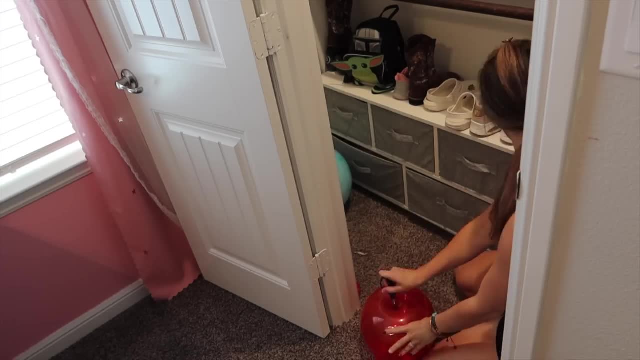 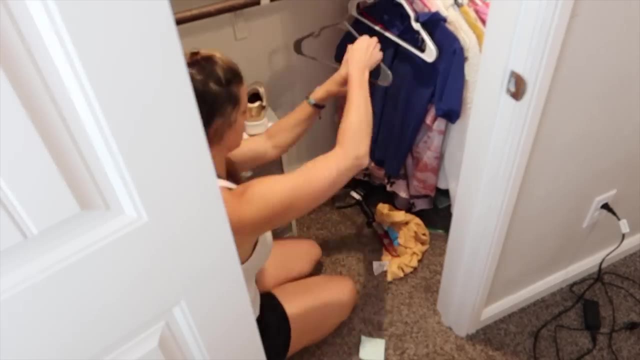 underneath of her comforter. so I was like you know what? I cleaned her sheets not too long ago. I'm just going to go ahead and do that, and then I'm going to go ahead and do that, and then I'm just going to wash the ones that she actually lays on and that looked dirty. so I pulled those. 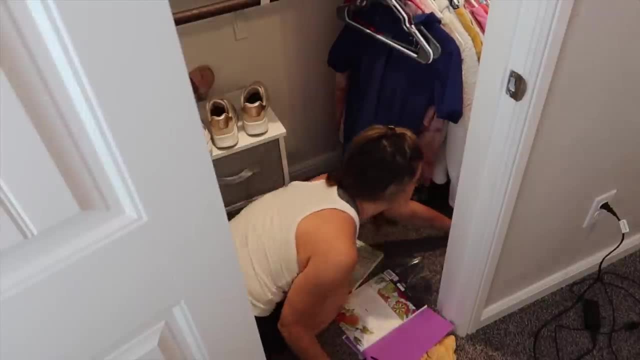 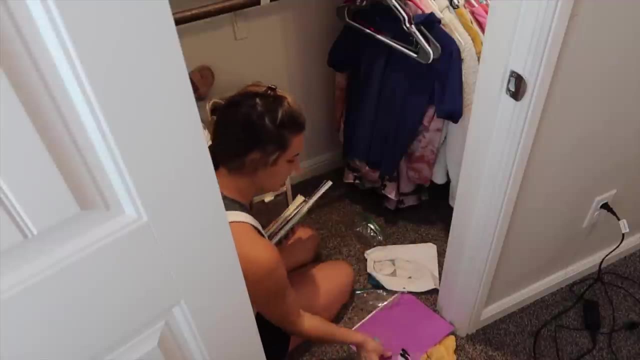 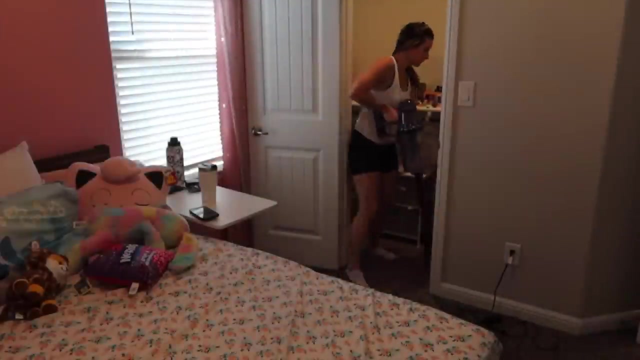 off. that way, we could get them in the washer as soon as that first load was done and now we're heading into her closet. there was a lot of random things on the floor- papers, of course- so we're just going to quickly tidy up the bottom half of her closet. I also needed to pop some balloons that. 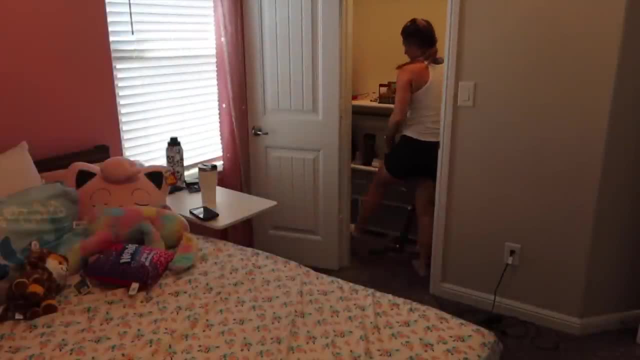 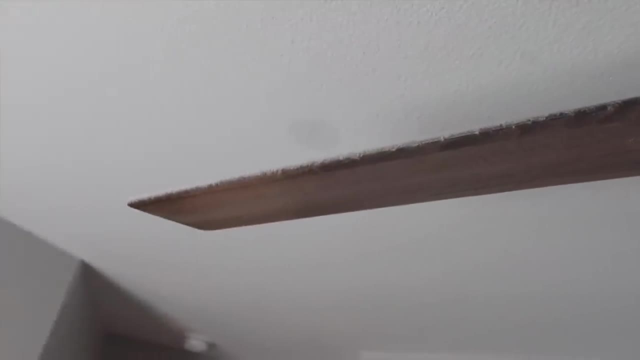 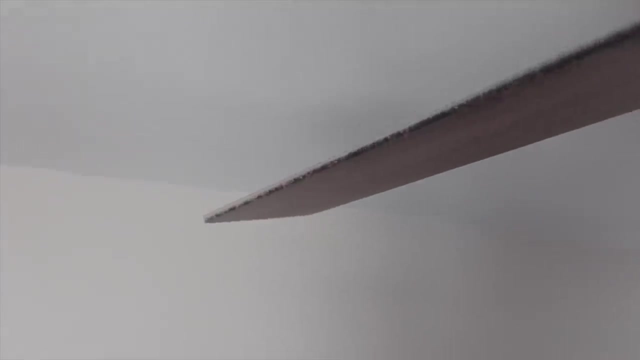 were left over from athens birthday and I got rid of those because adrian's birthday is actually coming up. it's November 1st, so I already know we're going to have a lot more balloons in the house, so I needed to get rid of the old ones, and that is the desk that I was talking about you. 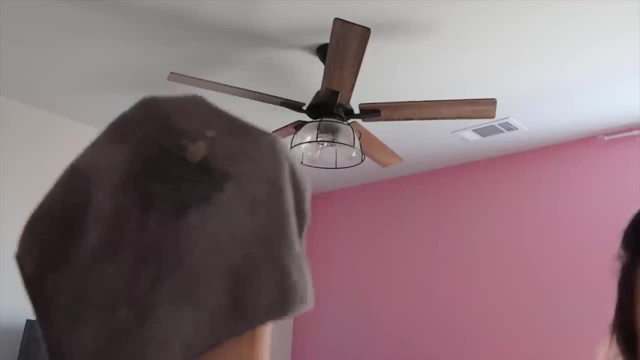 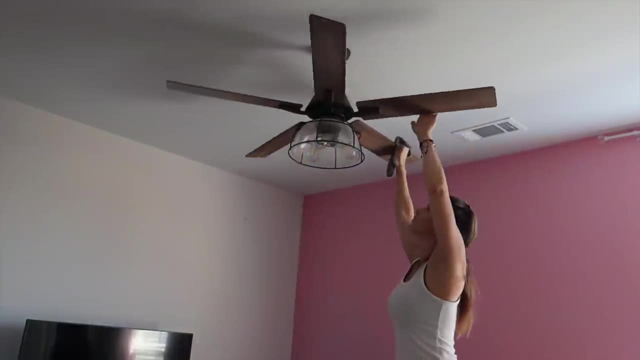 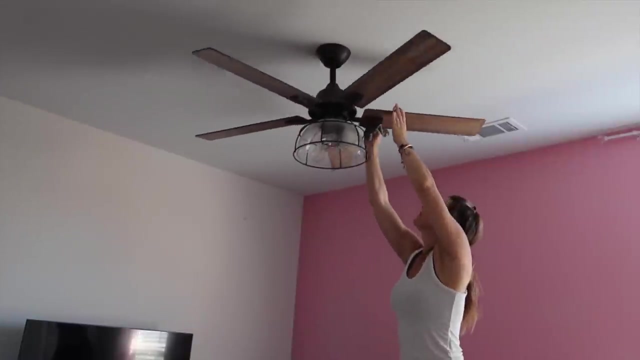 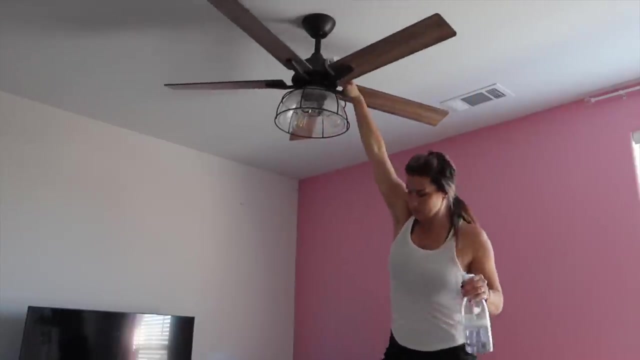 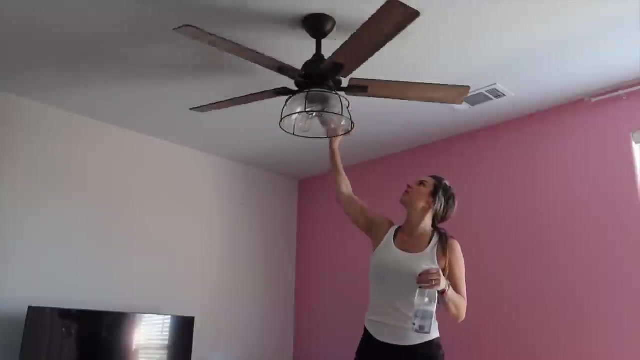 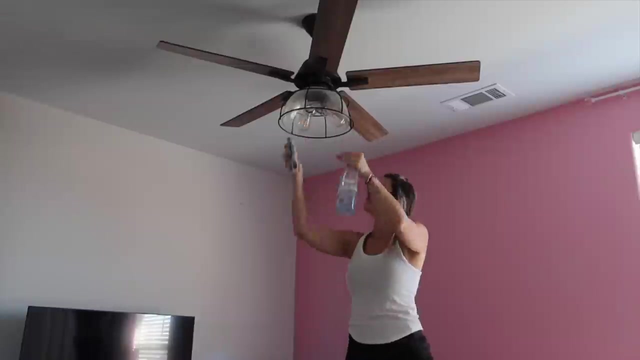 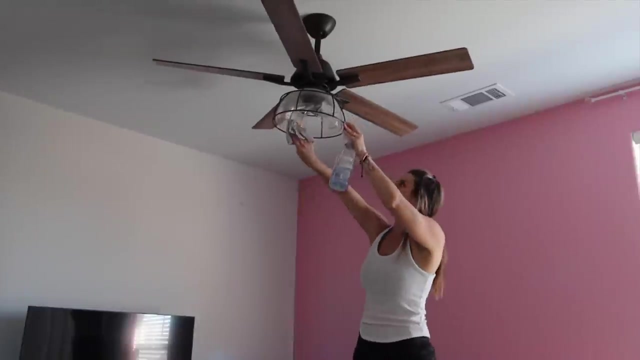 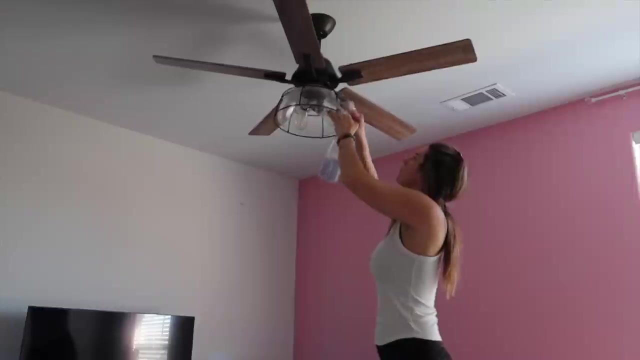 guys. it was so caked on, it was disgusting, foreign, foreign. I went ahead and got the glass cleaner so I could clean the glass, because while I was up there I realized, holy cow, the glass is not see-through anymore. there's a huge film of dirt on here. so 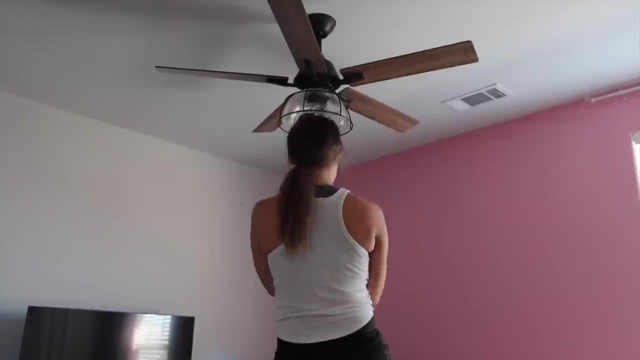 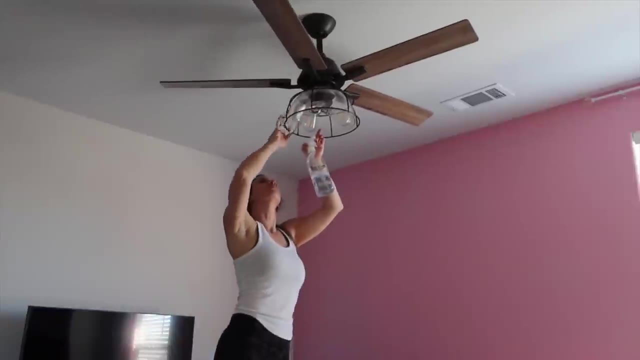 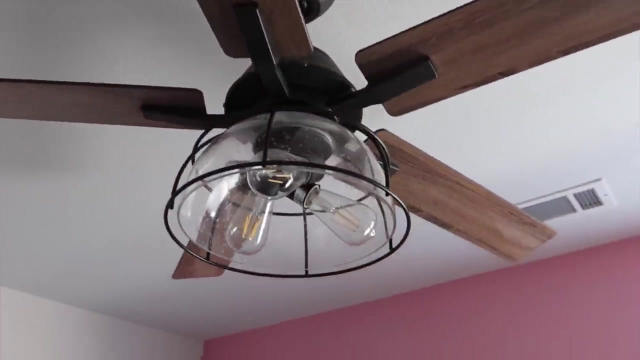 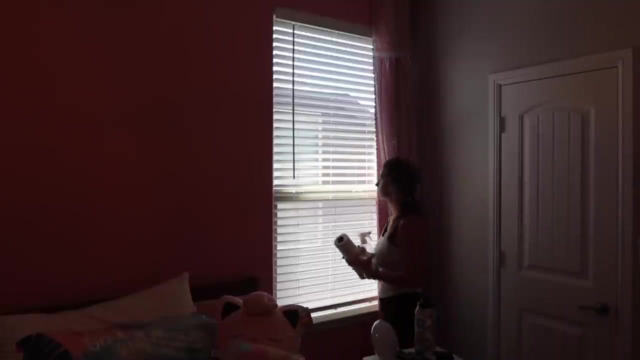 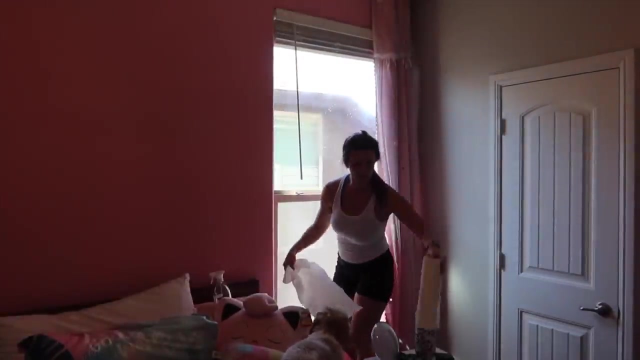 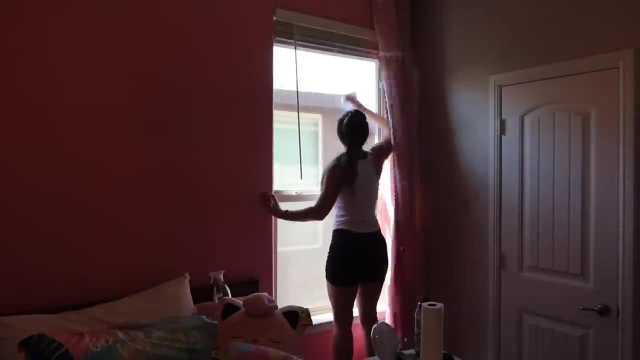 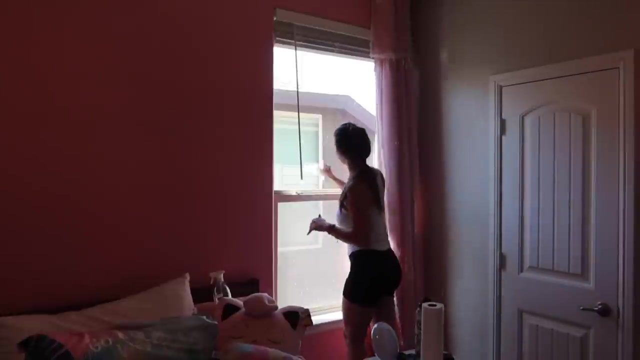 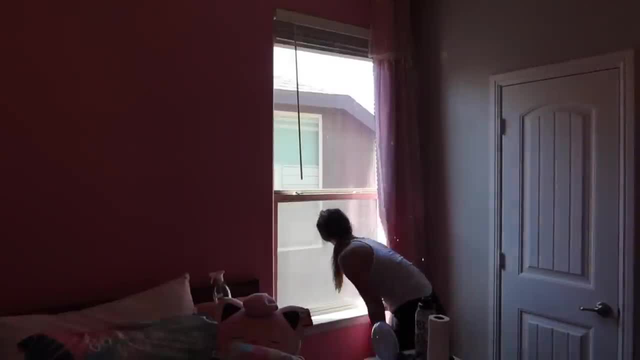 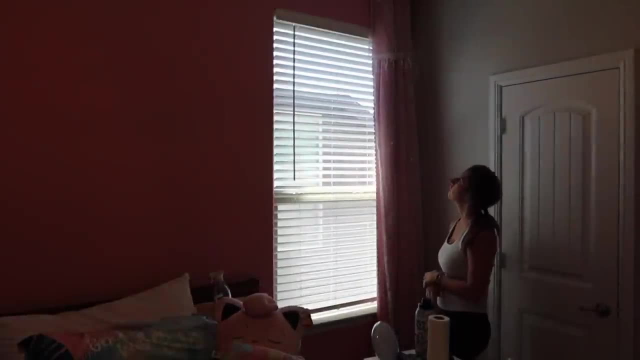 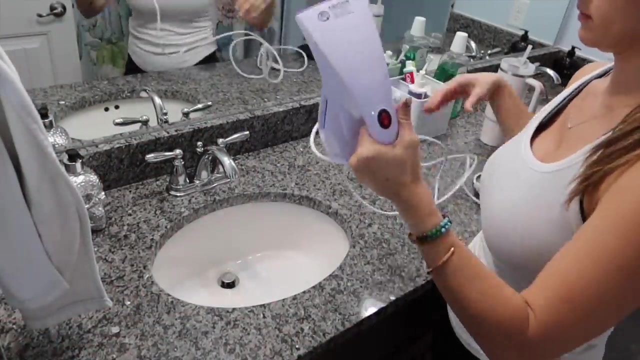 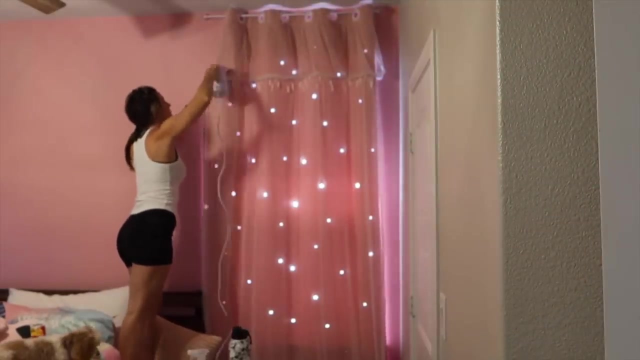 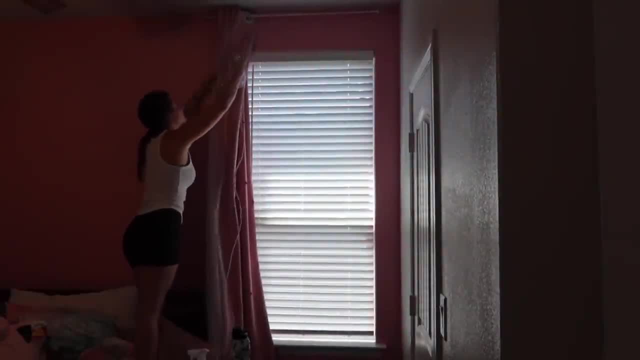 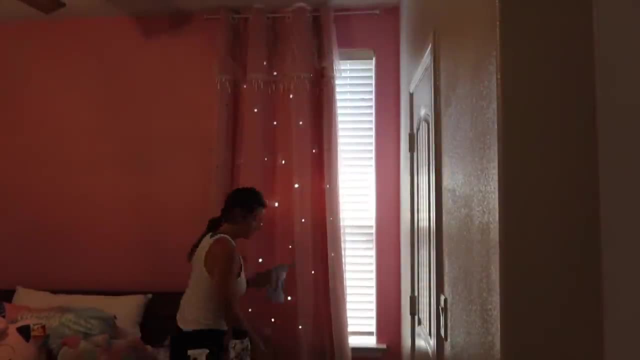 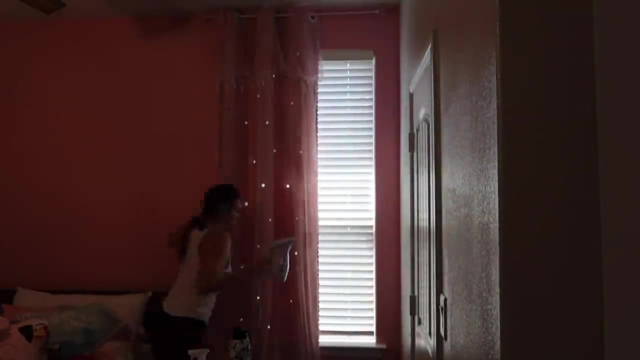 have this little handheld steamer. This is what I use for my clothes. I also have my Bissell steamer, but this one is great for like flatter items like curtains and clothes, stuff like that. So I pulled this one out. I got it off of Amazon. It was really affordable and I love it. It works. 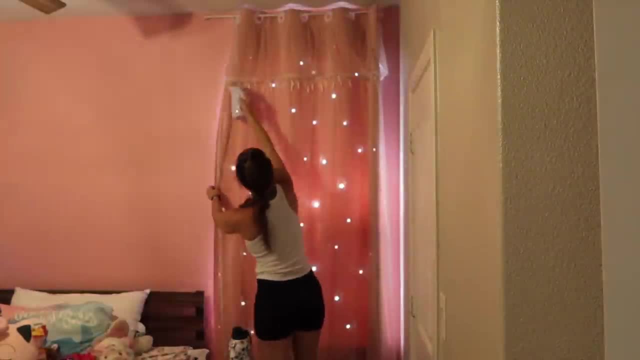 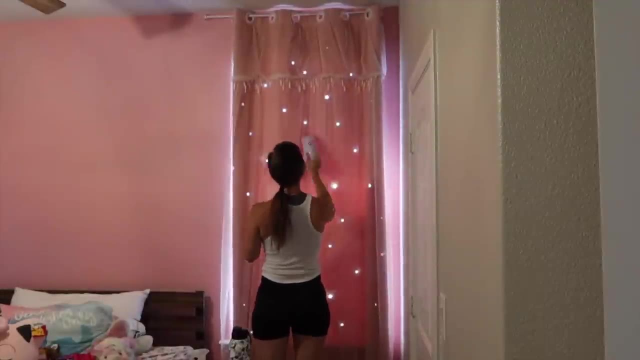 great So I'll be sure to link it in my description for y'all. But I could not believe the amount of dust that was coming off of these curtains. It was getting caked on to the tip of my steamer. I had to keep stopping and wiping the tip of my steamer because it was so dusty. I definitely need. 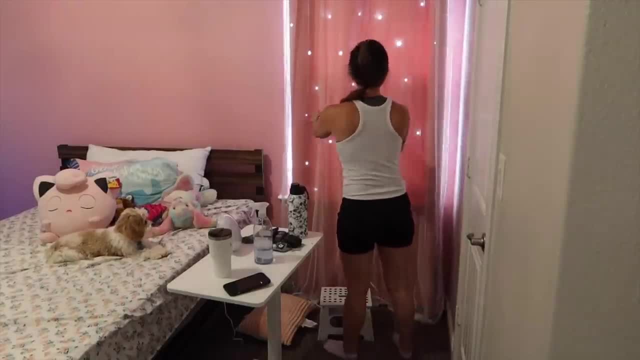 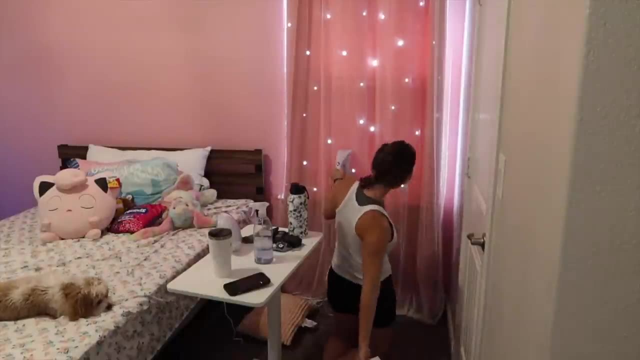 to start doing this more often, because I did not realize how much dust was trapped in here And, like I said, her curtains are really the only ones in the house that I don't wash, which I don't know. Let me know if you guys think I could wash these and just hang dry them. 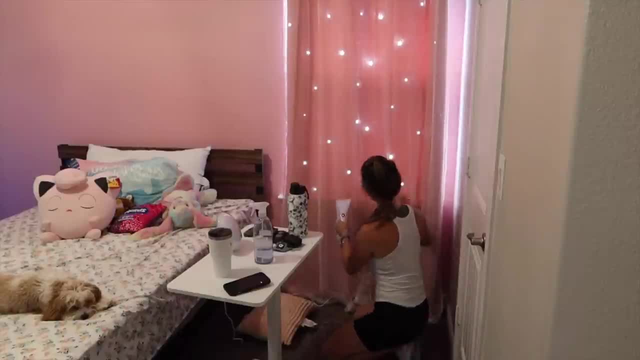 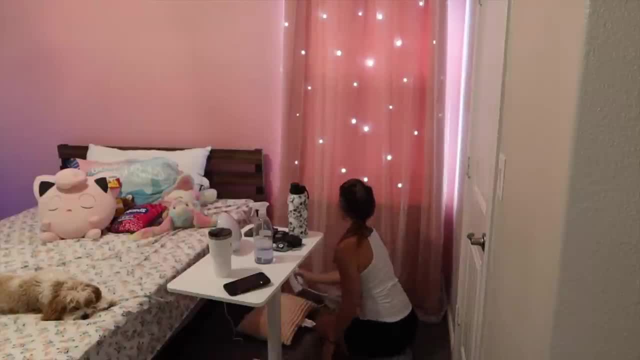 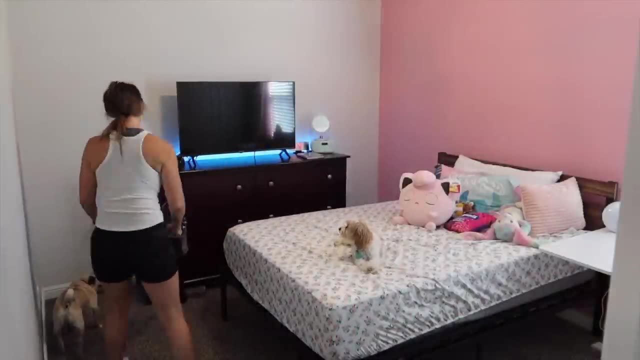 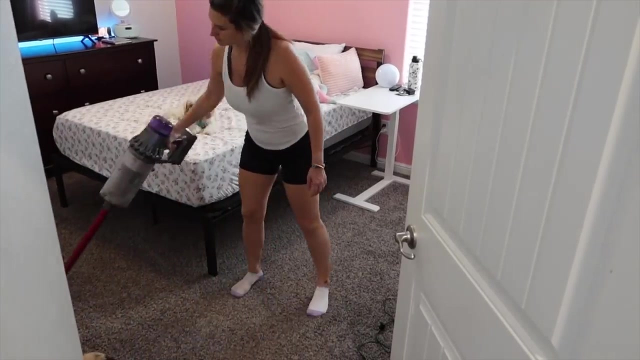 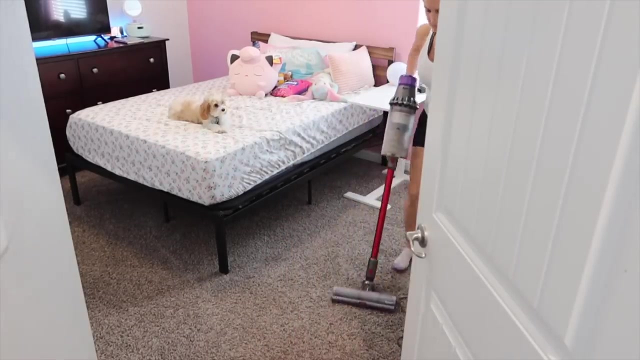 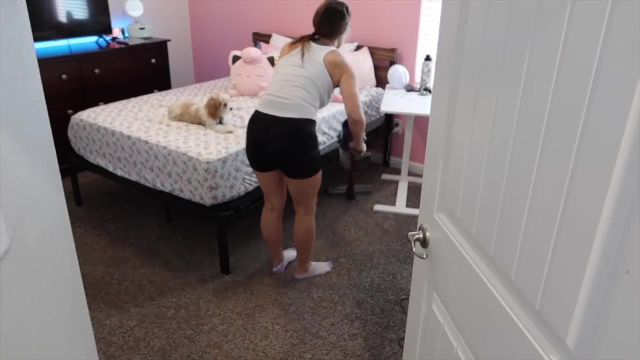 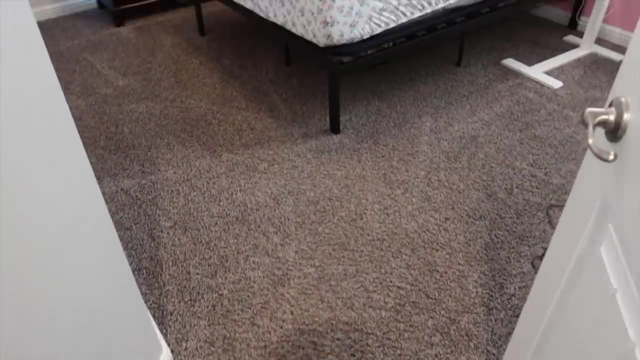 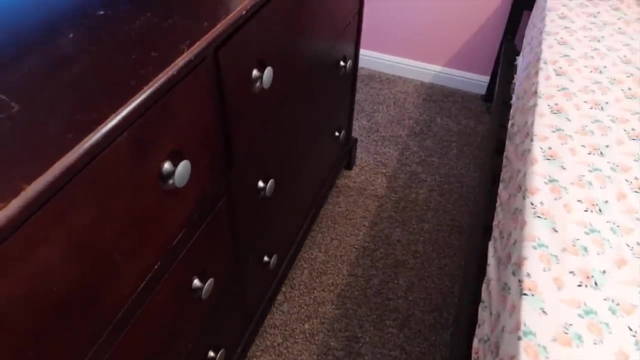 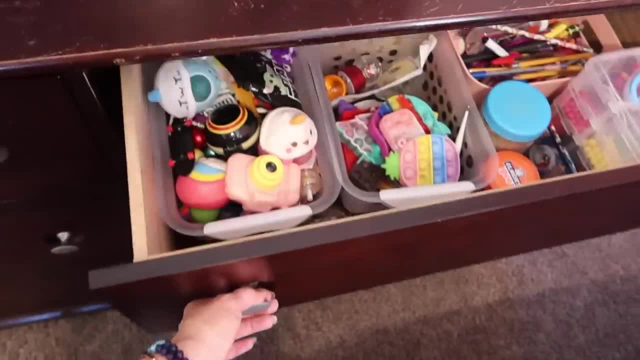 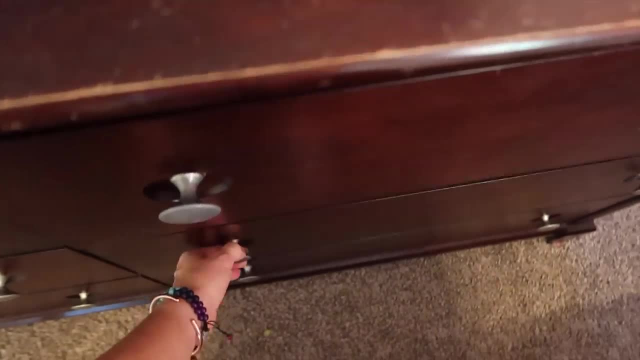 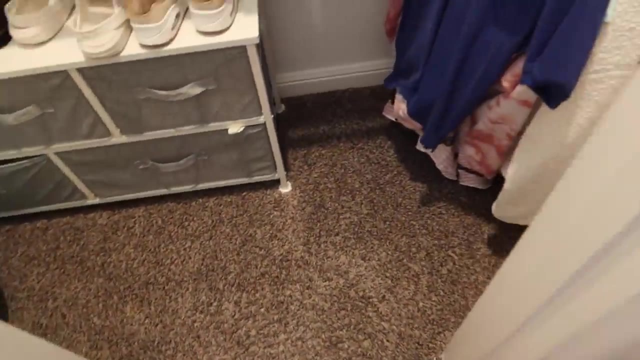 She was so appreciative Every time I clean her room. she is so sweet. She's like: thank you, mom, so much I love it. I promise I'm going to keep it clean. this time. It is honestly the sweetest And I know she tries really hard. but I also appreciate that every child is different. 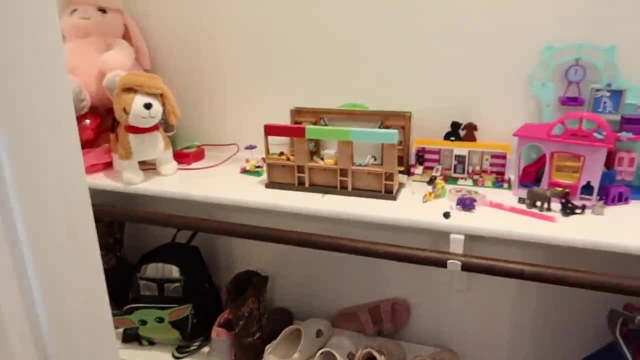 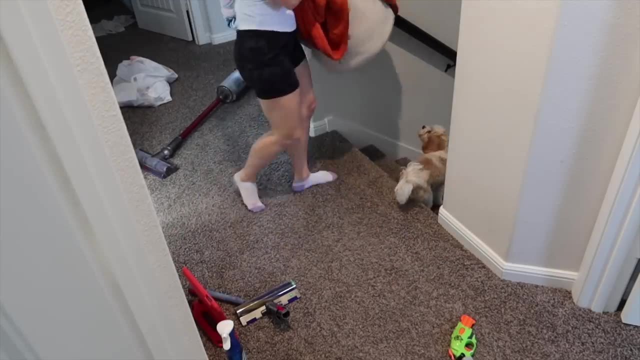 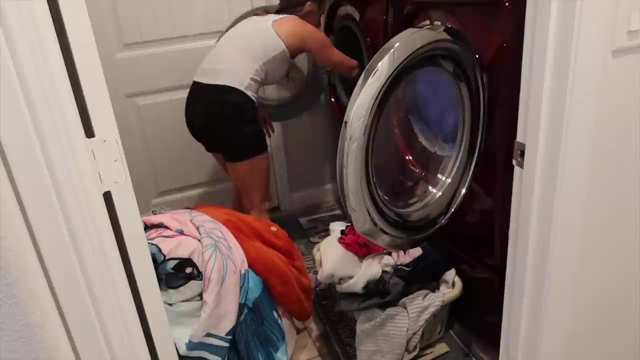 And what might seem like chaos to one person is complete serenity for the other. So to each their own. but I do try to get in there and help her out every once in a while. I do make the kids clean their rooms, but I mean, let's be honest, kids do not do that great of a job at cleaning. 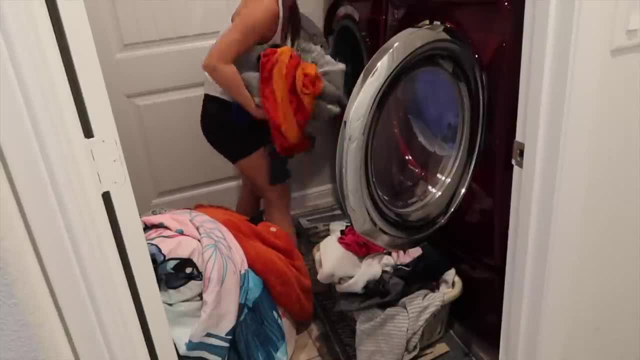 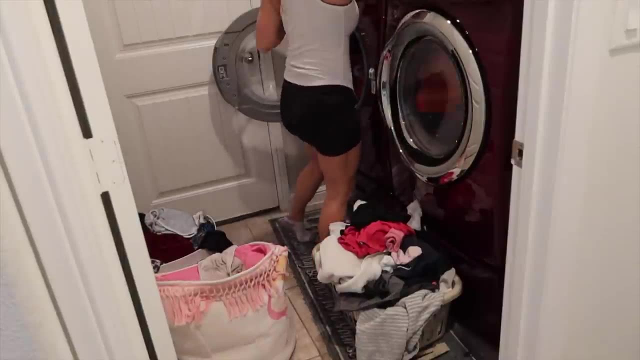 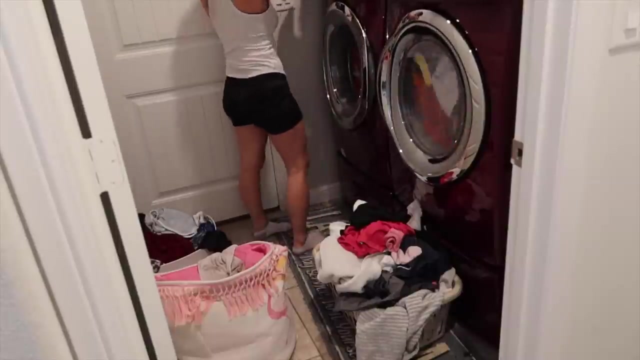 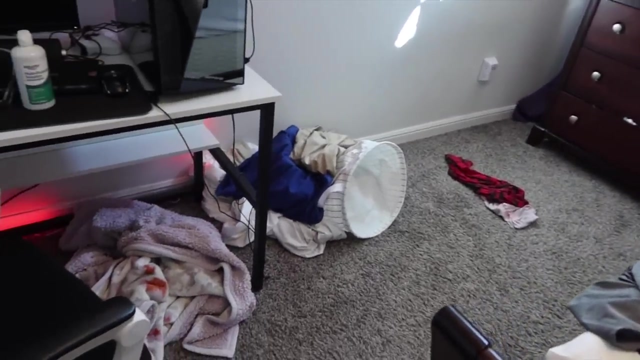 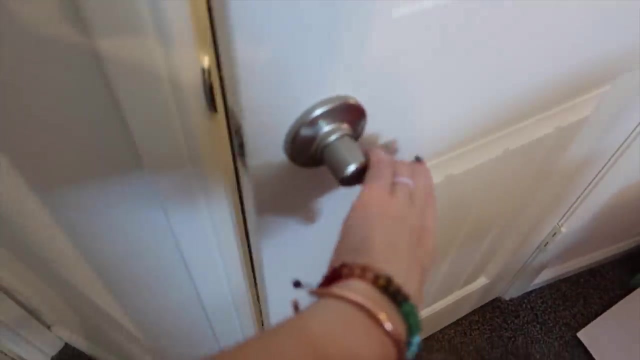 their rooms. Now it's time to head into Aubrey's bedroom. She is my oldest, She is 13 now, and her room usually isn't too dirty, But it is dusty. This is the dustiest room by far. It doesn't matter how many times I come in here. 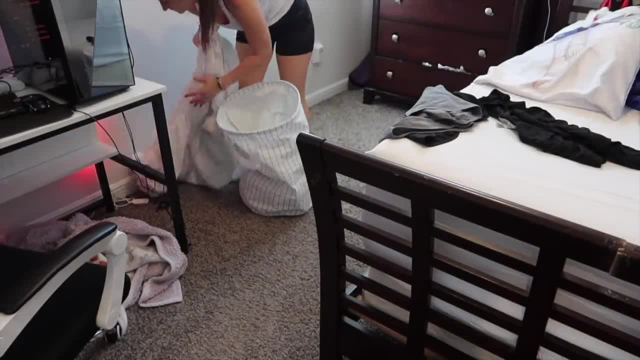 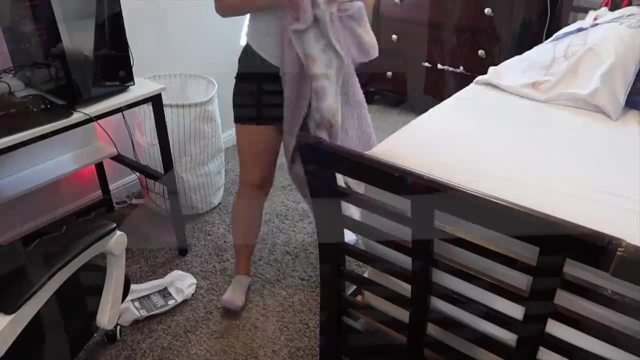 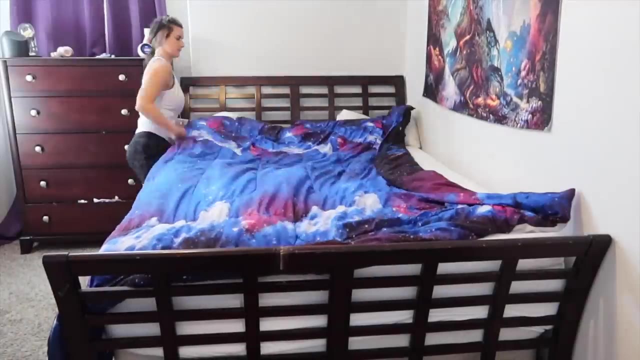 and dust. there is always a film of dust on her dresser, on her desk, So I thought today would be a great day to come in here and just take everything off of her desk and do a deep clean, because I haven't done that for her in quite some time. I've been making her do most of the dusting. 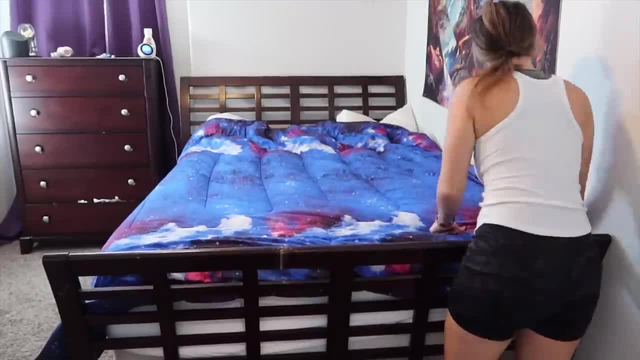 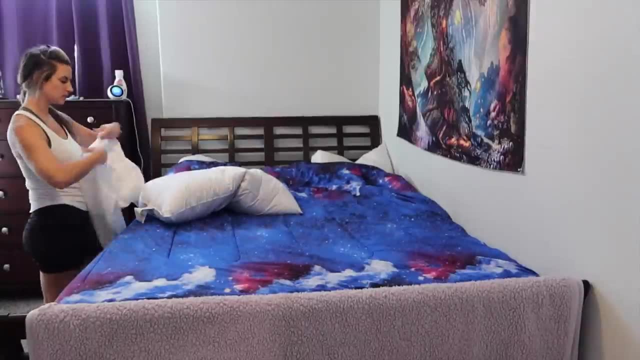 but I just noticed that it's really starting to cake on, not only on her but on her ceiling fan, but everywhere else. So we're going to do a nice deep clean in here. I almost took down her curtains, but I actually recently washed her curtains and got them all cleaned up, because 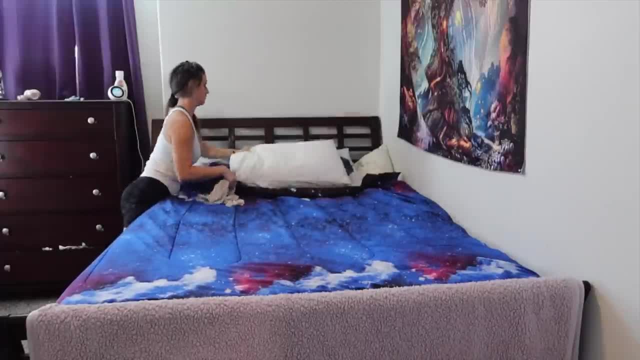 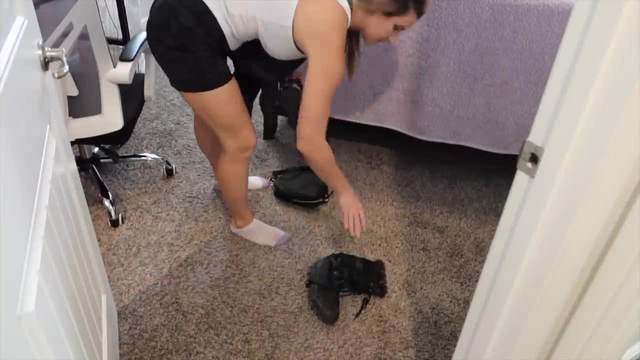 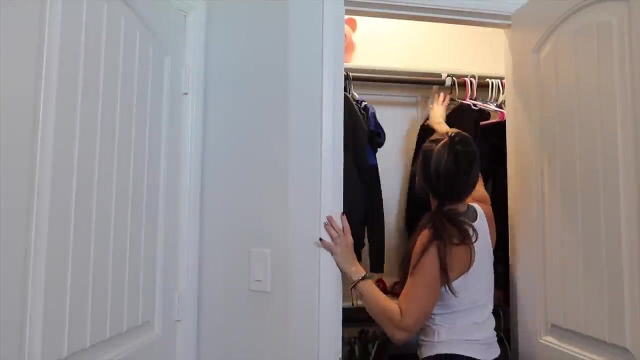 I had to take the um. I had, like, the sticker that would block out the sun on the upper half of her window. So whenever I took that sticker off, I like took down her curtains and wash them and everything. So I figured her curtains weren't too bad this day, but we're going to get everything. 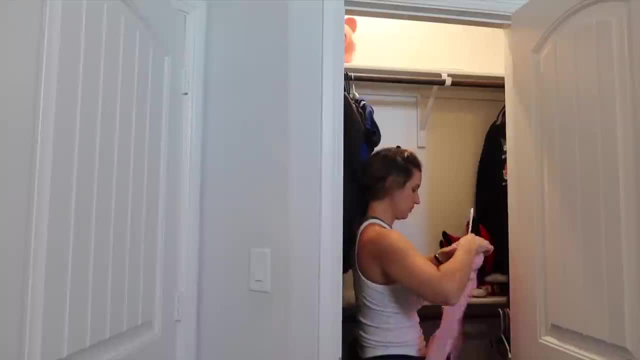 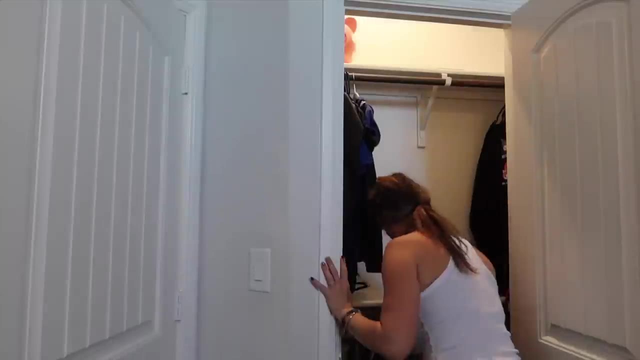 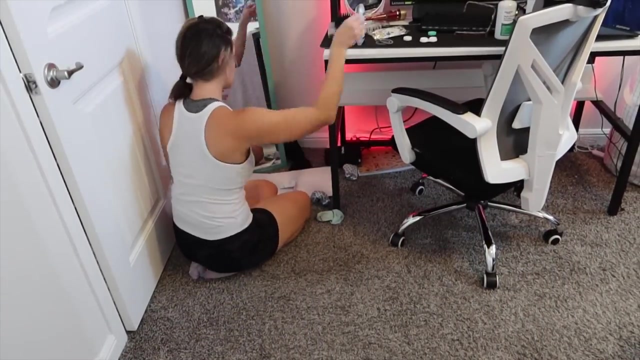 else in here dust free. But if y'all have not washed your curtains ever before, I highly recommend doing it. I just recently started doing this and I can feel the difference in the room after I pull them out and hang them back up again. It just feels lighter and cleaner And it's great because 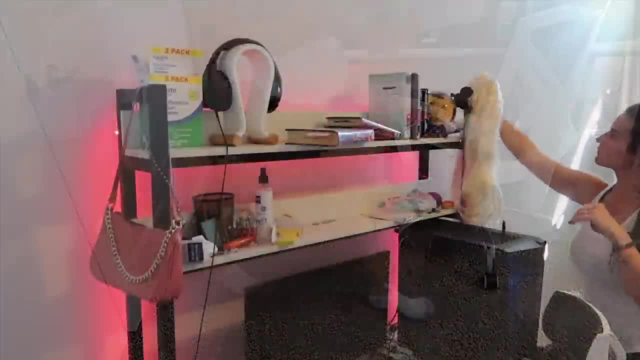 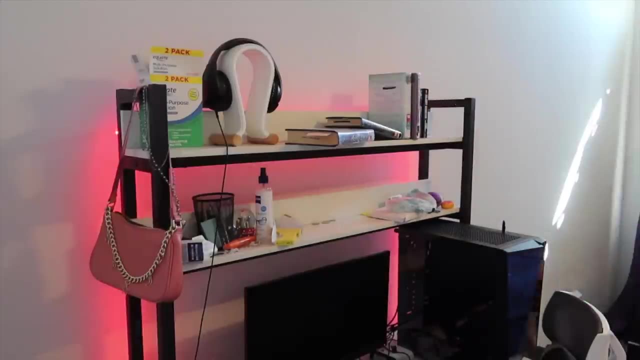 you don't even have to put them in the dryer, because you know sometimes you worry about shrinking. You can just hang them directly back on the curtain rod And then you can just hang them and let them hang dry, And it also makes your house smell really good Like laundry. 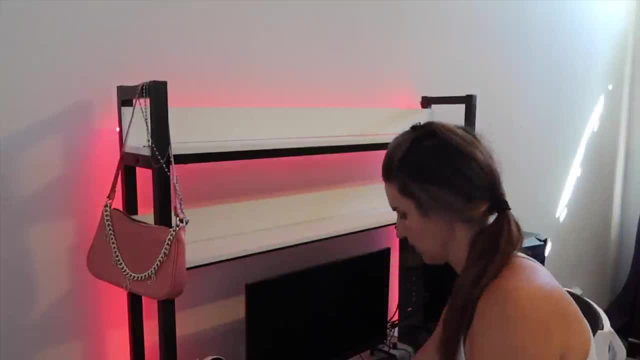 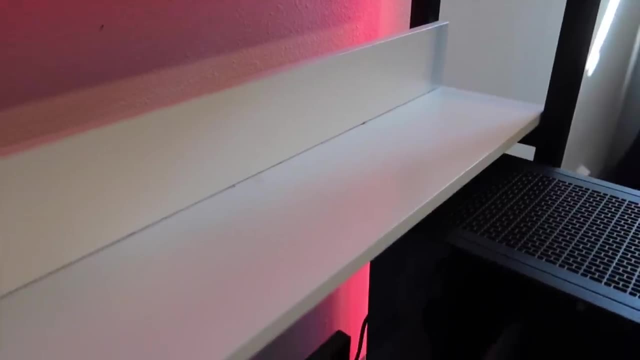 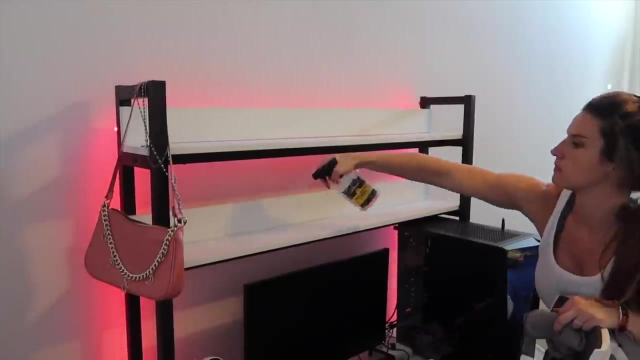 So, as you can see, I'm just going ahead and taking everything off of her desk, That way I can wipe it down. And then I wanted to make sure I vacuumed really good all near her computer and just got all the dust up. I think because she does have so many electronics in here. that might be. 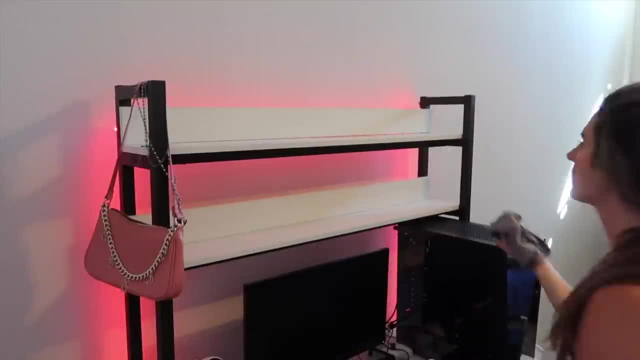 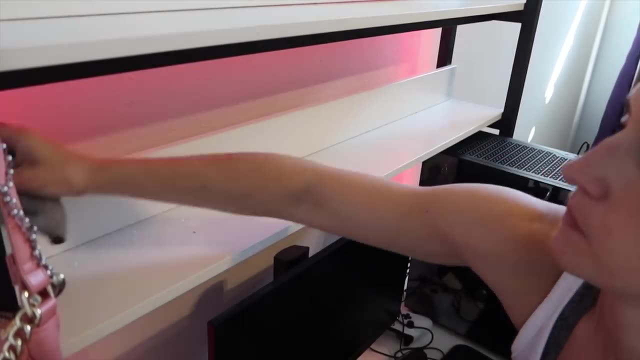 contributing to all of the dust, but whatever it is, this room is so dusty. I also have a little air purifier in here for the air purifier, So I'm going to go ahead and put that in there, Just to kind of help. but it recently fell apart and I just haven't came in here to put it back. 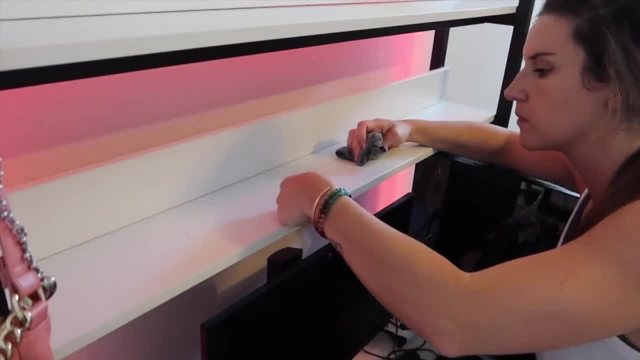 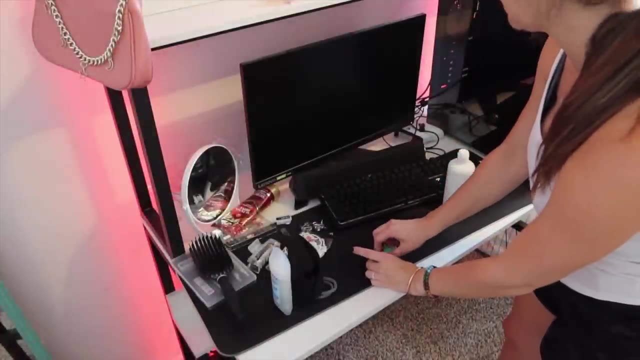 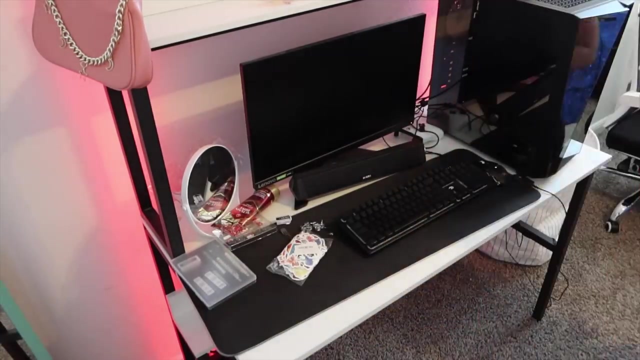 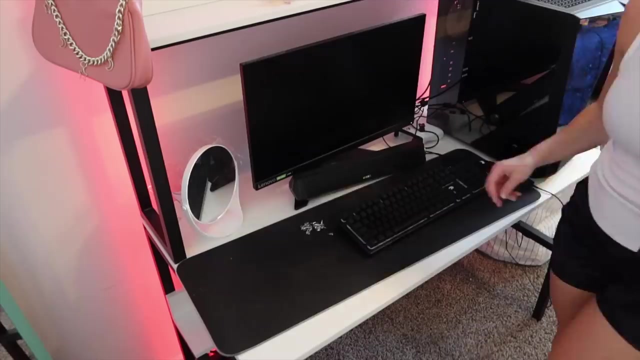 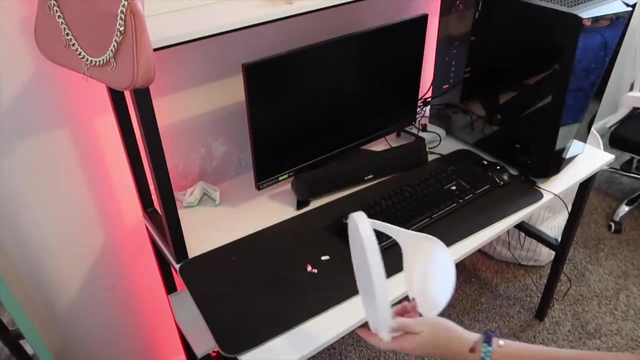 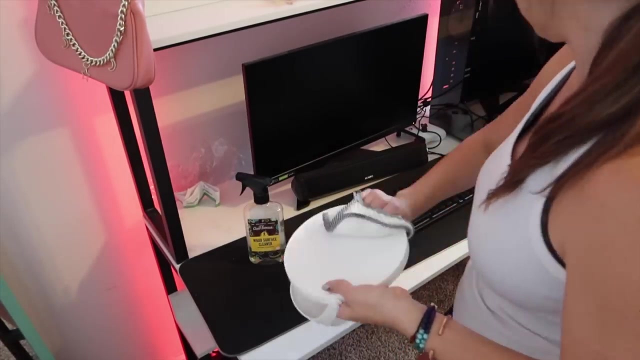 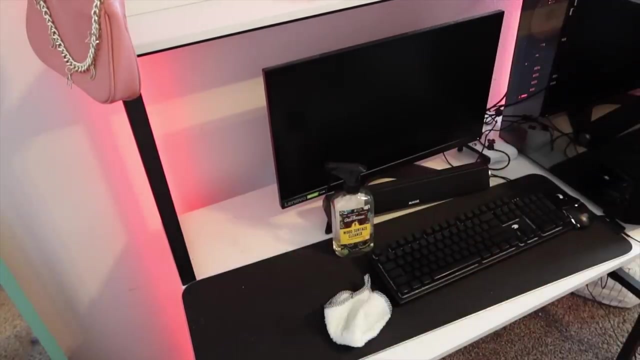 together again and clean it. So we're also going to be doing that today and getting it back up and running for her. So I wanted to share a little quote with you guys that I've been thinking about recently, just from some of the comments that I get on my channel about people saying like: 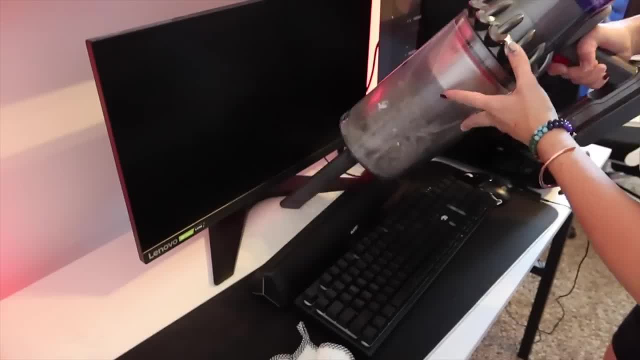 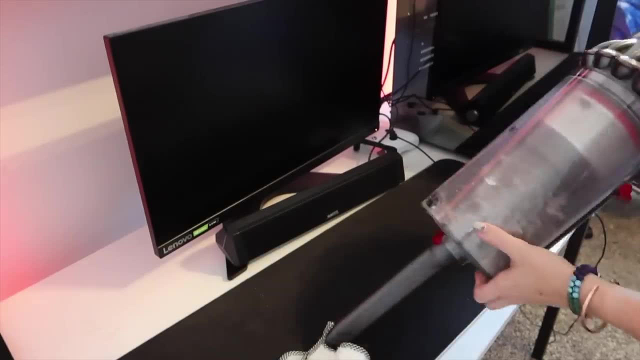 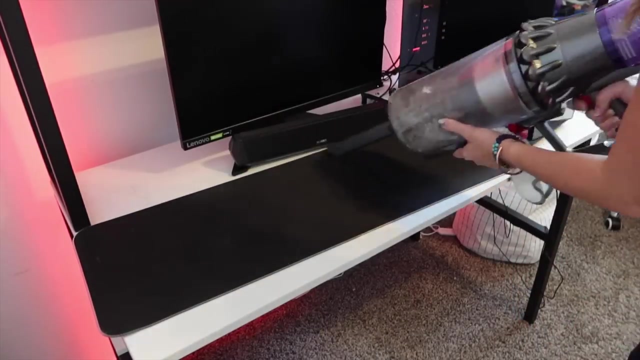 I wish I had your energy, or I wish I could get as much done as you, And I just want to encourage you that you have the energy inside of you. You can get everything done that you want to, and you can do whatever you want. whatever you put your mind to, I promise you can do. 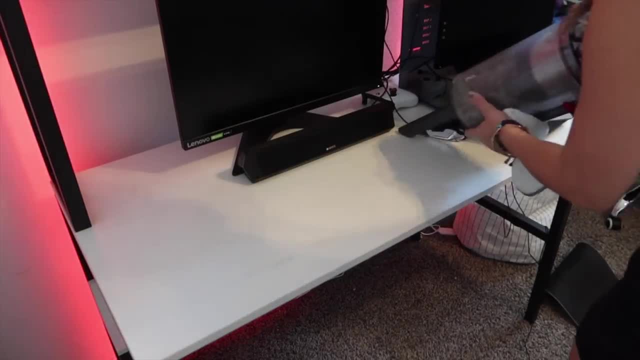 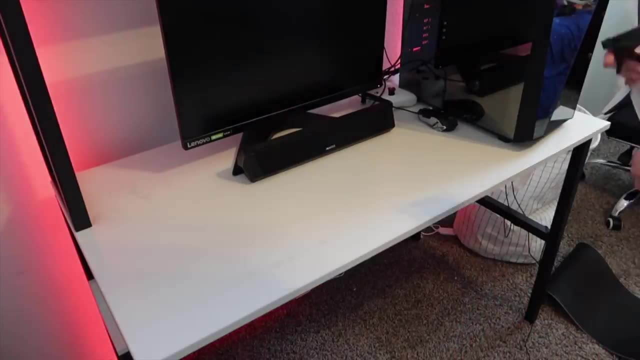 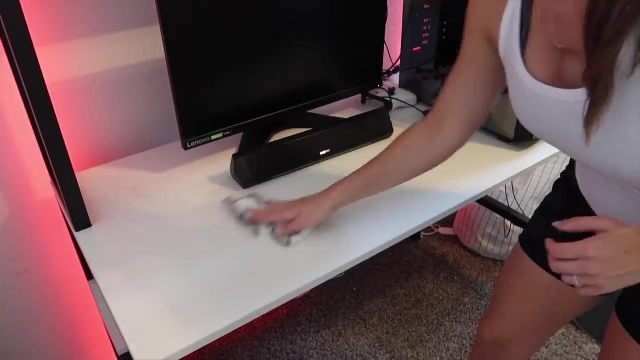 And one of the quotes that I love is from Sir Isaac Newton, and it's his first law of motion, And it's that a body at motion stays in motion and a body at rest stays at rest. And you guys, this could not be more true If I have a day where I just wake up and I'm feeling: 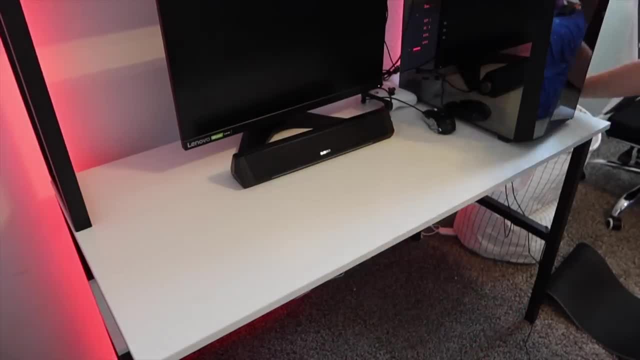 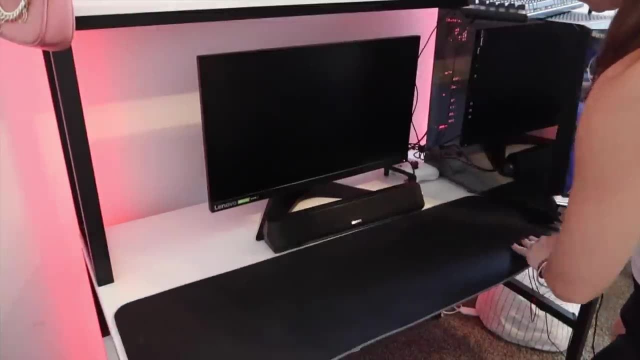 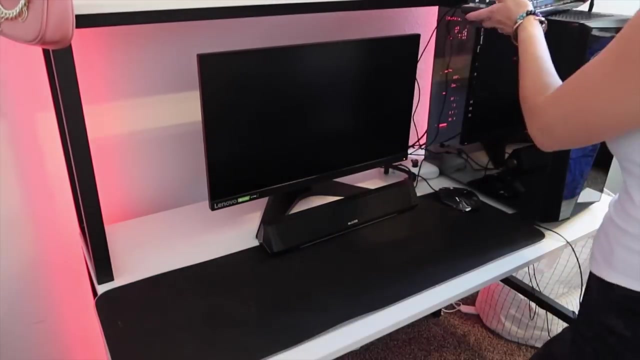 run down and I just start my morning off by lounging on the couch watching some TV, scrolling on social media. before I know it, over half of the day is gone And I've done nothing. I've not been productive, I've sat on my butt and not accomplished anything that I wanted to. 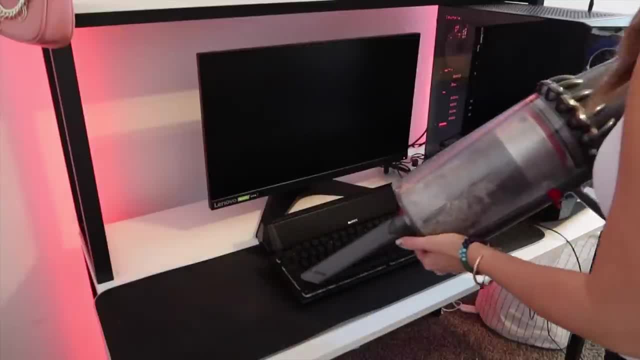 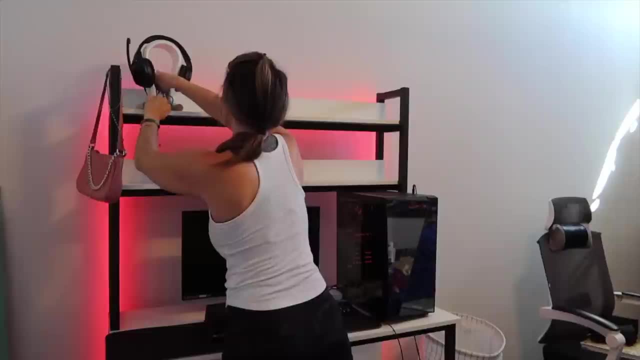 versus. if I wake up and I'm like you know what, I'm really not feeling it today, I tell myself, let's just go get my steps in, I'm just going to go on the treadmill, nothing crazy, but I'm just going to go get my body moving. And nine times. 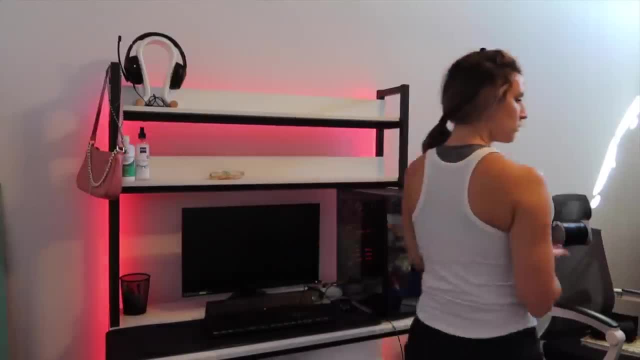 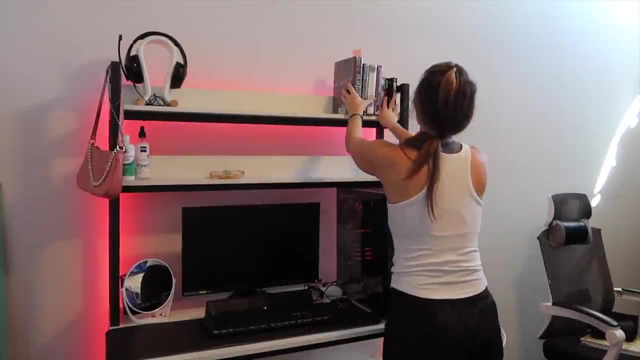 out of 10, by me just taking that step to move. not even do anything crazy, just simply walk. It gives me the energy to start the next thing and the next thing. So I promise you, you guys, you have it in you. 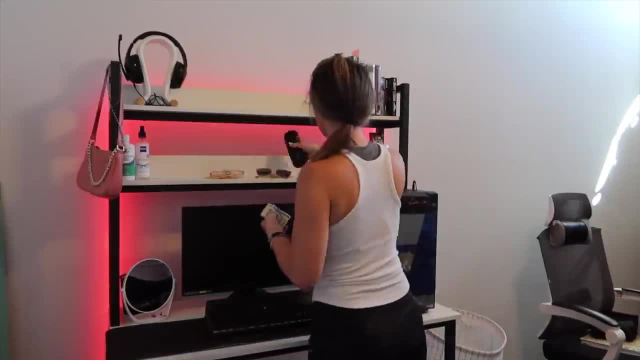 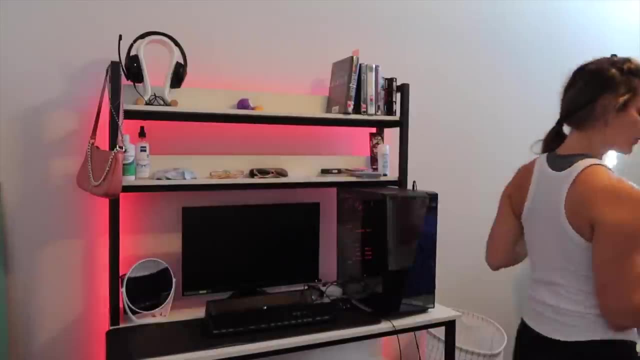 If you've been struggling with just getting up and getting moving, take that first step: just get up and start moving. It doesn't even have to be anything crazy, And that goes with not only cleaning. If you need to get motivated with cleaning just by getting up, starting on. 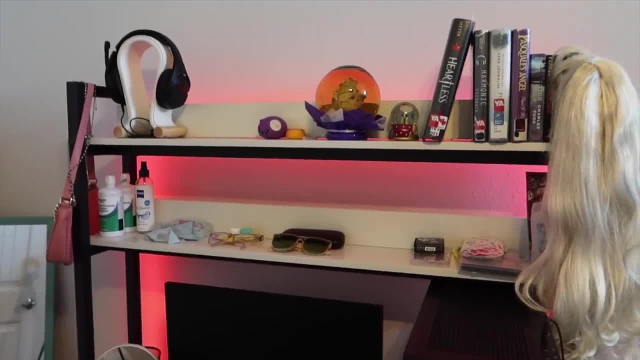 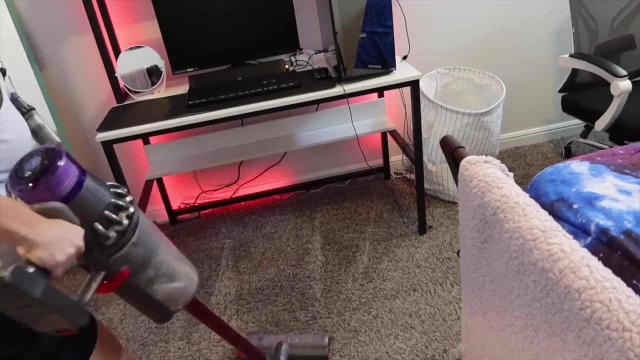 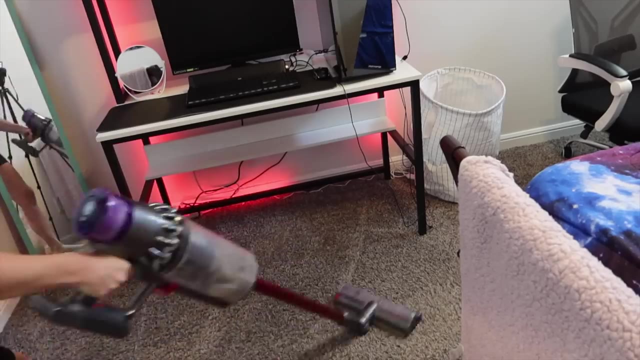 one small task. If it's just loading the dishwasher or unloading the dishwasher, usually that momentum will get you moving and, you know, get you wanting to clean the next thing. But that also goes for like if you've been struggling on wanting to get in shape or start a fitness journey, start small. 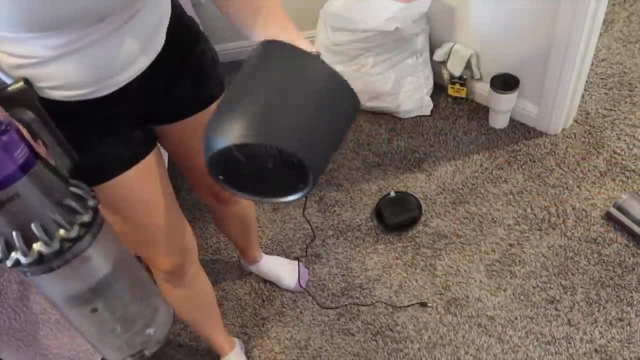 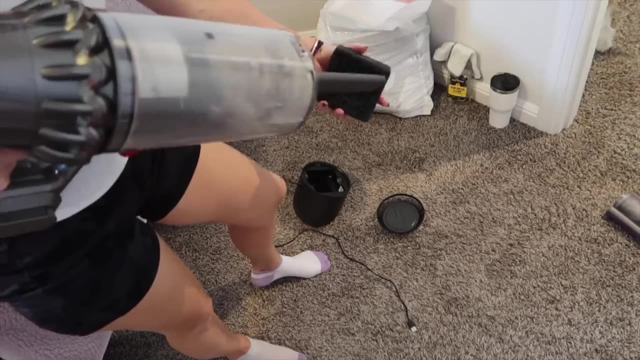 And I promise those little baby steps are going to add up. just by starting to get your steps in and doing that consistently, You're going to find that you have more energy and you're more encouraged and motivated to start doing more, being more active. 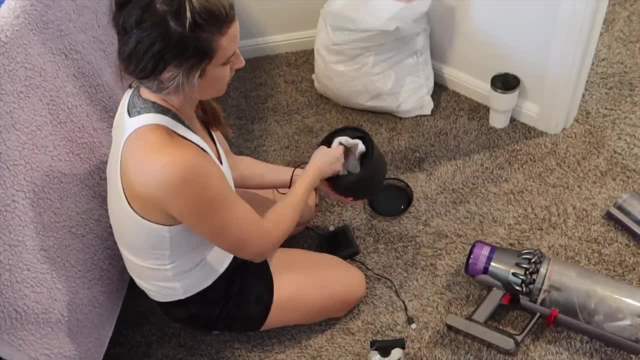 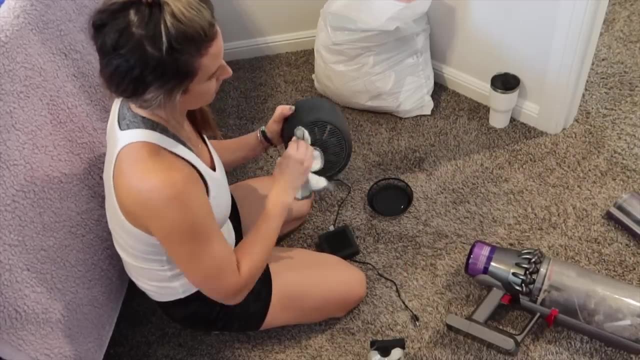 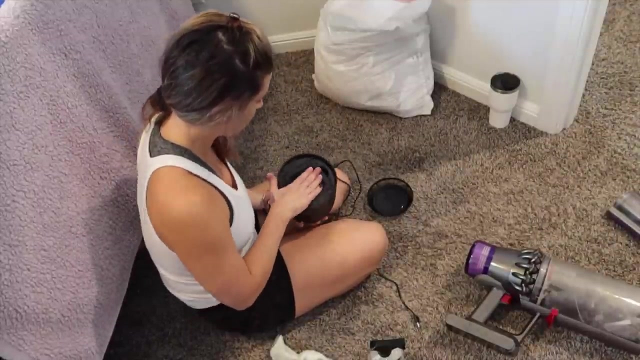 So I just thought I would leave you guys with those words of encouragement, because I've just been thinking about it a lot. I'm going to start doing more being more active. I'm going to start doing more being more active. I'm going to start doing more being more active. 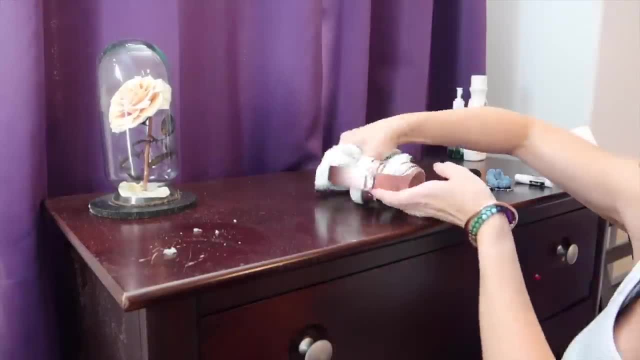 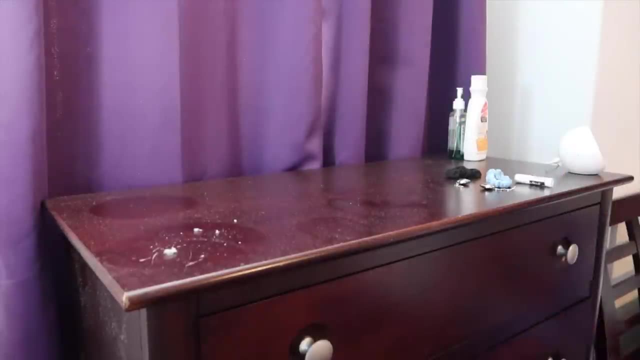 My goodness y'all. look at all the dust up here. So we're going to go ahead, get all of this dust free, wipe it down, And then, while I was at it, I needed to clean it up a little bit. So I'm going to go ahead and start doing more, being more active. 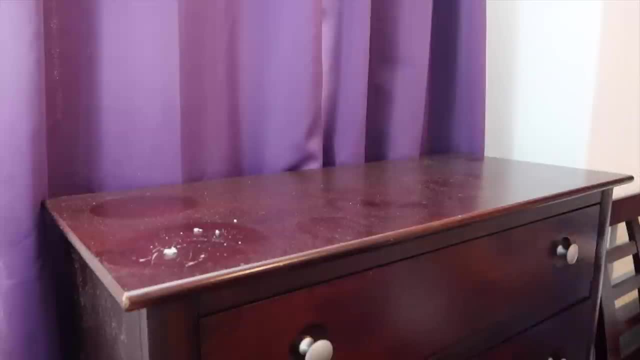 Aubrey's lower drawer. Once again it was off of track and I needed to pull it out. She had a bunch of clothes that fell behind it, So I'm going to fix that for her. And then when she got home from school, I had her declutter that bottom drawer. She had so many things in there that 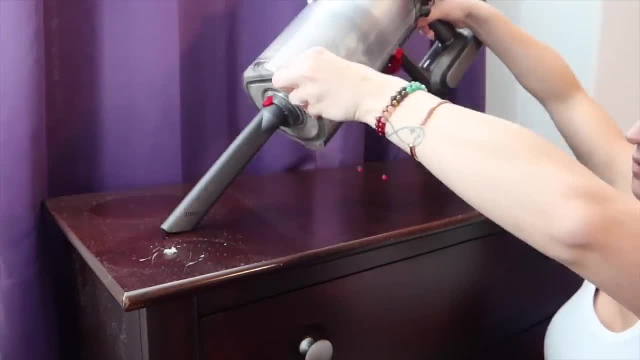 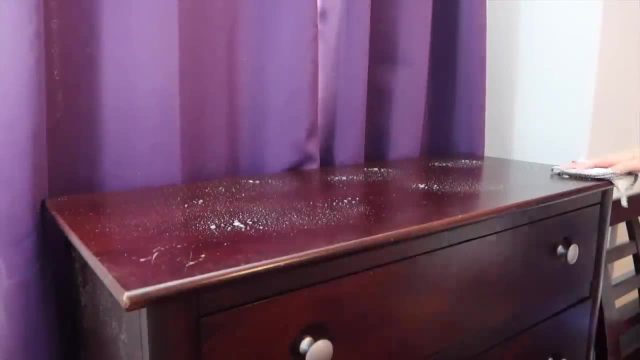 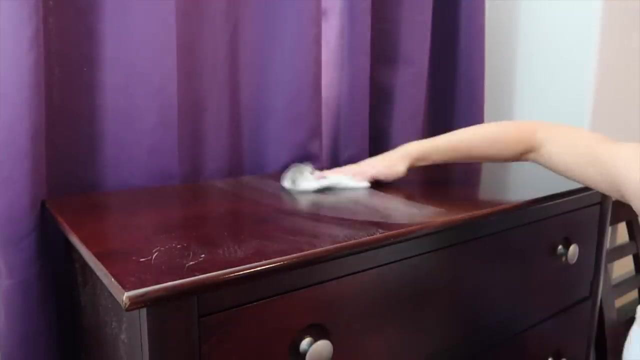 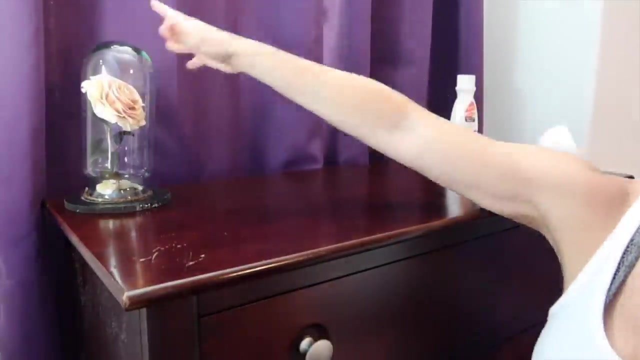 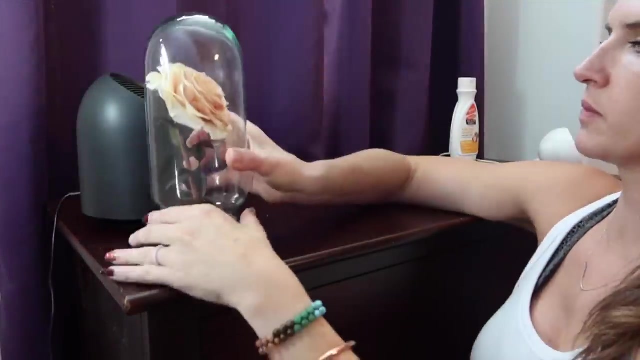 she no longer uses. So she finally went through that So her drawer can close properly, Say point month somewhere, in the sense that like the her drawer, I had bought this stupid spray. I hate추 n't suspect if she's spray too much. 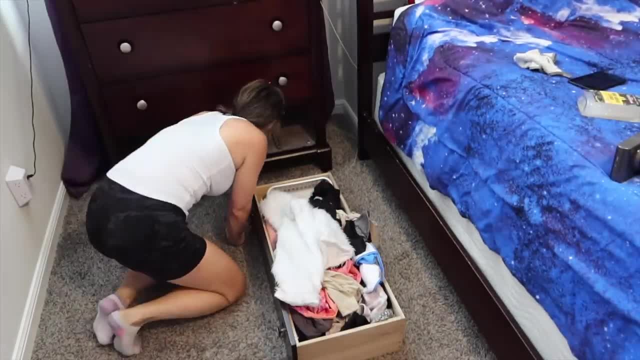 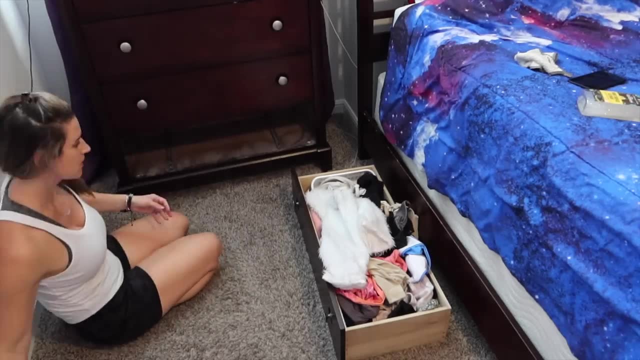 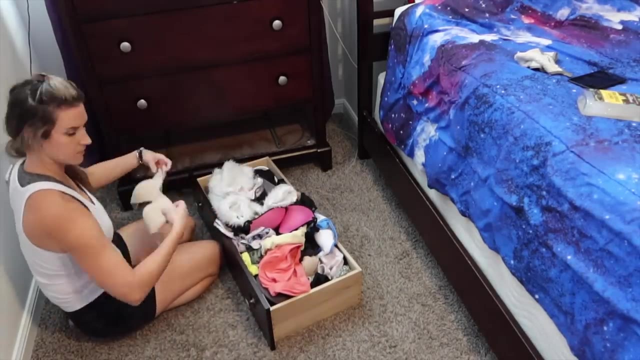 Oh, it's hot, C'mon on your feet. Oh, she's a little hot, as every other day. Come on, C'mon, Come on, Come on. i cannot believe how long we've had this dresser. you guys, this is the first furniture that we ever. 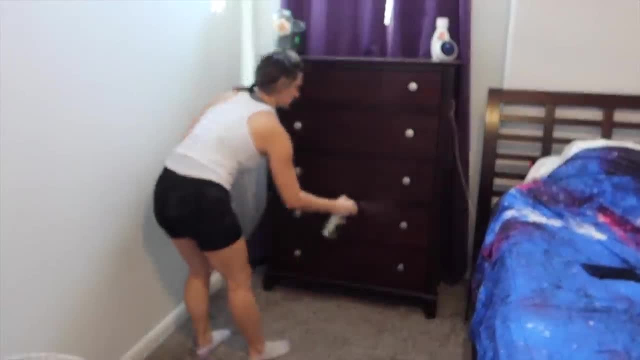 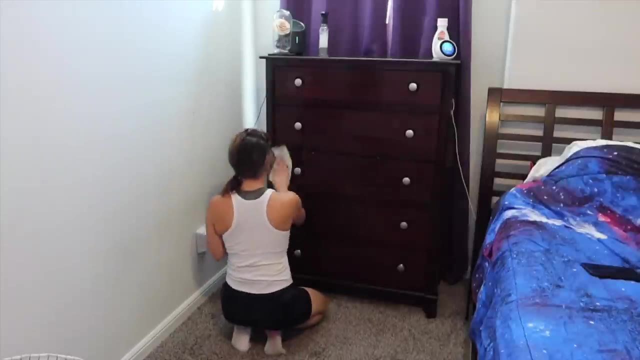 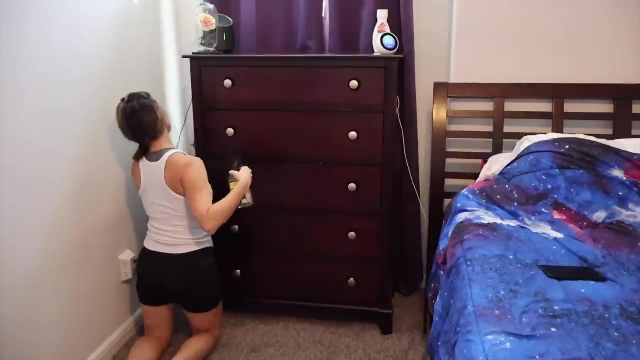 purchased this dresser and that bed frame. me and my husband bought that when we first moved in together over 15 years ago, so this has held up for quite some time. the end of the bed is a little cracked. the frame has been cracked for quite some time, so I think probably in the near future we 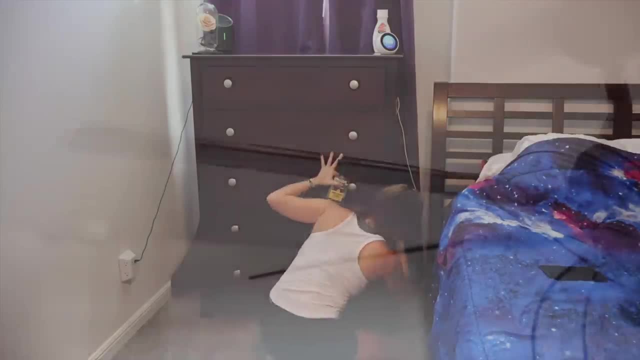 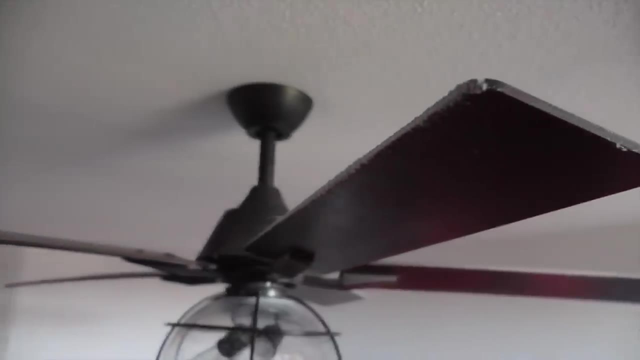 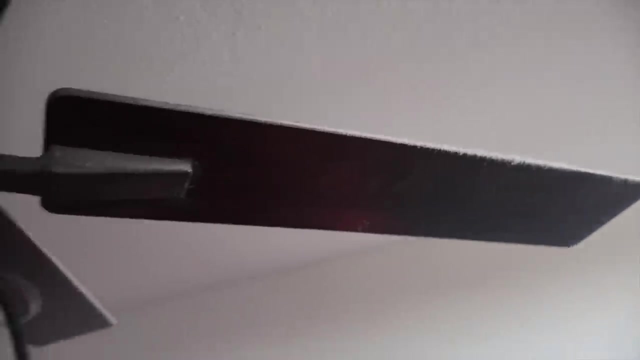 will be buying Aubrey a new bed frame and I've actually been thinking about maybe painting the dresser and giving it a good like revamp, a refresh, because the dresser is still in perfect condition. just the wood on the side of it is a little scratched up from when we used to have a little 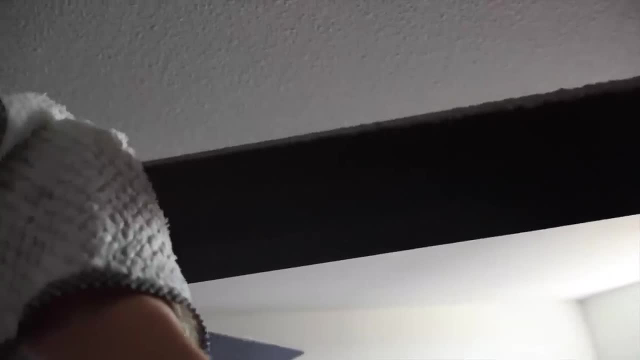 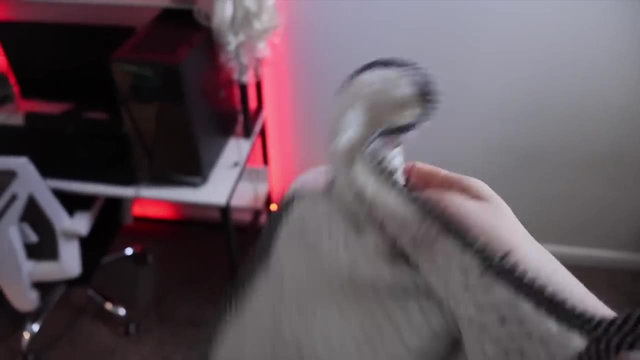 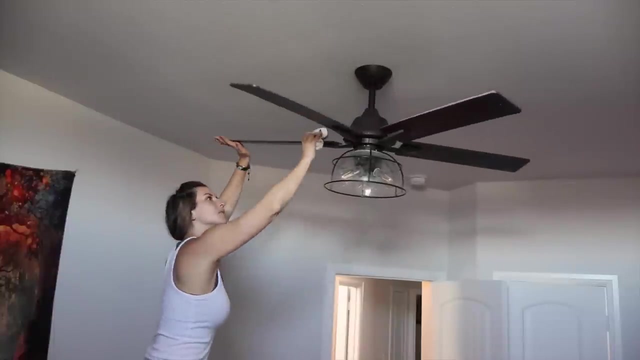 kitten and it scratched up the dresser. so I've been thinking about maybe redoing it whenever we finally decide on like a new bed frame, then I could do a little DIY on her dresser to match whatever color she might end up picking. but I've been thinking about 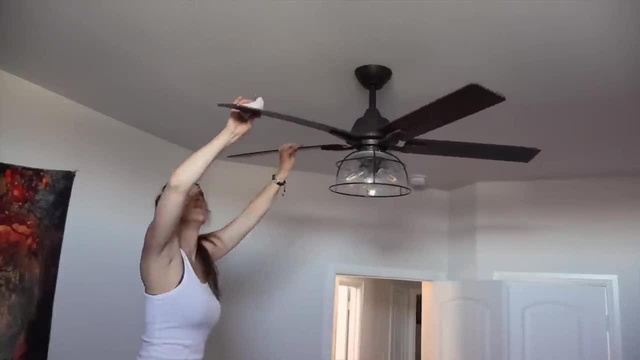 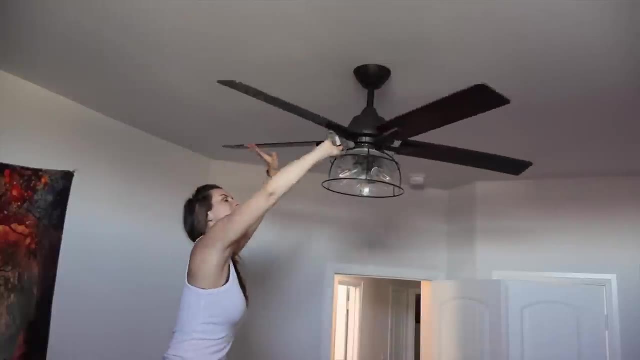 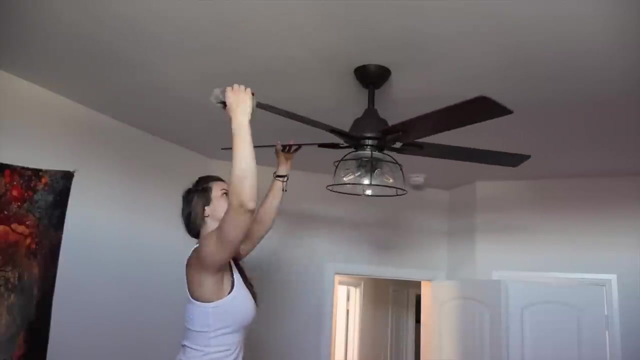 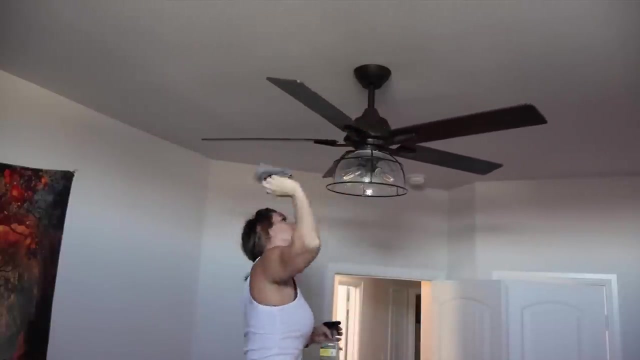 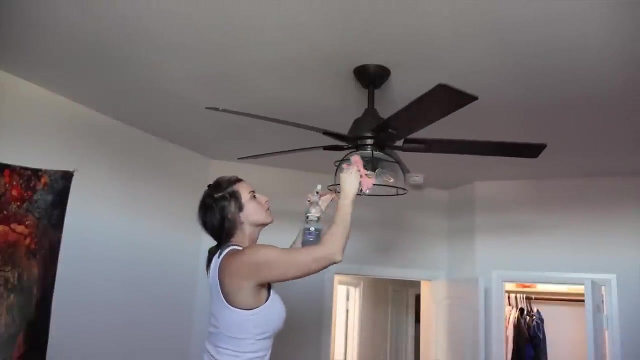 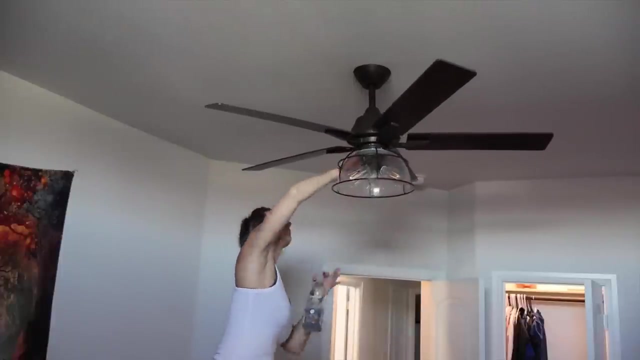 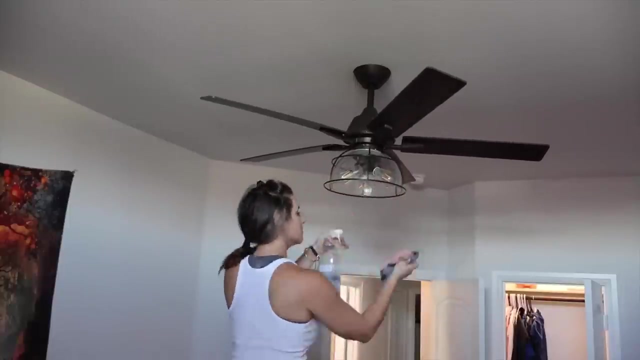 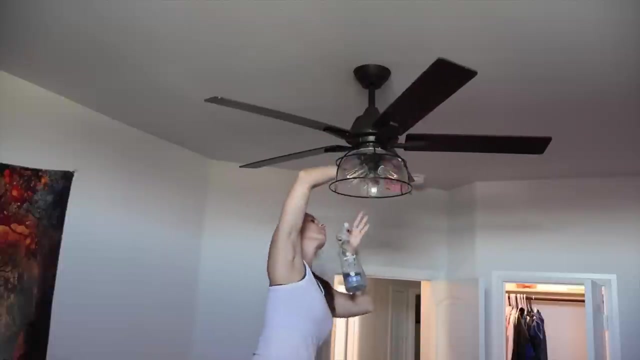 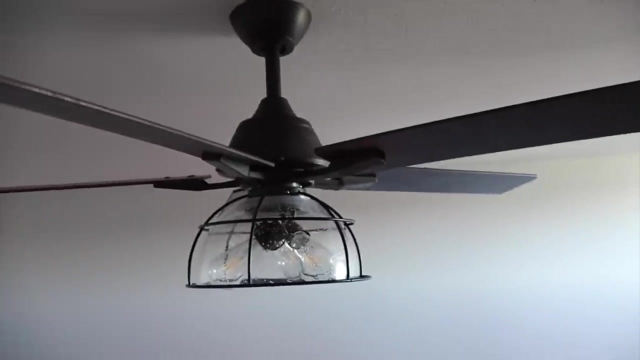 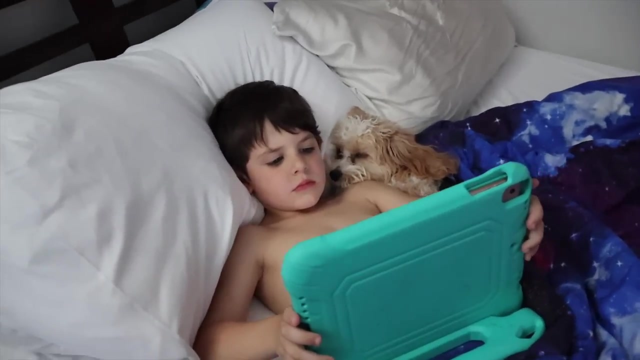 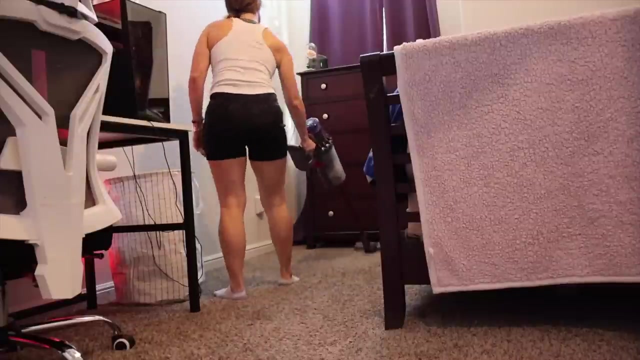 that I've been having the itch to kind of do some DIY projects recently, so maybe that will be in the near future on my channel. you- this was so sweet, i had to put this in the video. athan and stella are two little peas in a pod. he is always carrying her around the house. 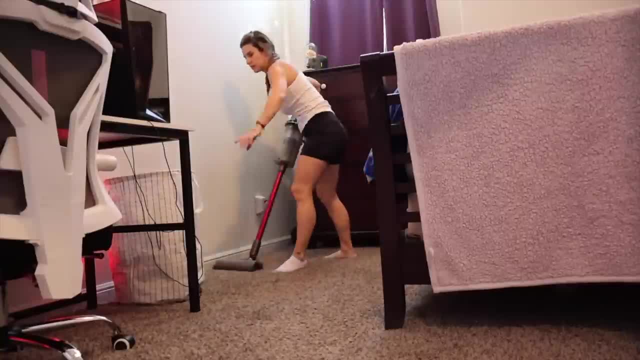 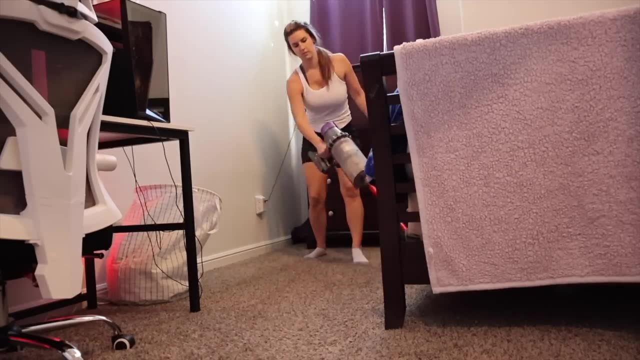 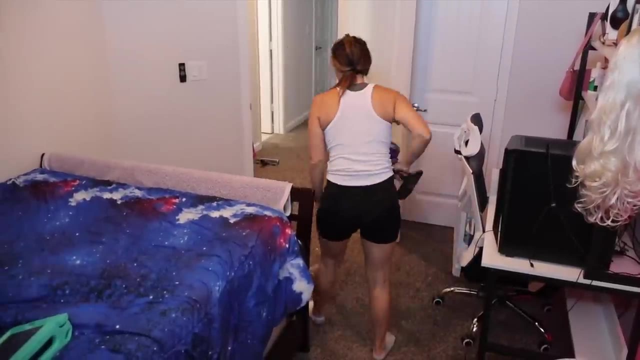 she is such a sweet dog, you guys like, honestly, we won the jackpot with her. she is so sweet and just lets athan do whatever he wants to her. i'm oftentimes telling athan: like remember, she's not a stuffed animal. like you have to be very gentle, but he does so good with her. they are. 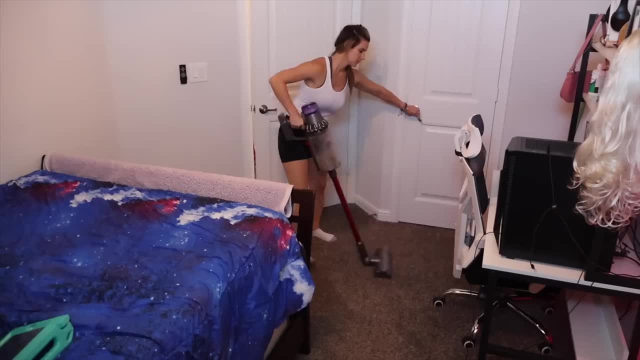 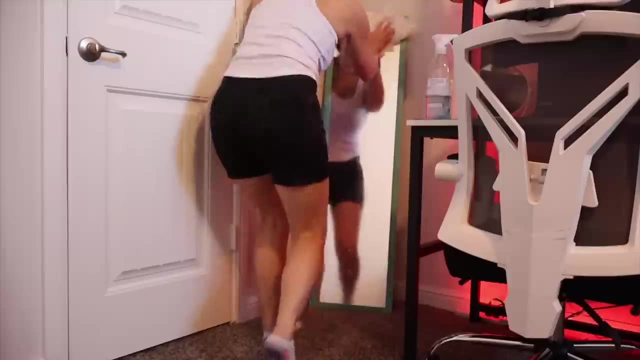 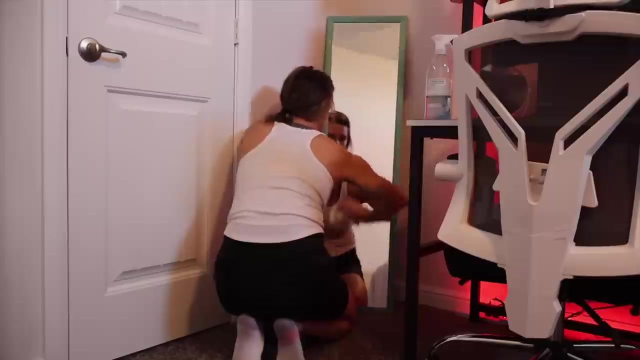 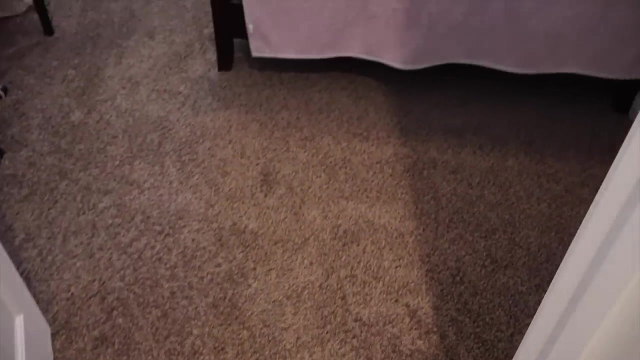 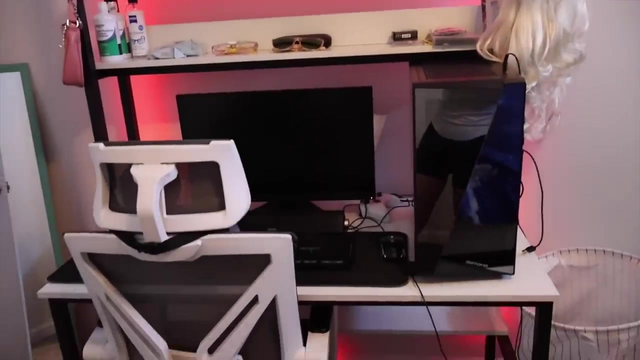 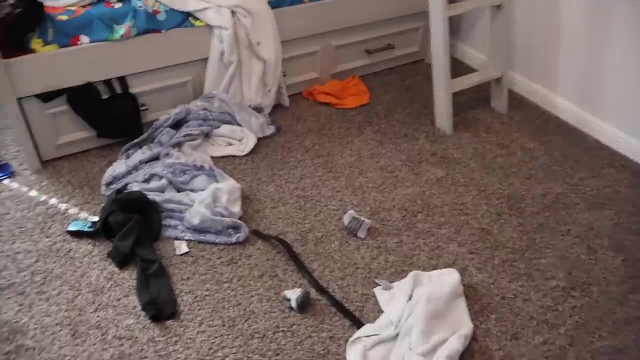 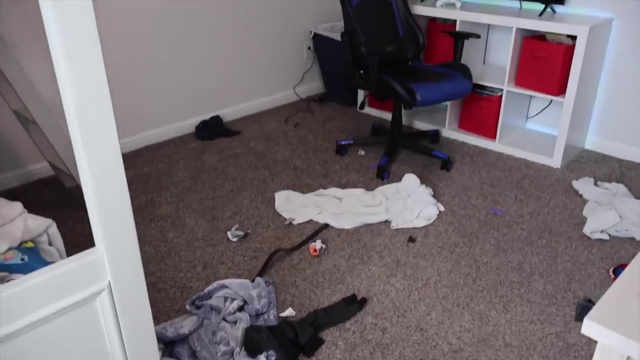 so sweet together and i'm really excited to just watch them grow up together. the last and final space that needed to be tackled upstairs is my boys shared bedroom, and if you guys watched my previous video, you know that i recently did a makeover in here. just a. 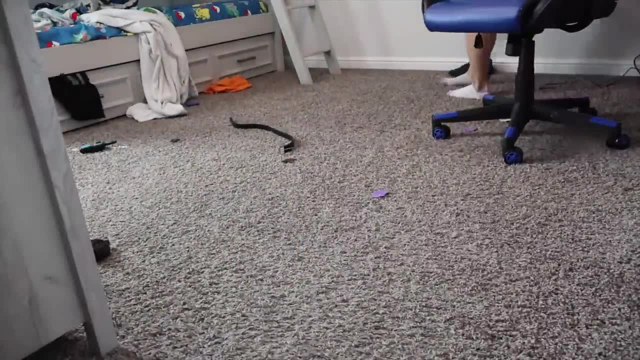 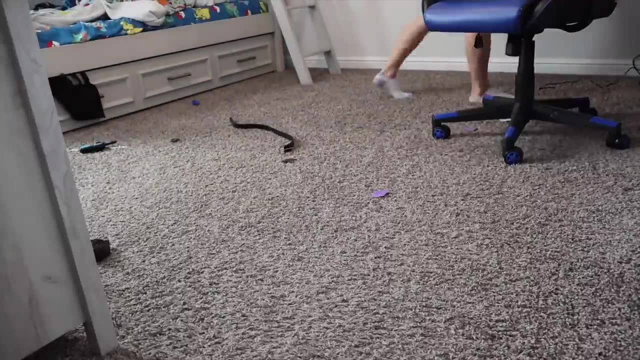 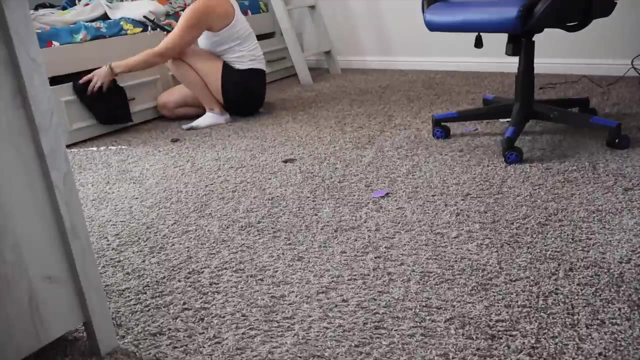 little revamp. i got their dresser, so it really wasn't terribly dirty in here, but i did want to do some deep cleaning. i needed to pull their tv stand out and clean behind that, because whenever i was wiping it down i bent down and realized how dusty it was back there. so we're 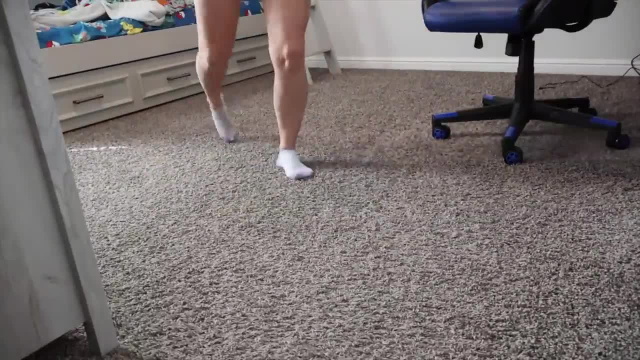 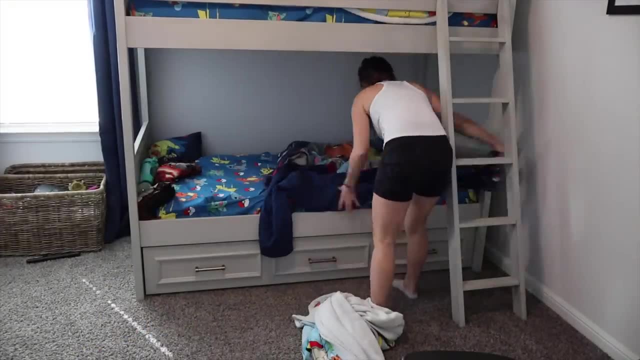 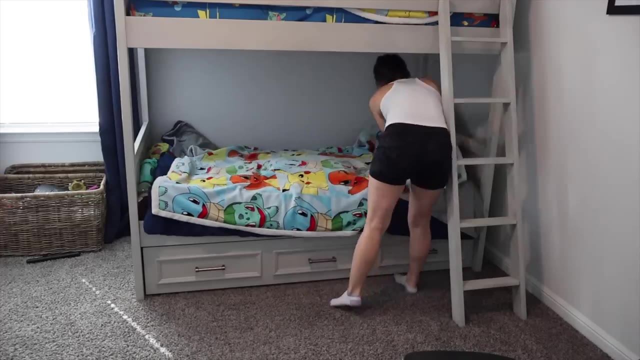 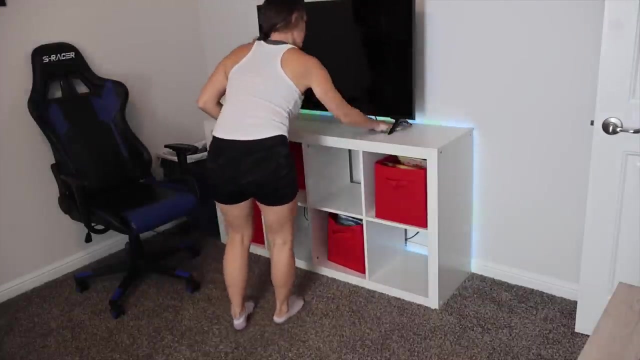 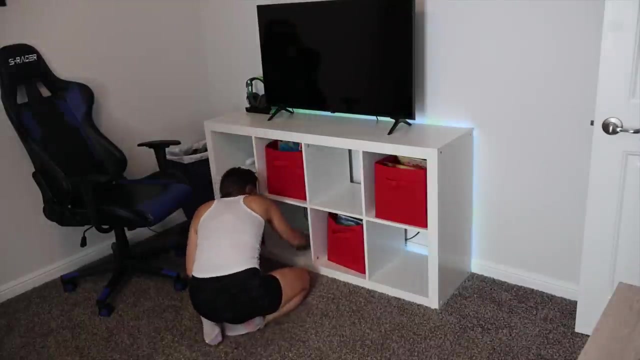 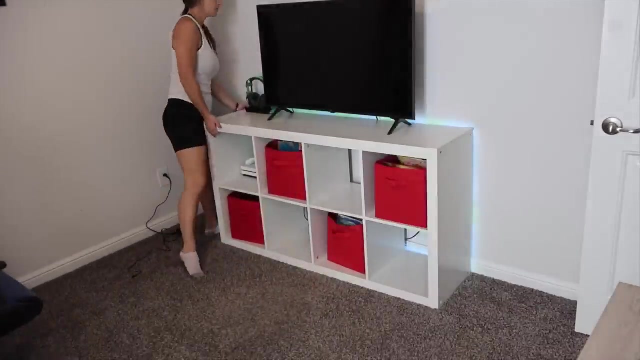 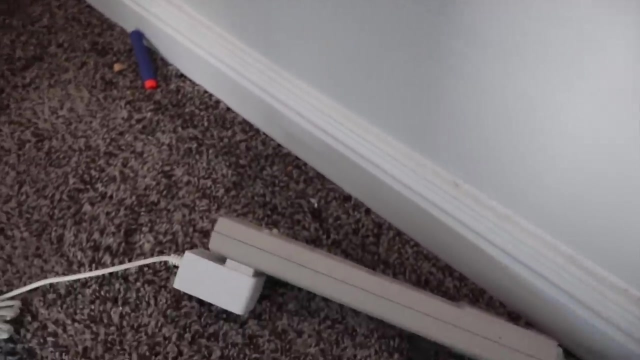 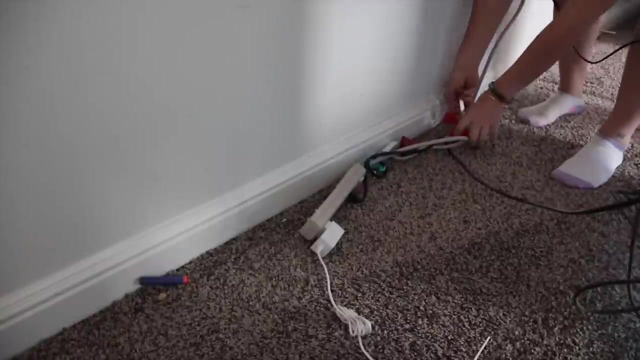 gonna move the tv, stand clean back there and also wipe down their fan and just get it looking tidier in here and dust free. so i don't think the camera does it justice with how much dust was back here, you guys. it was so большое. 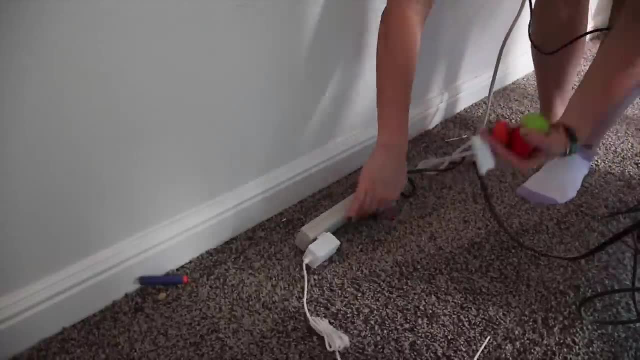 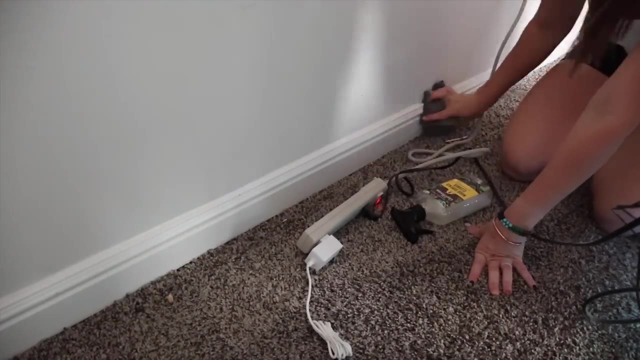 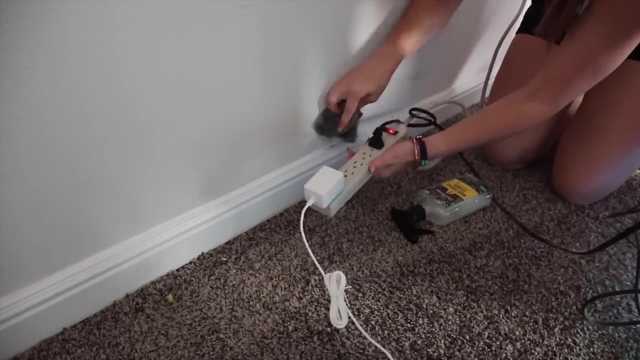 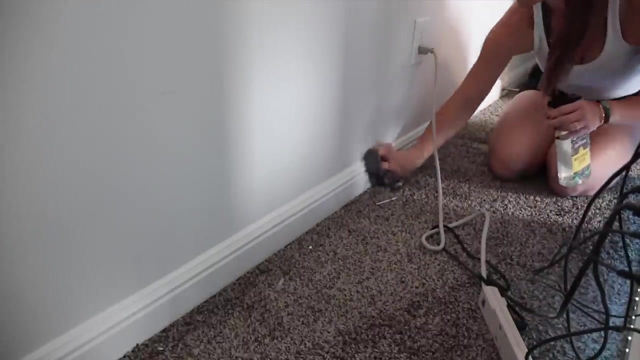 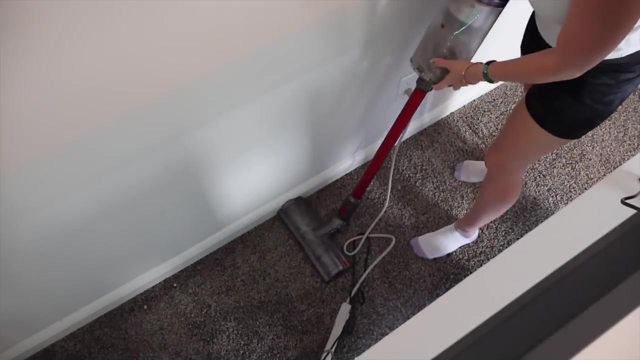 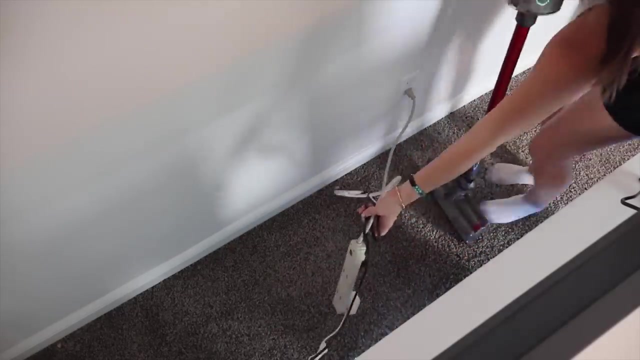 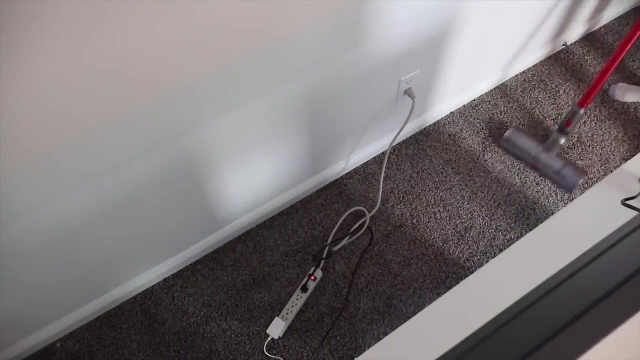 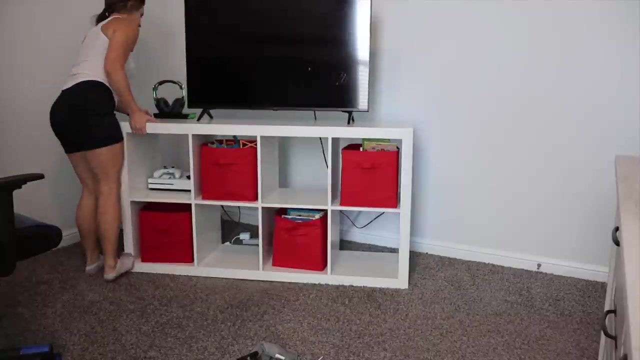 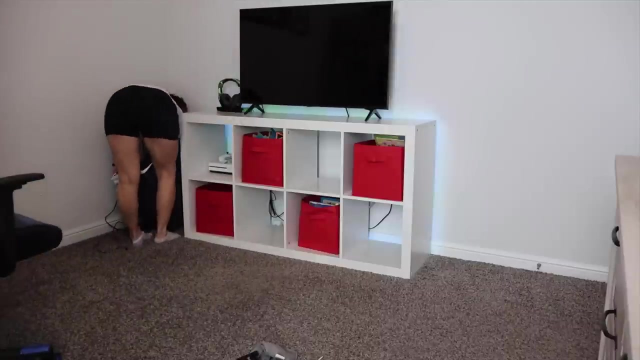 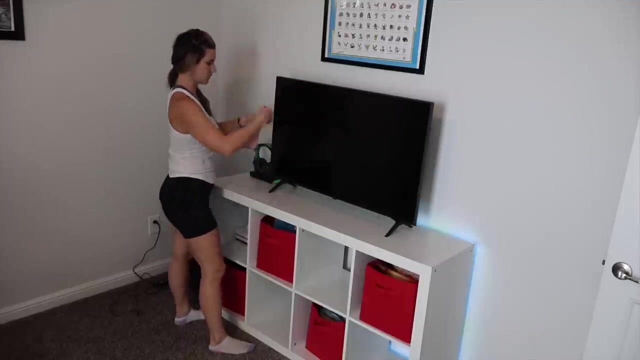 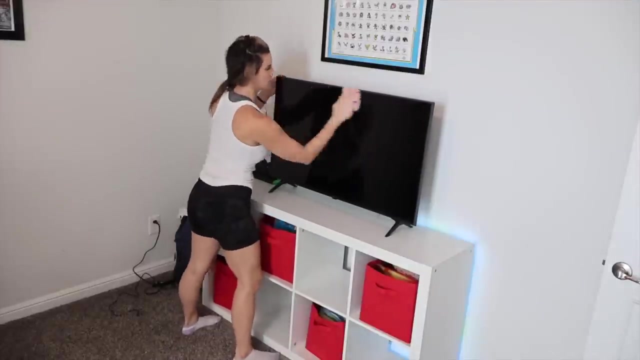 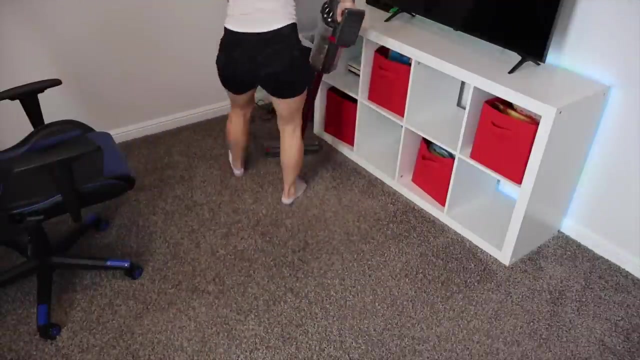 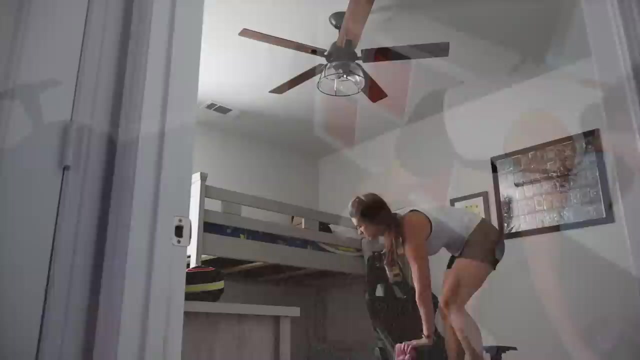 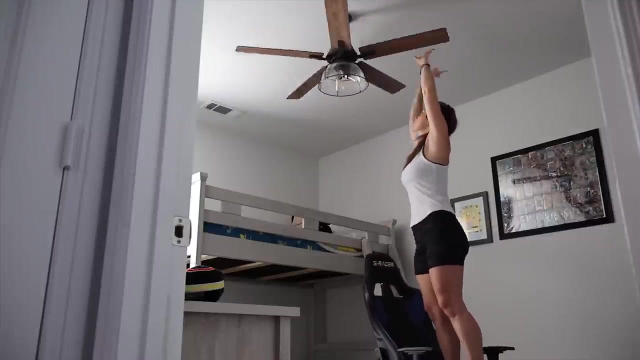 dusty, So I'm glad I finally moved this away from the wall and got it all cleaned up. Thank you, Thank you. I was getting a little nervous standing on this chair, Trying to keep my balance and wiping the fan was no easy task, but I got it done. I got their fan. 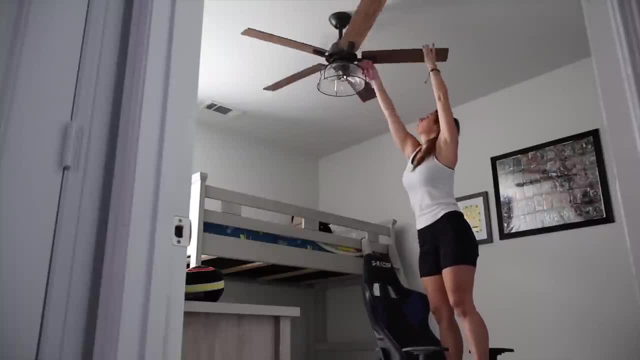 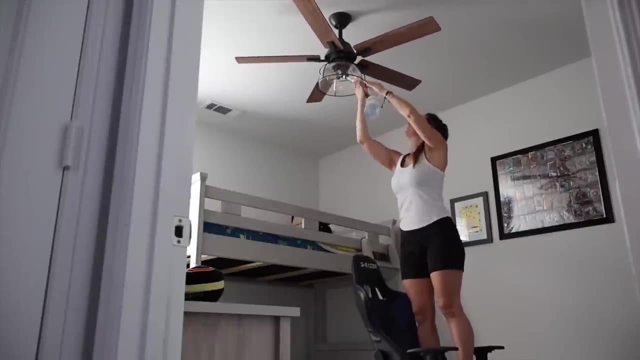 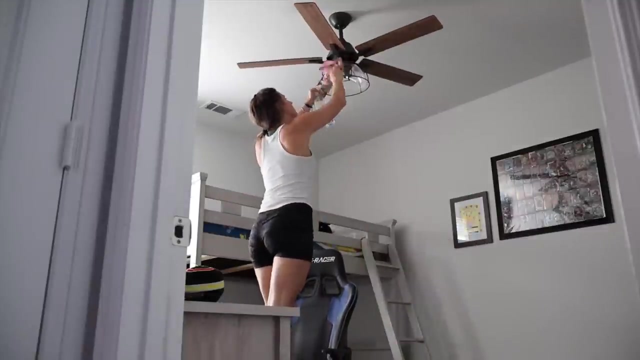 cleaned up. It definitely wasn't as bad as the girls fan, because I have cleaned theirs pretty recently, But I was like you know what. I'm just gonna do it today. That way I know I did all of the kids bedrooms at the same time, So when I notice one, I'll just clean all of them. the next: